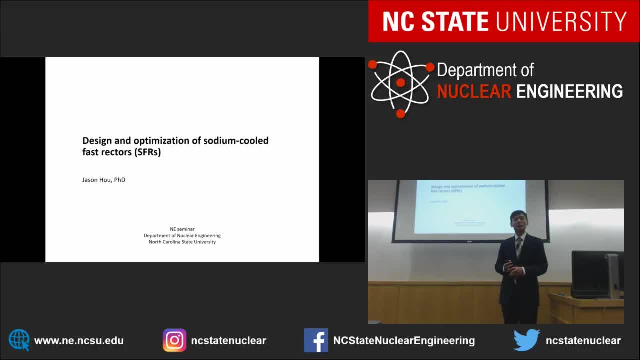 It's design and optimization of the sodium-cooled fast reactor. Sodium-cooled fast reactors. So, before I get started, I want to ask you a question, which is the following: Is the world's first nuclear reactor of any type to generate usable quantity of electricity? 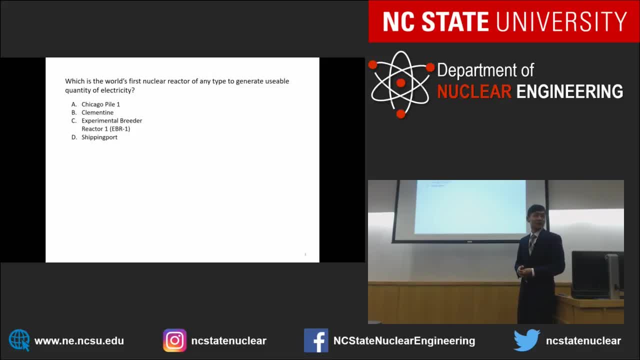 So I have four choices here. So you know, when I was in high school I was going to take the entrance exam of the university. I've always been told that if you don't answer, pick C, Because most likely it will be C. 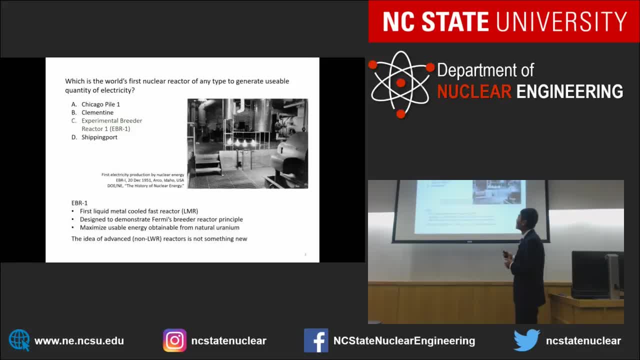 Yes, so it is actually the experimental reactor, breeder reactor EBR1.. In December 1951, the electricity coming out of this reactor was able to light up four light bulbs. That was the electricity coming that's usable Now. I see two things from here. 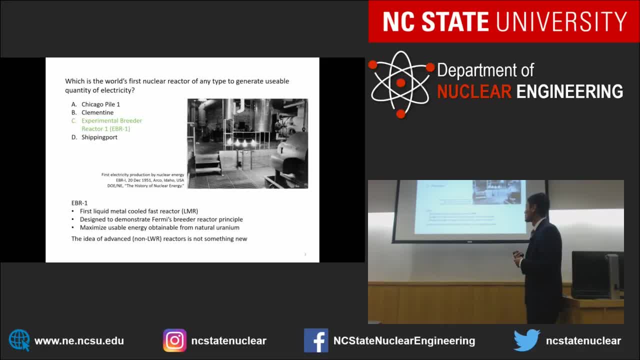 The first one is that the idea of the advanced non-light water reactor based advanced reactors is not something like really new. I mean, there has been the EBR1, which is a sodium-cooled fast reactor based technology since 1950s. 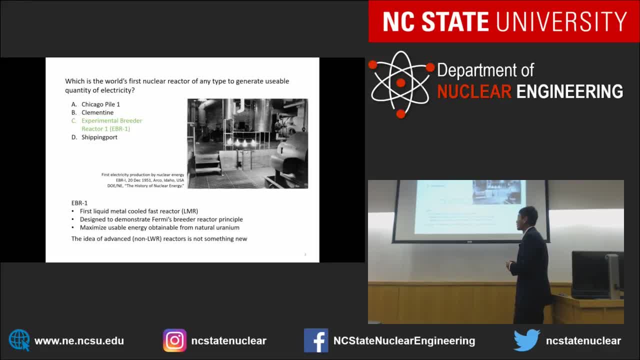 Okay. And the second way here is that if you define enough Or constraints or conditions, everything or everybody can be the world's first. Okay. So actually EBR is the first liquid metal cooled fast reactor, the breeder reactor, And it's designed to demonstrate the Fermi's breeder reactor principle where he says, okay, we can maximize the usable energy obtainable from the natural uranium. 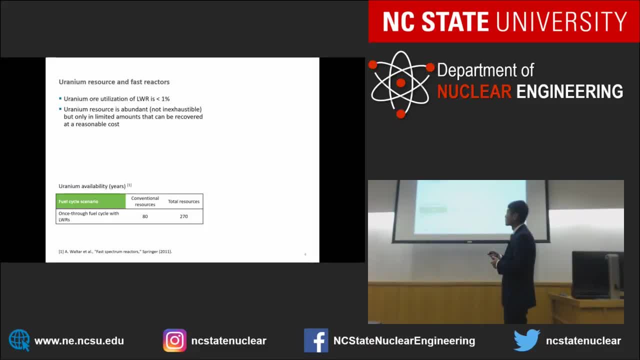 But why do we need that? I thought uranium resource is abundant, So we're told, But in fact only limited amount of this uranium can be recovered at a reasonable price. at a reasonable cost, Okay, And our current light water reactor systems can use less than 1% of the uranium that is available in the uranium ore that we dig out of the ground. So if we continue to use ones through light water reactors with open fuel cycle, then the current resource can sustain the nuclear industry for like 80 years or so. If we count all the uranium, regardless their grade, then we're talking about less than 300 years. 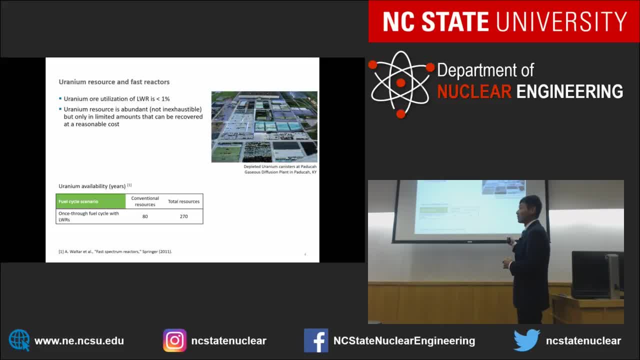 But at the same time we have a lot of tailings from the enrichment process we made for the light water reactor fuels. Okay, These are called depleted uranium, with enrichment about 0.2 to 0.3% of uranium-235. 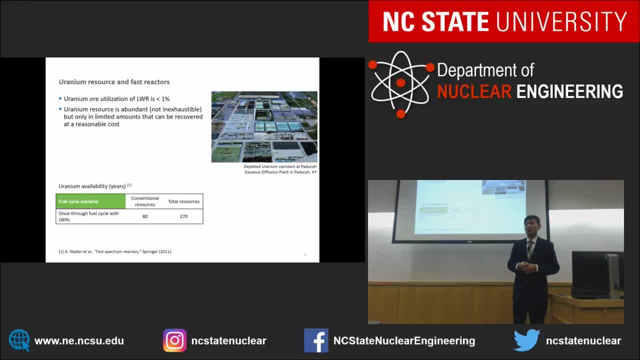 They're just sitting part of the enrichment plant And a lot of the energy I see in here are totally wasted. We realize that by using the fast breeder reactor, which has the conversion ratio larger than one, we can extend the uranium resource by a third. 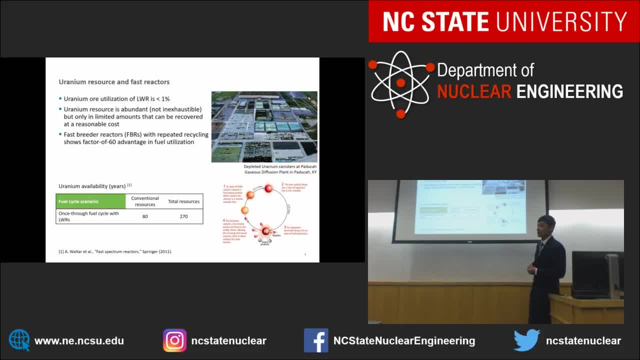 Okay, We can extend the resource by a factor of 60, comparing to light water reactors. The way we do it is that we heat uranium-238 with neutron And then we transmute the plutonium-239.. Okay, After a couple of decays, then we get plutonium-239. 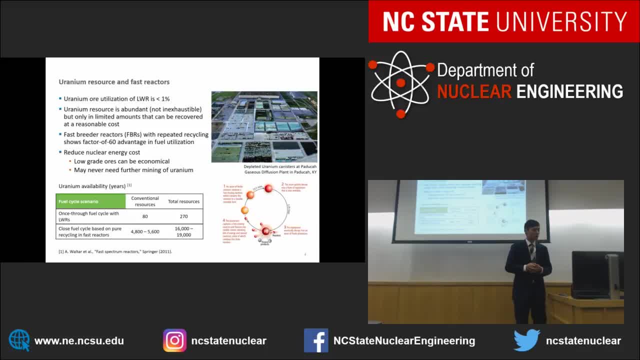 Now, if we can do this, we'll be able to extend our resource available to us to about 5,000 years. Okay, But if we can use all this uranium-238 in this depleted uranium, That means that we can reduce the nuclear energy cost, mainly coming from the nuclear fuel. Because low-grade ores can be economical again And we may never need to mine more uranium. Okay, We can just use whatever is already available. Another advantage of using fast reactor is that we can use uranium-239.. Another advantage of using fast reactor is that we can use it to minimize the waste. 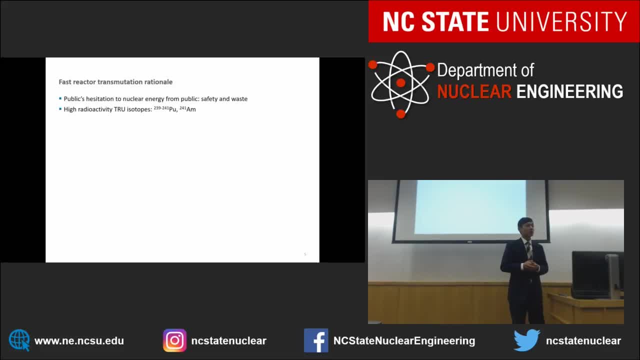 Okay, I hope you all agree with me that the public hesitation to nuclear energy mainly comes from two sides. One is the safety, The other is the waste. Now, talking about the waste, the really nasty ones are these long-lived transuranics. 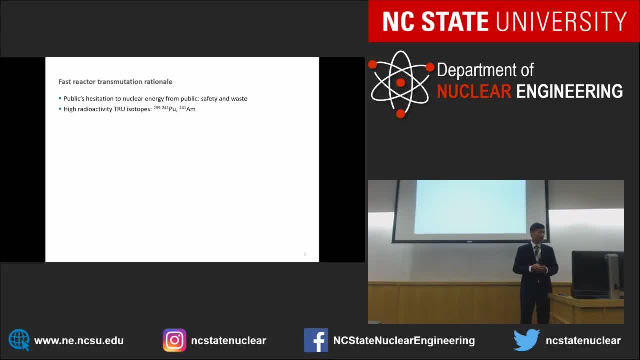 Okay, Plutonium or americium, for example, And fast system. This is the very resistant one that we host, But we can destroy it. We can destroy it. This is the high break for the low-grade. Many people may not have thought about that, but you can destroy it. 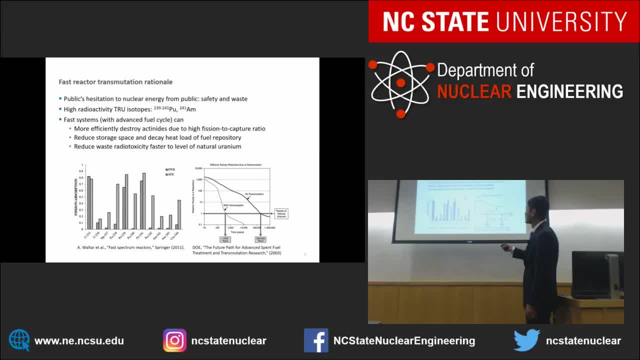 You can destroy it. And here's an example of the process of this, for example, thechant. How about this? You can destroy it And you can destroy it. You can destroy it, You can destroy it. So look. 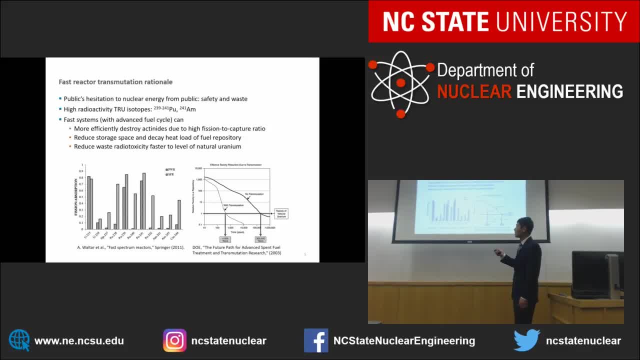 We can destroy this, We can destroy it, but it just cannot be destroyed. Everything is just a waste, But when you destroy it, you take the waste away And you destroy it. That's the good thing. And the water, the water, the waste is gone. 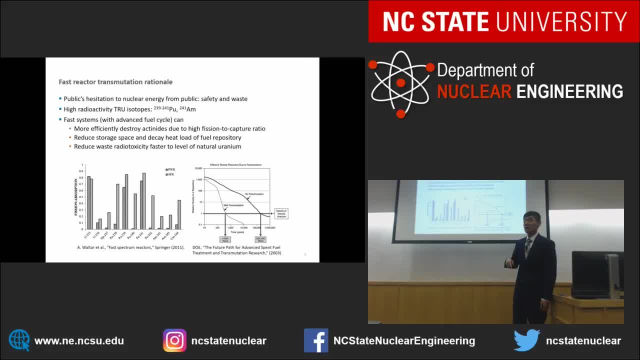 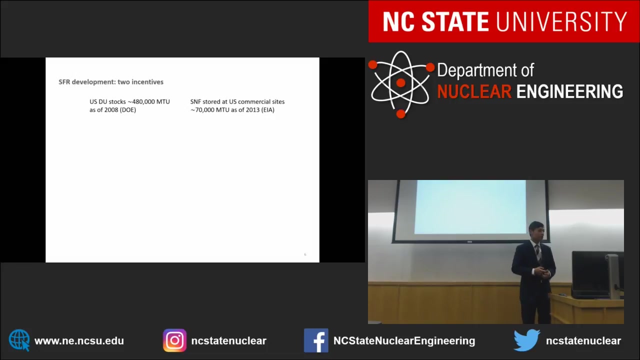 And then that's the worst thing. Okay, I don't know. in light water reactors That means we can reduce by implementing fast reactors with closer fuel cycle and decay heat load of fuel repository And we can reduce waste radio toxicity faster to the level of natural uranium than otherwise. So right now we have 480,000. 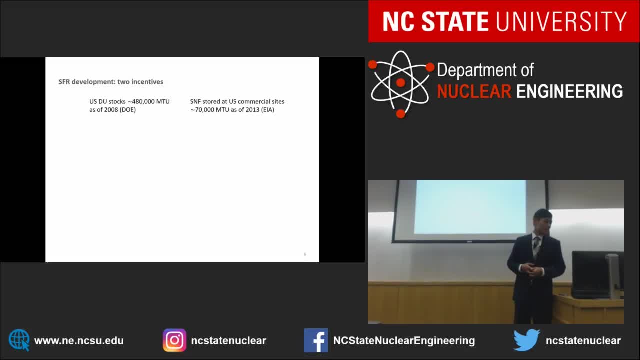 metric tons of depleted uranium in the US and about 70,000 metric tons of spent nuclear fuel in the US And this number is going to continue to grow. And I see a big problem And I also see big opportunity Because for the long term the fast reactors can give. 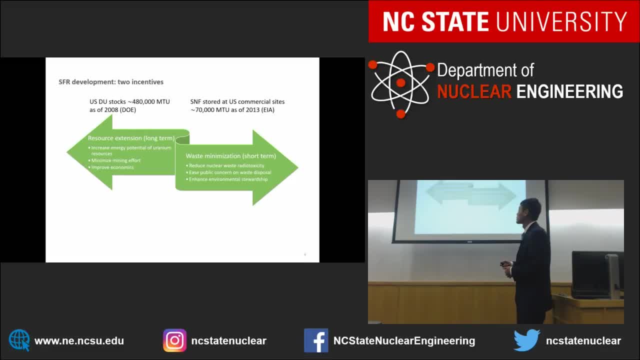 us the solution for the resource extension which I just mentioned. Also, for the short term, we can do the waste with the fast reactors. So that's why I break down this talk in two pieces. I want to talk about the two flavors of this fast reactor system. One is more towards the 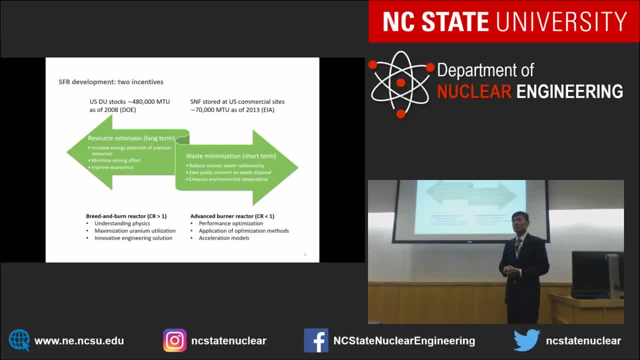 breeder. It's a breed and burn type of reactor which has conversion ratio larger than one. The other is advanced burner reactor which can help us to minimize the waste, which has the conversion ratio less than one, just as light water reactors. 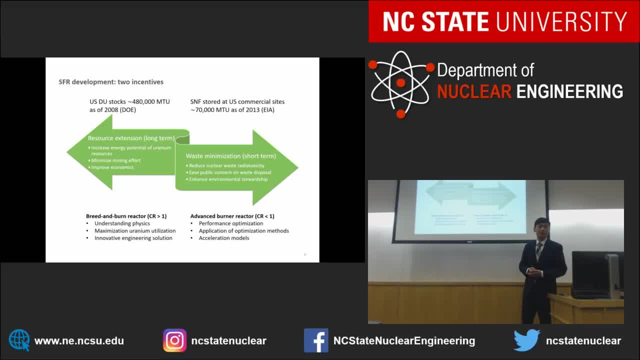 And one nice thing about the fast reactor system is that these two designs are really interchangeable. They're easy to do. You can just change the pitch to diameter ratio in the design. Then you can convert a burner to a breeder. You cannot do this so easily. 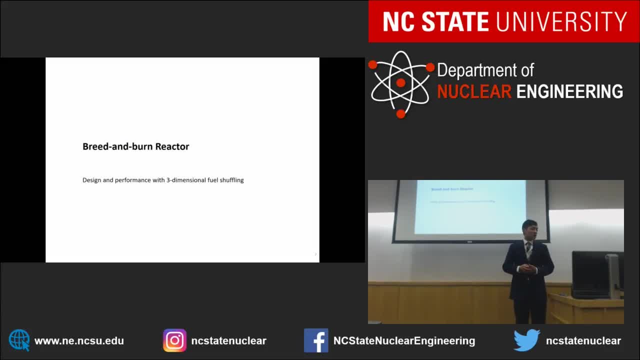 with light water reactors. Okay, so I start with the first part, a breed and burn type reactor. I'll focus on the design, the performance of a three-dimensional fuel shuffling, which I'll tell you why we need this. Okay, At this moment, recycling is not acceptable in the US for a few reasons, And so we really 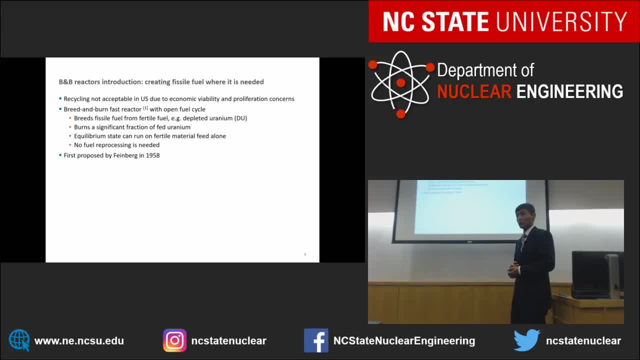 cannot directly go to the fuel reprocessing, But with fast reactor that is operating in the so-called breed and burn mode of operation, we are able to get the fuel back. Now I wanted to mention the method of recycling in a beginner's development. 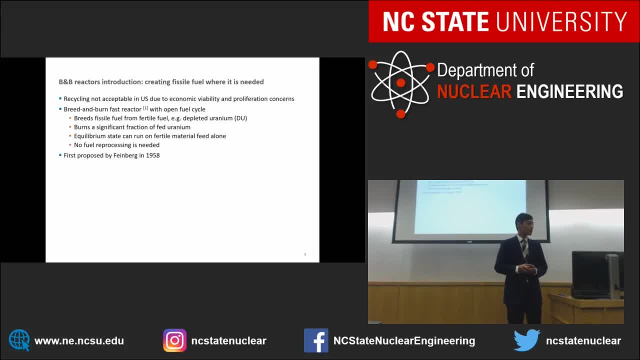 In the past, the method of recycling was very similar to what you can do in a master's lab. In the first step you would release a container and then the container would be washed in a few days, But in the second step you would let the container dry. 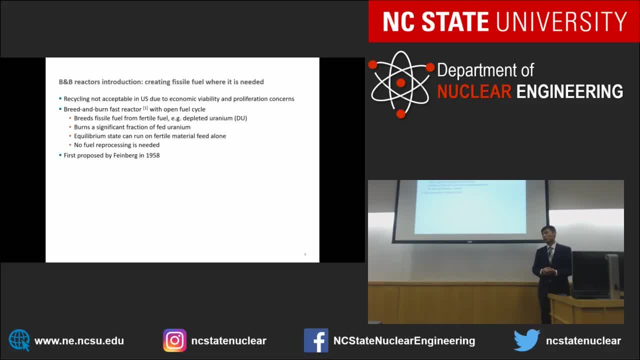 So there are more than a third of the time. the temperature of the container is very different compared to other types of materials, So what we have is that a second batch comes out in the first batch and we have two of the atoms that we're going to be using, and then we have the energy bubbles. 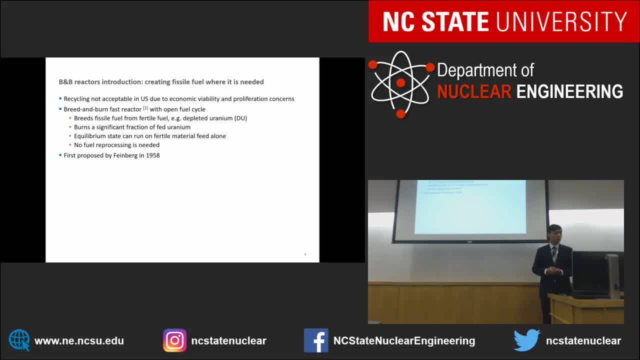 The energy bubbles chocolate. So this is the bottom. there's no need for enrichment. this idea, again, is not something new. has been proposed since 1958. there are two types of the breathe and burn reactors. the first one is so called traveling wave reactor. you probably heard about this. 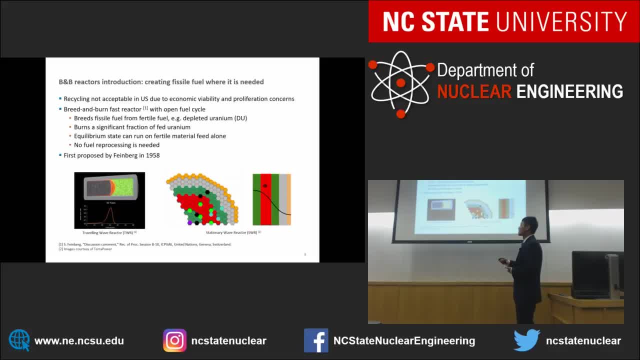 from the tire power design. so the concept is really: imagine you have a candle, you light it from one end- okay, the candles made of uranium 238- you hit the neutron, you light it up. then you start to have the conversion, then fission, more neutrons coming out. this new trans will consume, transmute more. 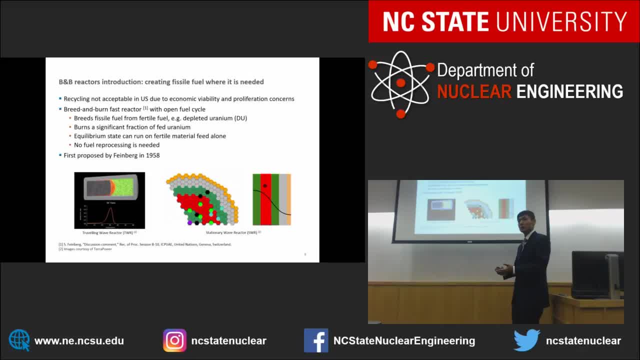 further materials into a fissile, then you continue with a, with a process, so you candle from one end to the other. this is not really economic because the neutrons leaking to the wrong direction will never be able to contribute for the transmutation. so if you have a new neutron, you light it up and you start to have the conversion. 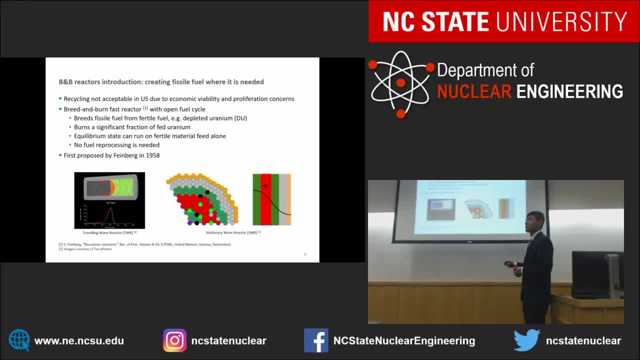 it is more reasonable to design the system so-called stationary wave reactor, SWR. in fact, what's called TWR- traveling wave reactor by the terrapower- is actually a stationary wave reactor. okay, what is done is that instead of having stationary fuel but moving fission wave, we achieve a. 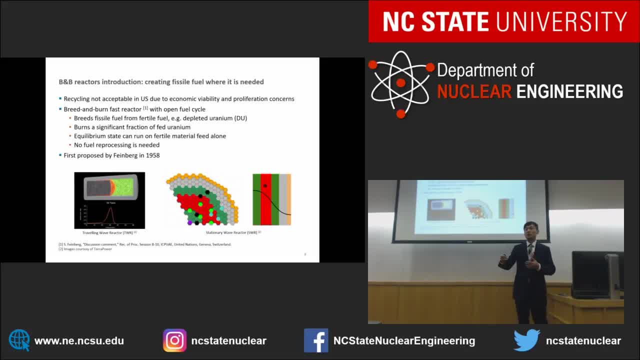 stationary wave of fission. by shuffling the fuel periodically, just as we do with light or reactors, every like 18 months or every two years, we do the maintenance that we, we shuffle, we reload the core and you have relative stationary fission distribution or fission rate wave in a reactor. so we're going to talk about the stationary wave. 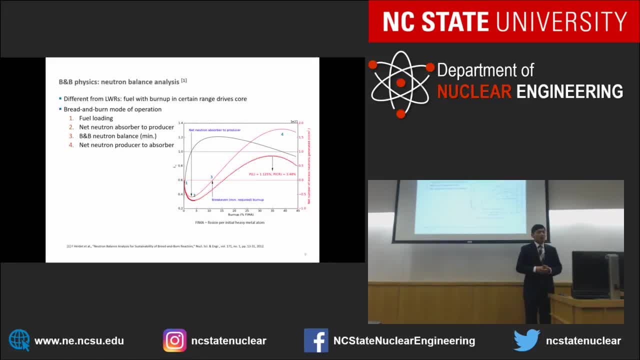 reactor. in this, in this talk, the physics of brilliant burn reactor is significantly different from light water reactors in that remember that in the light reactors, what is really driving the reactor is the fresh fuel, which has the highest reactivity. so that's why you have remember the boron lead down curve. right, you have a curve. 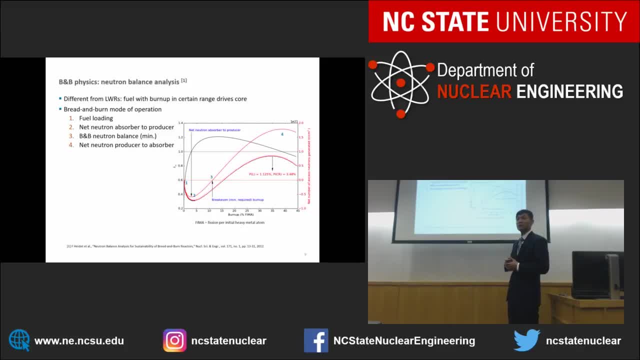 like that of k-infinity over as a function of burn up. but if you feed your brilliant burn reactor with depleted uranium, which is really low reactivity, you start with some low value. okay, if you look at this curve, you start with some low value. then as you burn a few, more fertile material is converted to. 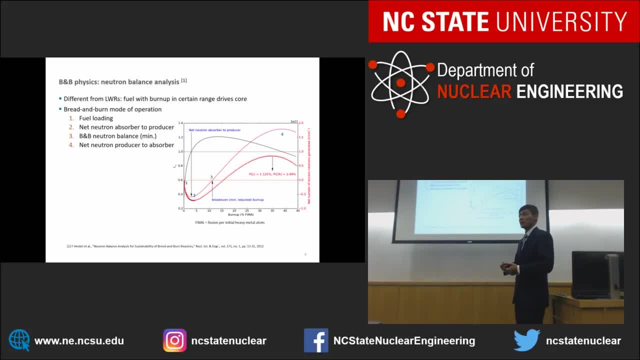 fissile, you turn it to be more reactive fuel. then you see this k-infinity increase and then eventually it becomes less useful and you'll see this curve decrease. so it's important for us to understand that in order to sustain the brilliant burn type of reaction, we really need to burn. 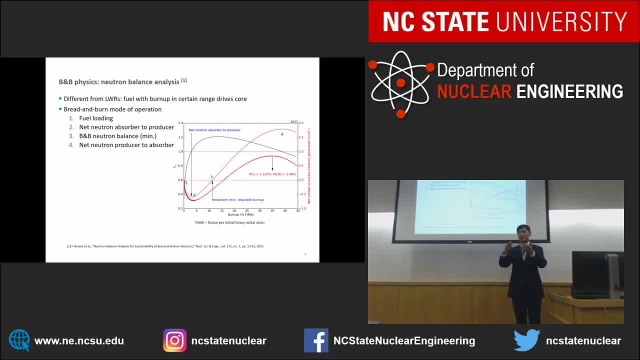 a few to certain burn up. okay, we're not going to use the fresh fuel because they are kind of useless. and so if we look at this net number of excess neutrons, which is just a neutron balance between the production and and the loss, so this is. 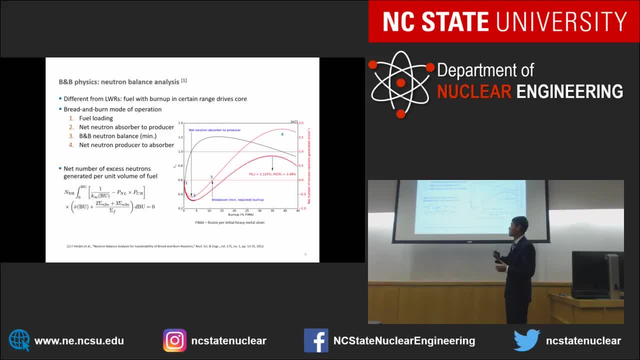 production right, and then you have a loss from leakage, for example, and we call this neutron balance. we count this as the function of burn up and we burn it- sorry, I, we plot it, plot this term- as a function of burn up. this is the red curve. what it shows, that how productive the, the fuel is. so at the beginning you 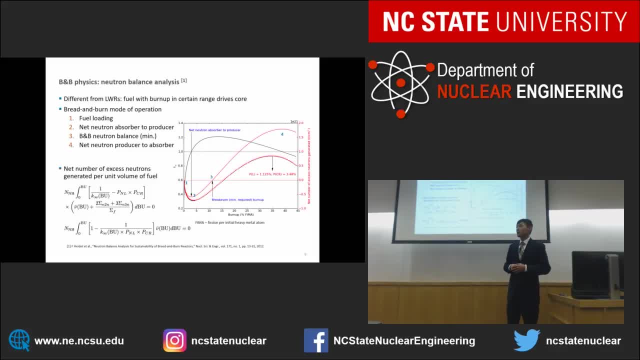 started from zero. the fuel is not producing anything, is not absorbing anything. then, once you start, this fresh fuel is going to absorb neutrons. they're not really giving out any more neutrons. so there are net neutral absorber and it continues until this turning point the neutron absorber will. 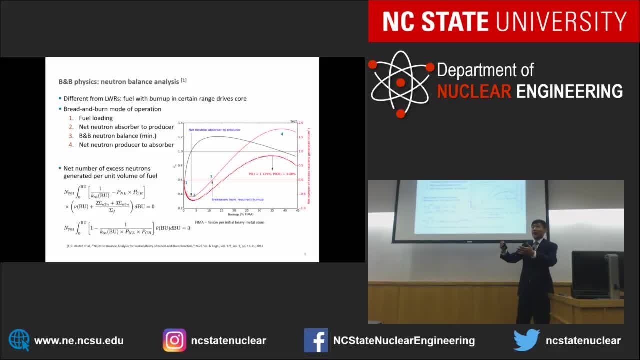 become neutral producer. okay, but this time this fuel has borrowed a lot of neutrons from the bank- neutron bank, if you will. there's a reactor but not have really paid back the debt. it is until this moment that this fuel has paid back all the neutron debt and really contribute to the neutron economy, right? 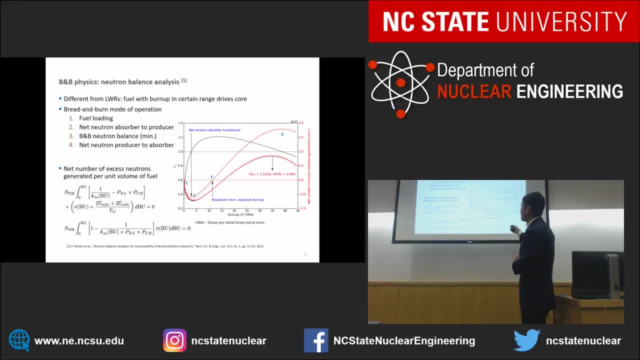 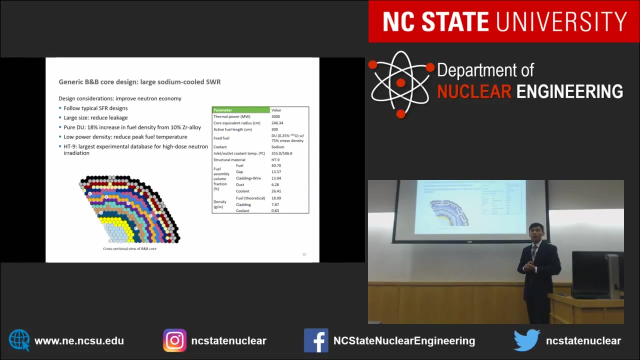 so, and if, from this moment on, it'll be a neutron producer? and this point here, number three, is the minimum required to burn up for for the, for the fuel to achieve. otherwise, there's no way for you to sustain the burn and burn type of operation. so if we are going to do this, we are going to do this, we are going to do this. 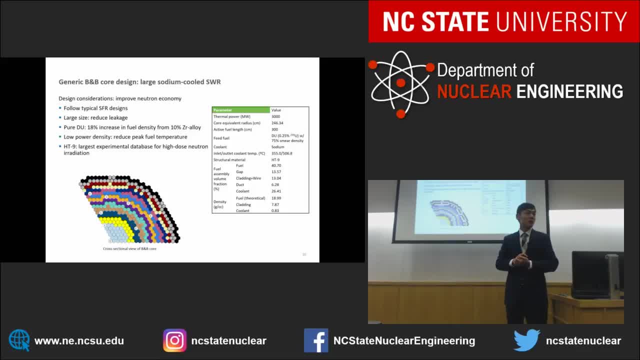 aying a breathe and burn type of reactor based on which is very normal sodium could fast reactor design like this- you have seen this type of figure many times- hexagonal fuel assembly design, and our goal is really to improve neutron economy, the reason being neutrons are so precious because we're 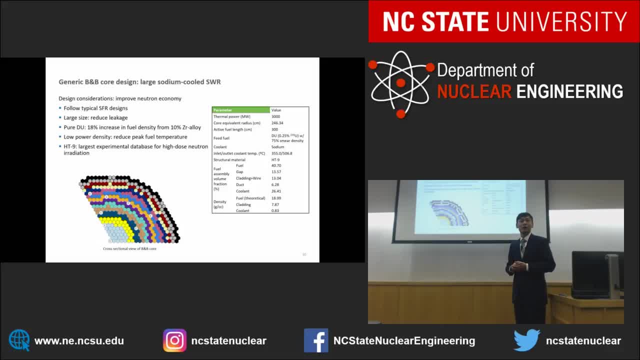 going use them to transmute the fuel. we don't want to lose them, either by absorption or leakage, so we're going to choose a large size of core to reduce the leakage. we're going to use depleted uranium metal as the fuel so that we can maximize the fuel loading and, as a result, we want to lower the. 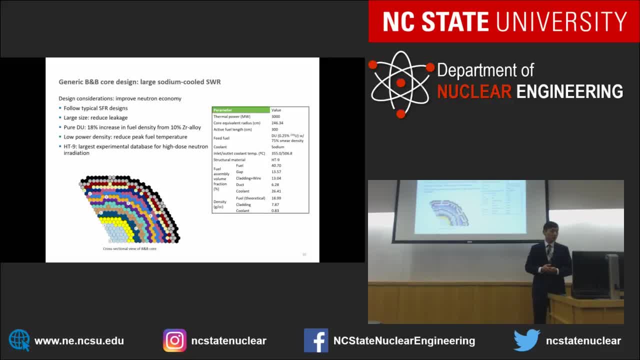 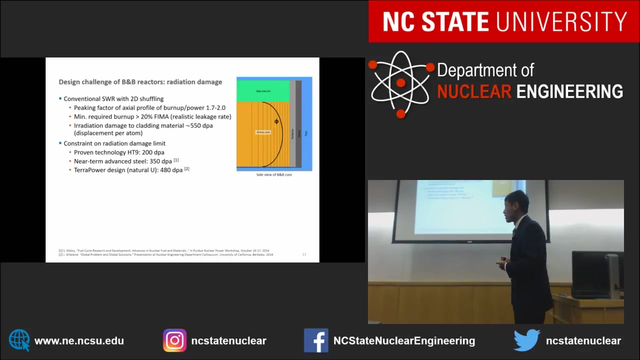 power density of the core to reduce the peak fuel temperature. okay, and we choose hd9 as the cladding or structural material because we know more about their performance in high neutral. Florence table here shows some basic design parameters, characteristics. but there's a challenge with this design. 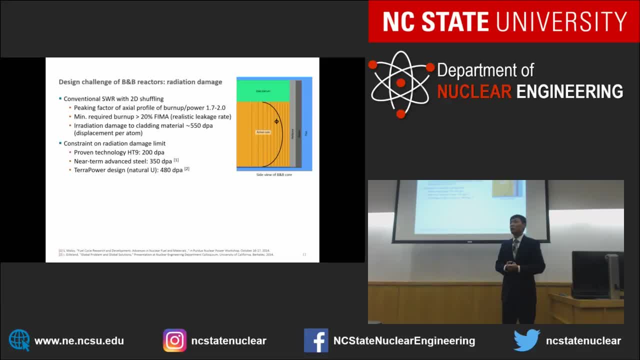 because usually you will see a high peaking at the center of the core in terms of flux or power. remember this fuel has to stay in the reactor long enough to be a neutron producer. that means the fuel or the structural material in this elevation will see a lot of radiation damage coming from the fast spectrum coming. 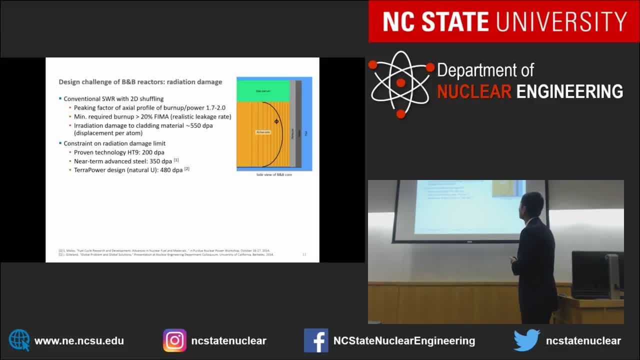 from the fast neutrons. this is a fast spectral reactor. if you exceed 20% FEMA, that's a unit of burn up. so 20 of 20 percent of the heavy metal has been has been used and you're talking about 550 dpa displacement per atom. that's how. 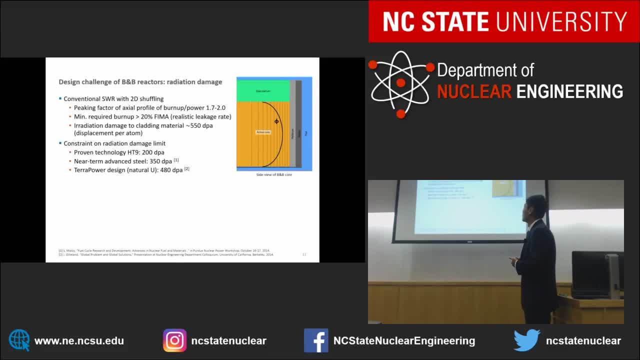 much radiation damage that will cost to this field. we only have experience with hd9 on the level of 200 EPA. okay, it doesn't mean that deep the hd9 will not survive beyond that, beyond this, this damaged level, but we just don't know. with a new advanced material development, you know. 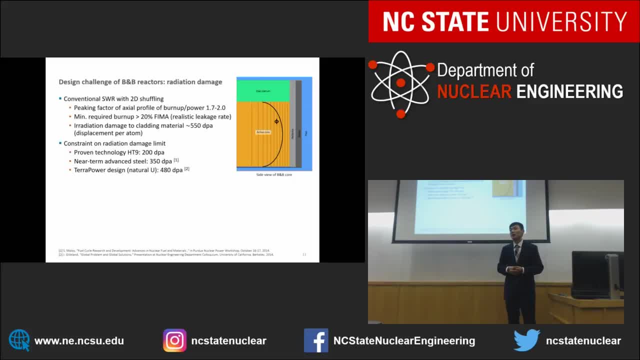 it's just suggested, 350 dpa is probably a realistic expectation. so our goal is to really bring down the radiation damage level from 550 to 350.. How do we do it? Well, the idea is that if we can minimize the axial peaking of the flux and the power, 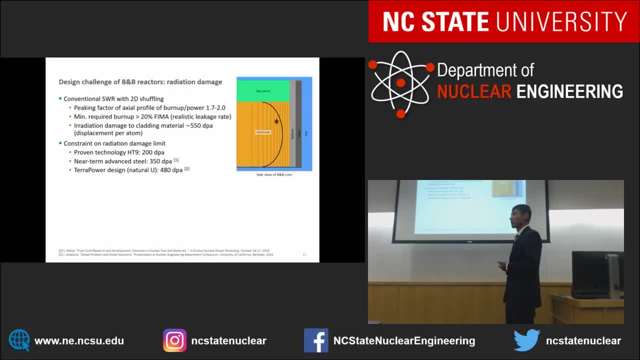 then we should be able to bring it down the radiation level. So the first thought to this is that if we can design a pebble bed reactor where the fuel is continuous flowing, circulating, then we should be able to minimize the radiation damage distribution or profile. But we tried that. it did not work. 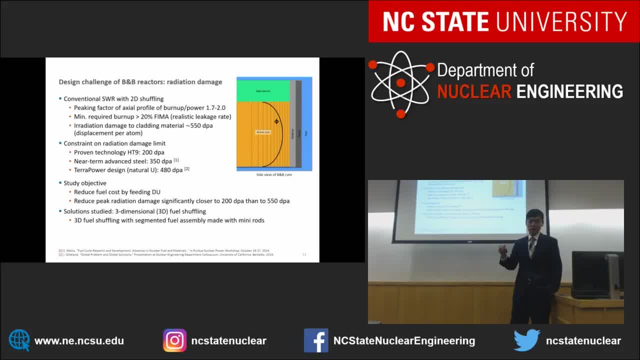 because of many reasons. One of them is that if you have pebble and the fuel volume fraction in that pebble is kind of limited, So you cannot really produce enough neutrons to contribute to the neutron economy. So we decided that we want to stay with the normal fuel assembly design. but 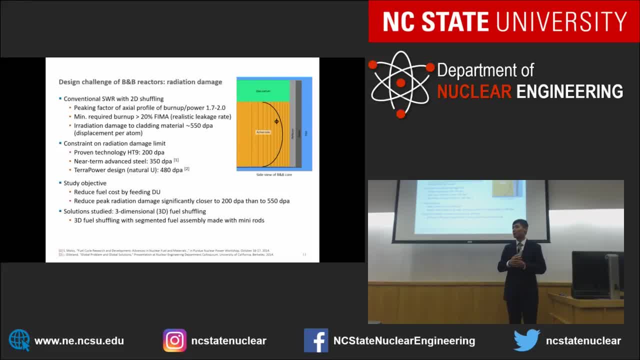 we want to chop the fuel assembly into different pieces in axial direction, and every time we reload we shuffle the fuel. when we not only relocate assembly- you know different radio locations- but also we change their axial location so that, with the hope that we can minimize the peaking in the radial Zeus position. 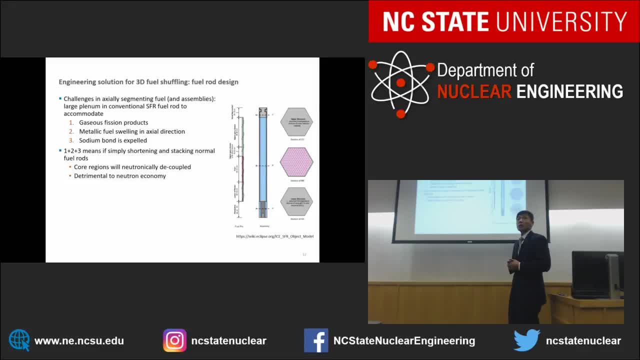 the radiation damage level. well, the issue with this is that- remember, in the fast record designs are always a large plenum either on top or bottom of that fuel rod base is necessary to accommodate fission products, fuel swelling and sodium bond. if we simply chop the fuel rod in this way and the 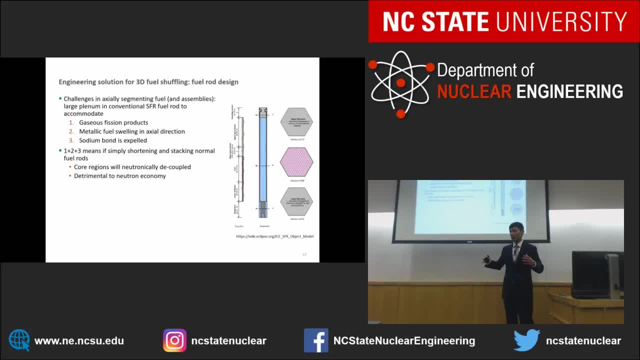 core regions will be neutronics decoupled because there will be void inside the core. it's gonna hurt you in the neutronic performance. this is that we want to remove this large plenum. we wanted to implement direct venting of the fission product into the coolant and we want to use mechanically bonded 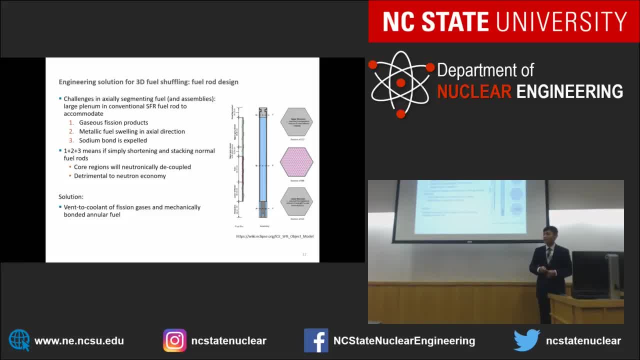 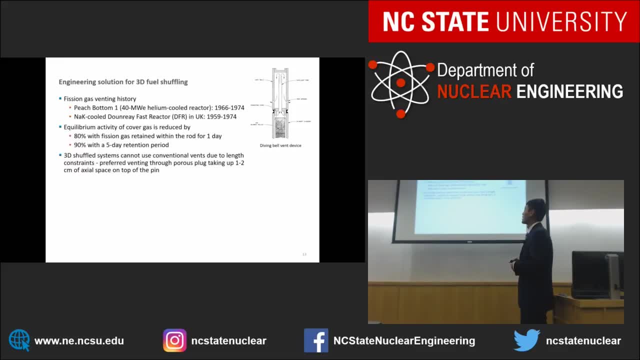 annular fuel. direct venting of the fission product. it is is not something crazy. there has been cases, successful cases- for this. for example, pitch bottom one, which is a gas cooled reactor used directly venting. a neck cooled reactor in UK has been using direct venting of the fission products before and for the annular fuel. our goal. 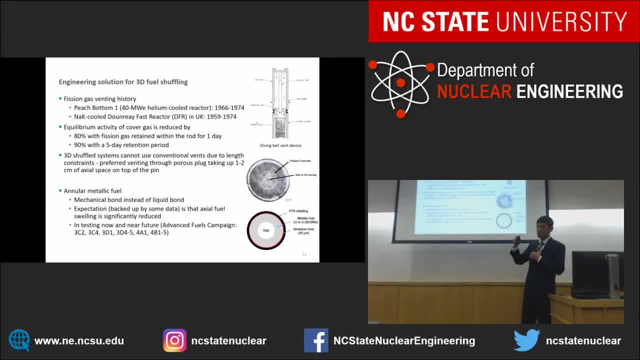 is to minimize the axial fuel swelling by putting a bound between the fuel and the cladding and this type of and we use the annular fuel so that we can further minimize swelling. this type of fuel has been tested in advance. the fuel campaign in this series, so again. 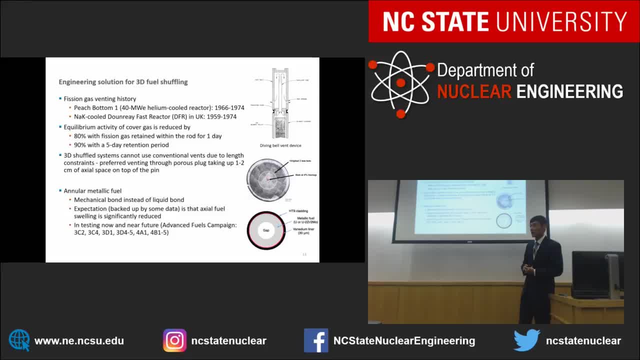 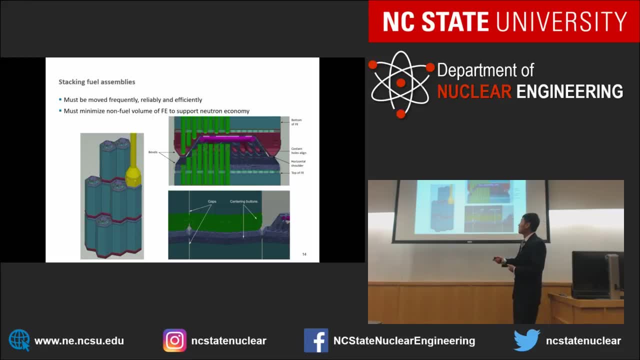 this is already. have some experimented data backup on the design. so these are the designs that come up with for the fuel assembly- shortened assembly, stack on top of each other. this is also a shuffling machine that can lift the fuel assembly. there are some small designs: gaps, centering buttons, bevels to make. 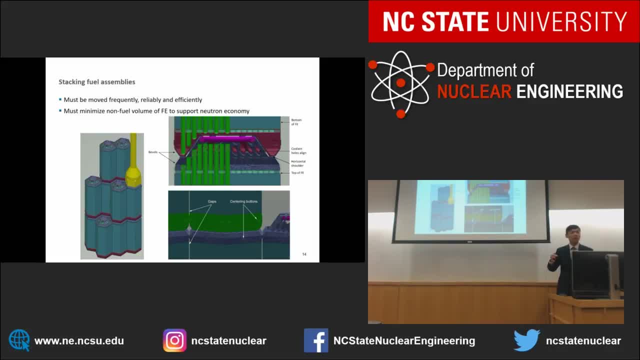 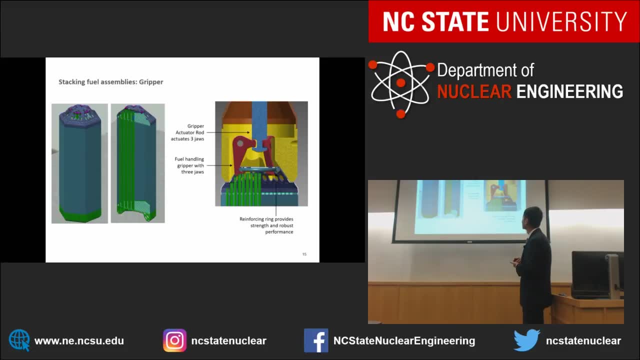 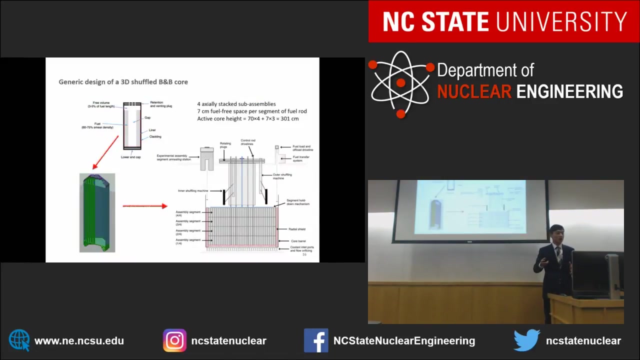 sure that the fuel assembly is well aligned in both radial and axial direction. now the close-up at the fuel assembly. this is how the shuffling scheme will- sorry, the shuffling machine will- work. there is a jaw reaching out and reaching down and the grip reinforcing ring. so we redesigned the fuel rod and 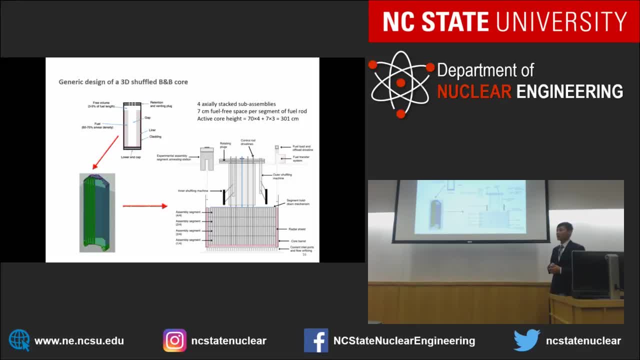 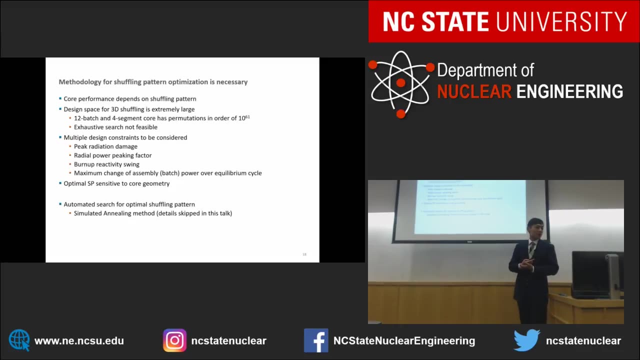 put it together, a new design of a fuel assembly, then your core now have four layers of a fuel assembly which will facilitate the 3d fuel shuffling. and then we need really to define what are our goals. our goal is to first minimize the peak radiation damage, but also, at the same time, we want to minimize the 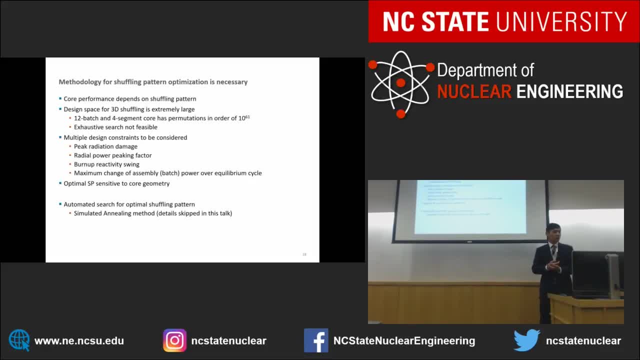 radio power picking factor. we also want to minimize the burn up reactivity swing, to reduce the burden on control rods etc. so this is the multi objective optimization problem, and so we design this optimization met scheme to find the best shuffling scheme. but I'm gonna skip the details in this talk. 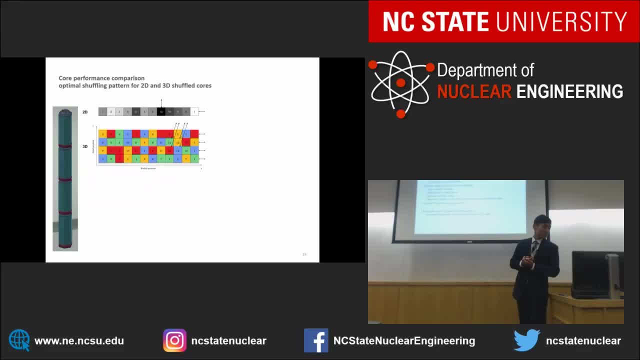 because in the second half I'll talk more in details. so in the end, let's say magically, I got this shuffling scheme coming from up, going to compare what I can achieve with a 3d shuffling with a 2d, the 3d shuffling. here is the shuffling scheme, core, Center, core. 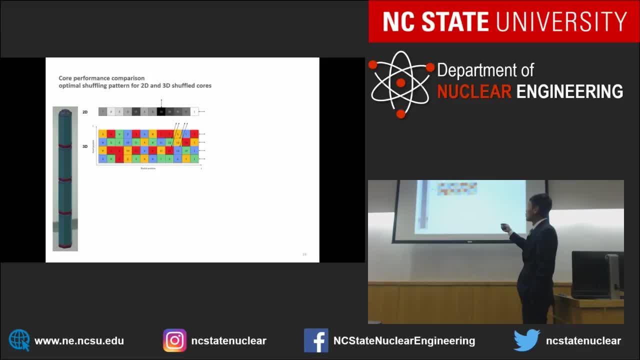 boundary feels loaded at boundary as number one: fresh fuel. next cycle jumps to this location and three and four and started jump back and forth within 12 cycles. after 12 cycles are going to be released. 3d shuffling is more complicated. the fuel assembly as a whole is loaded on the periphery. then 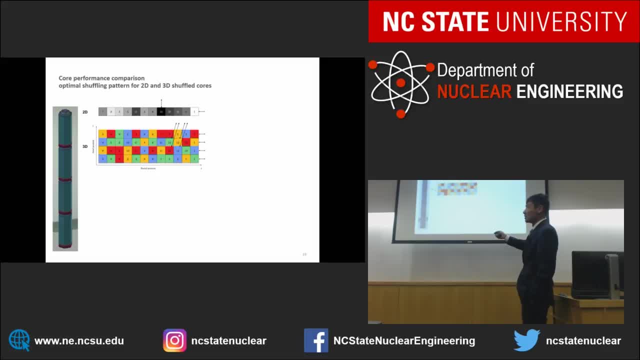 the top part is going to this location and then this location. if you follow that number each, the color does not change. then because of the symmetry of the problem, the bottom one will go to here and then here. the middle ones will follow a different path, but eventually they'll all be discharged from this. 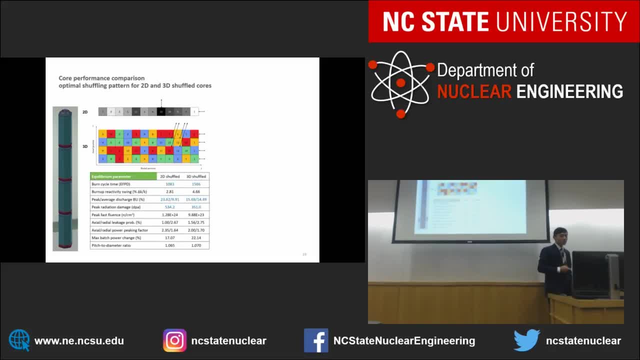 location. so how do pyro looks like from a channel focus? so now let's compare the performance with 3d. shuffling what I first noticed us that the peak rain damage has been brought down to 351. remember our goes 350. we're not there, but really extremely close, comparing especially with the 2d. 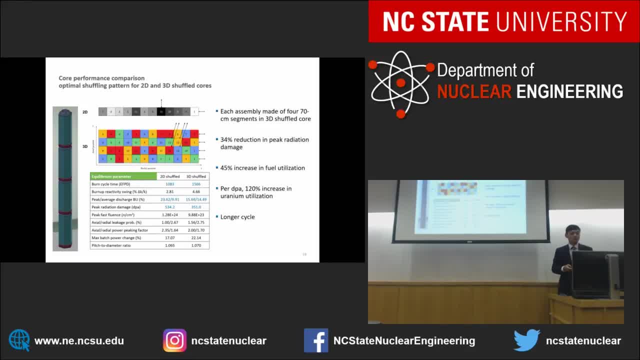 shuffled case 534, that's, you know, 34% decrease they will. also, if you look at the discharge burnup average fuel is cloud 4. most of you guys can see that 5X is five percent of peroxide. that's here tip number six. they're going to cool down quickly. a little bit of heat, ah, and then it agree with my report: still not leveled. so this is how u power works. 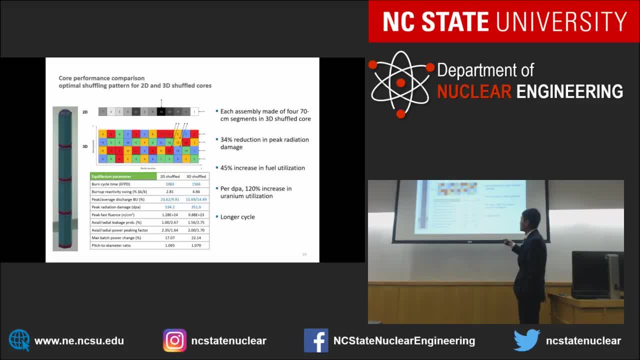 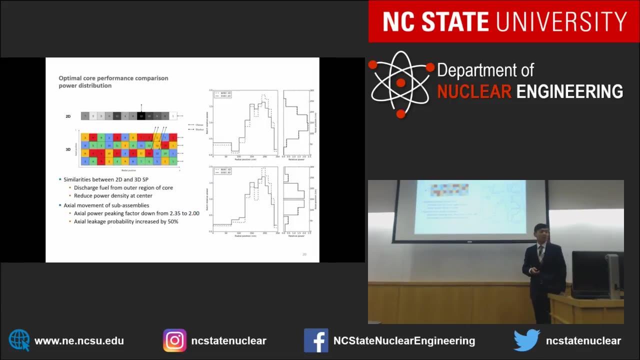 average discharge burn up 10% versus 14.5 shows 45% increase in a few utilization. much longer fuel cycle in days. so if I compare the shuffling scheme I do see similarities. fuel loaded at the boundary, jumping to the center, then back and forth in the inner and outer core. I does the optimizer tell me to do so? 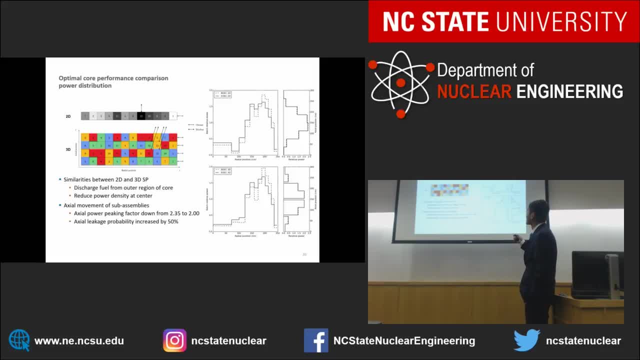 because that it really creates a low at radio power picking at a core center. this is radio power profile center and the boundary in 2d and 3d case. they look very similar because they that's what the ultimate optimizer was trying to do: minimize the power at a center so you can reduce the picking. 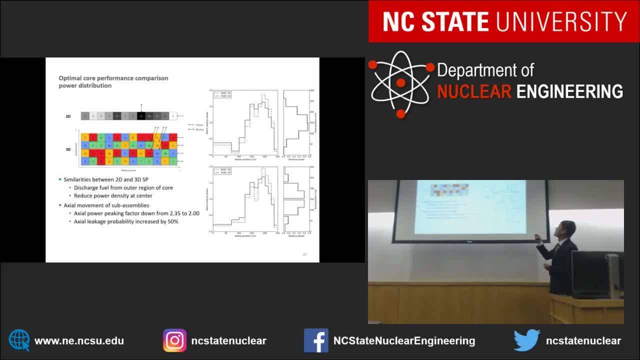 factor on radiation damage. but what it really is helping here is the actual power picking factor side way. if you look a side way, the power picking factor has been brought down from two point three, five to two in 3d shuffled case. but then the question is: well, if you do that, then your axial leakage probability will. 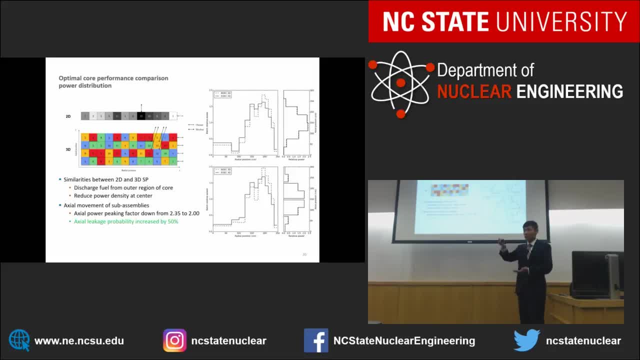 increase a lot by 50 if you push the center, then leakage on the top and bottom of increase. but you said at the beginning we're trying to save as much as possible neutrons because they are really important for the neutron economy. so how does this help? it's kind of counterintuitive. the way it helps can be. 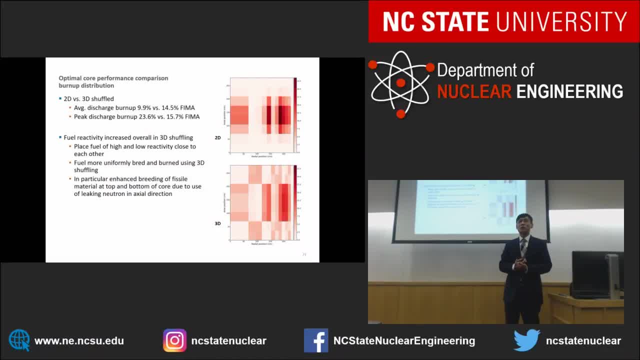 seen here if I plot the distribution of burnout of the fuel in the 2d shuffled and 3d shuffled case, again the side way, okay, my fuel is loaded at the, at the outer boundary, then this fresh fuel, so they're white. then as they're moving they start to collect. 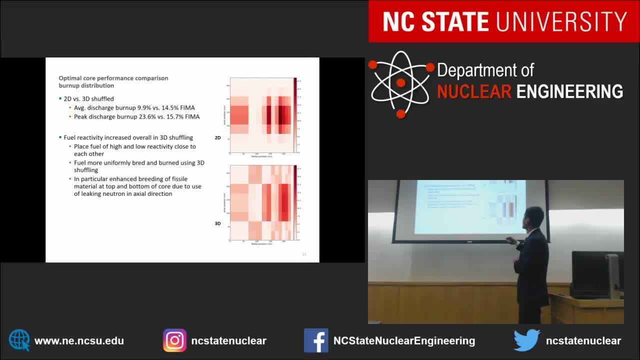 burn up. as they continue to be burned in a fuel, the color becomes darker and darker. this is where you get discharged, really dark. right, this is a 2d case. you don't really see burn up on the top and bottom of the core because there's neutrons. but if you look at the 3d map, 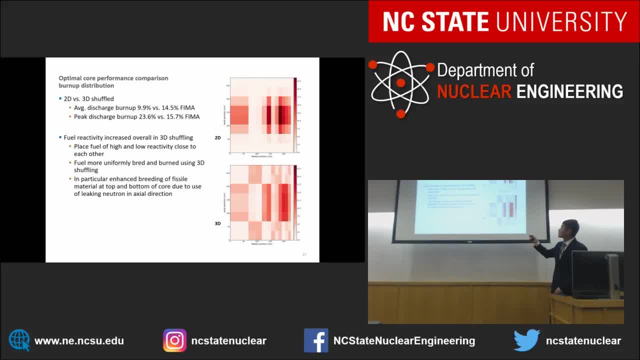 fuel is loaded here, but then quickly they're moved to the top and bottom of the core where they really sitting next to the high reactivity fuel. they can receive neutrons and to be transmuted to be more usable fuel. so that's why we see more red color on the top and the bottom of the core. 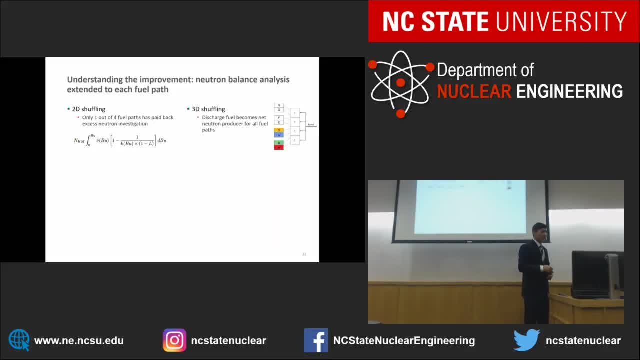 that is really helping us. and remember i showed you the red curve at the beginning as a neutron balance in, so i'm going to compare the 2d and 3d case. i discretize the assembly into eight pieces axially because of symmetry. i only look at the four pieces at the bottom as they 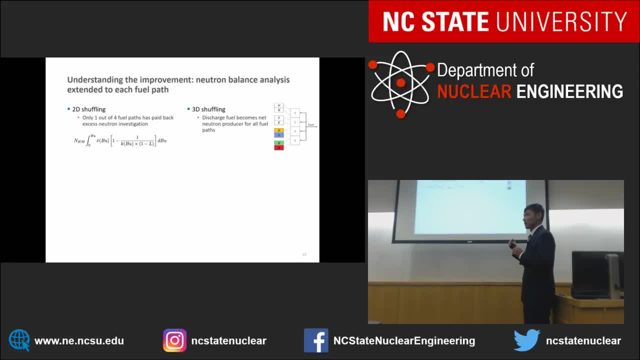 move across the reactor. they pick up, burn up. then we can follow each of this piece to plot the neutron balance or neutron life. again, at the top and bottom they're almost all metal that's whispering to each other. gl delayed in the field. so it's because of symmetry. this is the water will 여기는. 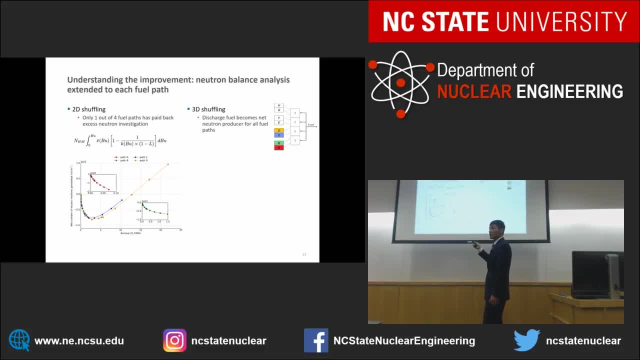 the energy source of very low pressure. it can reach zero concentrations. if you look at the first three pieces, it will decrease a lot. so this is the reason it will decrease a lot. this is the result of the neutralization. so that's what we're looking at right here. 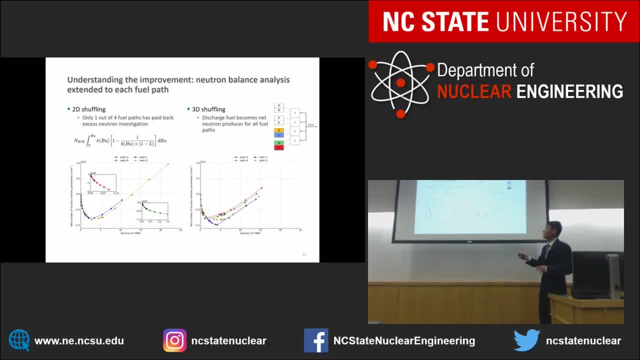 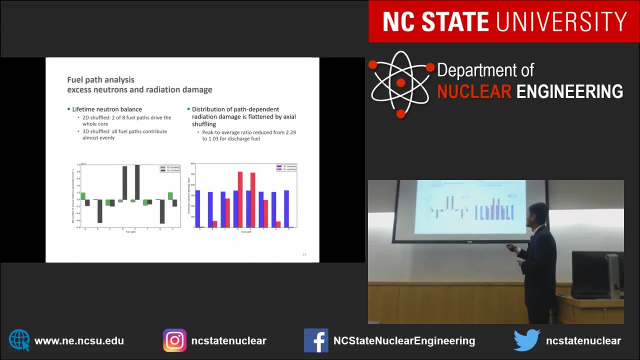 so the mustard gas went very, very high. the newly, Jacqueline des, tossed those gas right here almost evenly to the neutron economy. So that's why we can bring down radiation level or peak radiation level, because we can even those radiation across the fuel segments. Another way to look at this is lifetime. 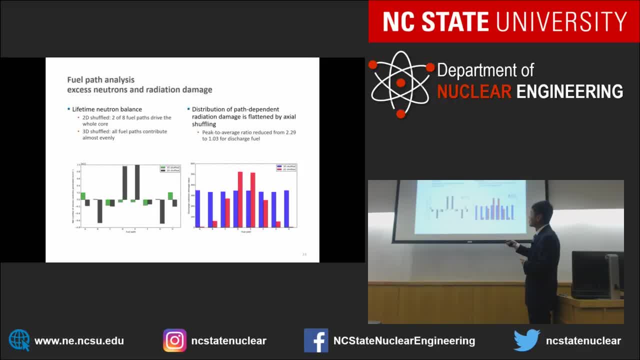 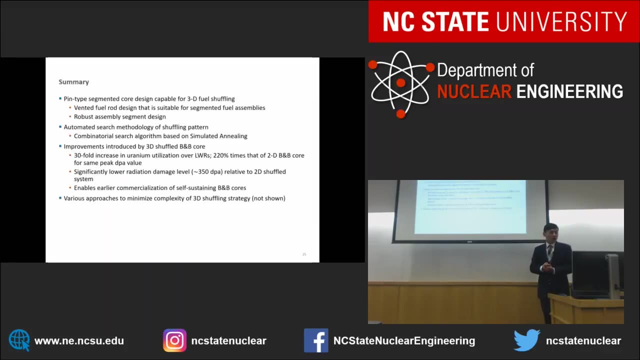 neutron balance. for the 2D, The gray ones really hide the center, but for the 3D case it's much more evenly distributed Radiation damage level. same thing. Okay, So that's the first part of this talk. I showed you how you design reactor. 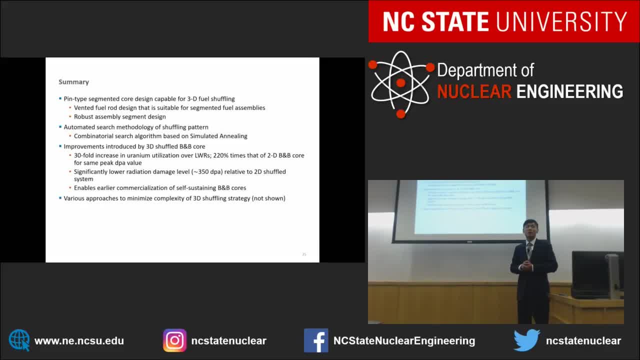 assembly and the shuffling scheme to facilitate the 3D fuel shuffling which really helps to bring down the radiation, that peak radiation leaf dam难, so that we can use that more realistic materialạt, material bound to facilitate, to actualize the breed and burn type of 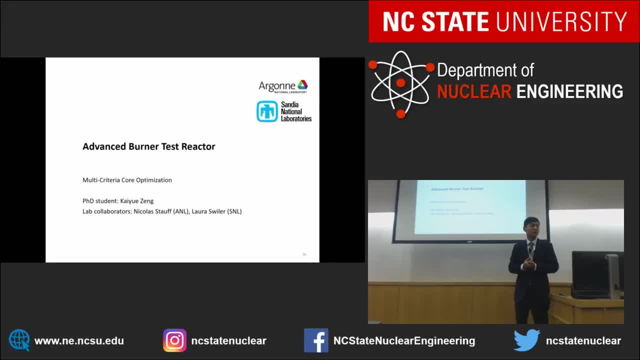 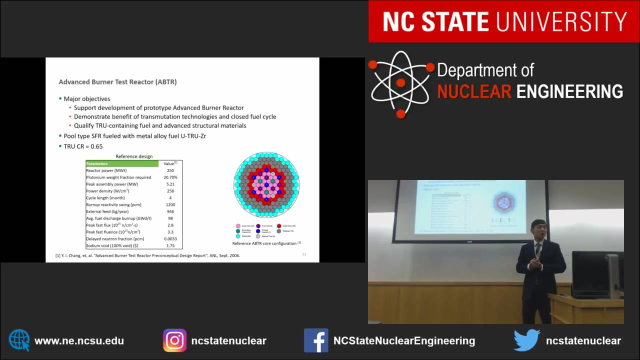 mode. so now switch to the next product, the multi criteria core optimization of advanced burner test director. this is what we've done, together with our national lab and Sandia National Lab- the student who did this actually sitting in the audience- and the ABTR is a small-scale advanced burner reactor. 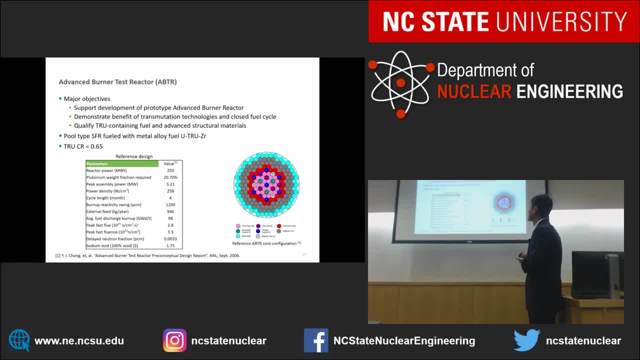 which was designed to support the development of the prototype of the advanced burner reactor, and it has the conversion ratio- no surprise, less than one. I use the fuel made of uranium, transuranic and zirconium. so this is the code that we're going to use for the ABTR, and we're going to use the code that we've used for the ABTR and we're going to use the code that we've used for the ABTR and we're going to use the code that we've used to simulate this used for the ABTR, and we're going to use the code that we've used to simulate this. 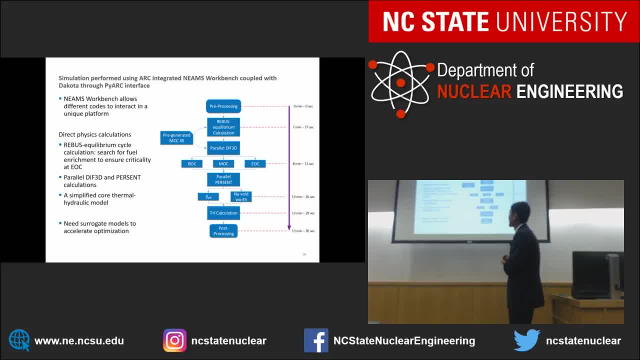 used for the ABTR and we're going to use the code that we've used to simulate this rack. we use the nemes workbench that use the code that we've used to simulate this rack. we use the nemes workbench that use the code that we've used to simulate this rack. we use the nemes workbench that integrates all the major software that for. rack. we use the code that we've used to simulate this rack. we use the nemes workbench that integrates all the major software that for rack. we use the code that we've used to simulate this rack. we use the nemes workbench that integrates all the major software that for the faster reactor simulation. there's a. 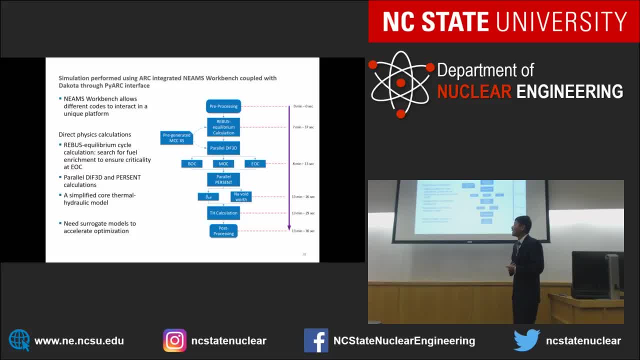 the nemes workbench that integrates all the major software. that for the faster reactor simulation. there's a the nemes workbench that integrates all the major software that for the faster reactor simulation. there's a complete process of doing this calculation, the main complete process of doing this calculation, the main. complete process of doing this calculation. the main takeaway here is that it takes. takeaway here is that it takes. takeaway here is that it takes about 13 minutes to evaluate one core. about 13 minutes to evaluate one core. about 13 minutes to evaluate one core design which seems fine, but eventually, 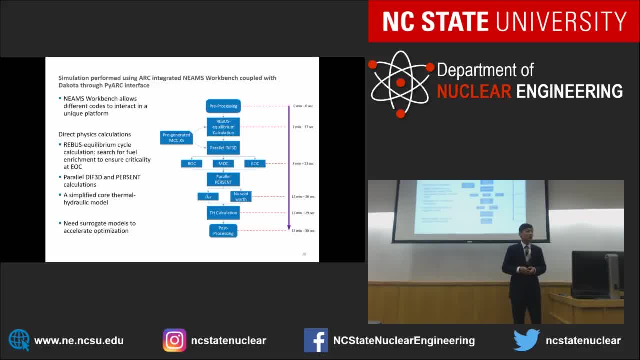 design which seems fine, but eventually, design which seems fine, but eventually, when we're doing when we're doing the, when we're doing when we're doing the, when we're doing, when we're doing the optimization, it is, it's going to be a optimization, it is, it's going to be a. 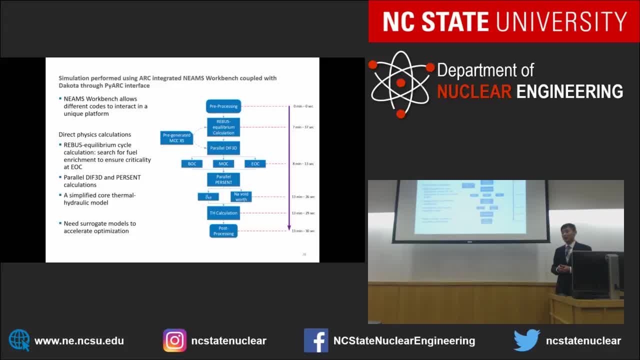 optimization. it is. it's going to be a limiting factor, because it will be limiting factor, because it will be limiting factor, because it will be looking at thousands of cases, just to looking at thousands of cases, just to looking at thousands of cases, just to find the best design. and how do we do? 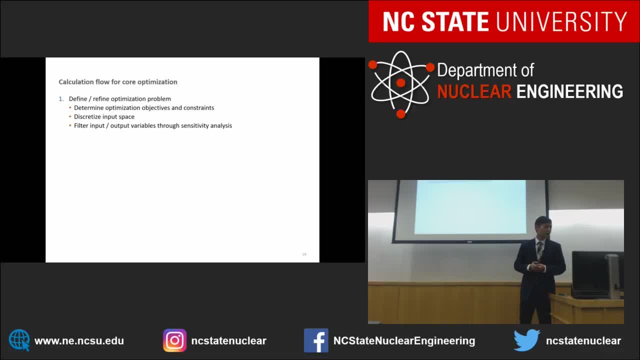 find the best design. and how do we do find the best design and how do we do the core optimization first. we need to the core optimization first. we need to the core optimization first. we need to understand what, what we need, we define, understand what, what we need, we define. 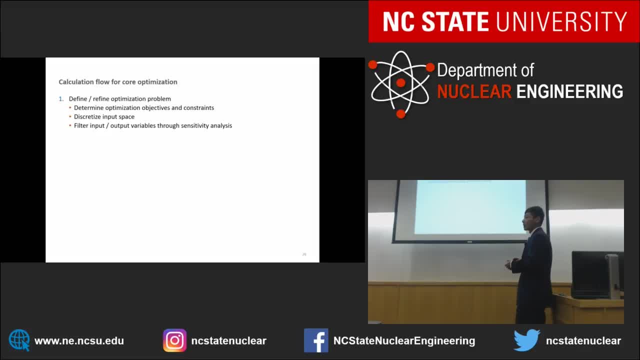 understand what, what we need, we define and we refine optimization without the and we refine optimization without the and we refine optimization without the inputs. what are the objectives? second, I inputs. what are the objectives? second, I inputs: what are the objectives? second, I choose the right optimization method. 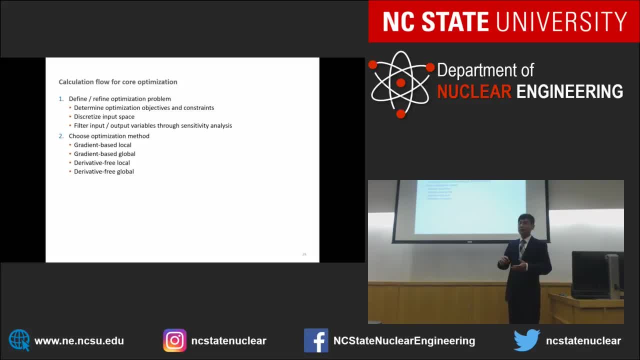 choose the right optimization method. choose the right optimization method: gradient-based or derivative, free, local or gradient-based or derivative, free, local or gradient-based or derivative, free, local or global optimization. global optimization- global optimization. next one: if it's too slow, should I be using? next one: if it's too slow, should I be using? 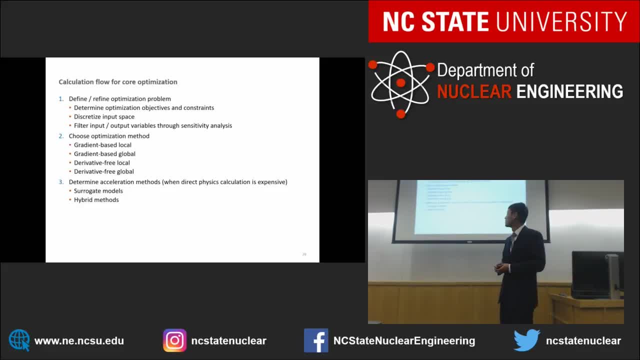 next one: if it's too slow, should I be using some acceleration technique? like some acceleration technique, like some acceleration technique, like surrogate model? next one is: how do we surrogate model? next one is: how do we surrogate model? next one is: how do we choose the final solution? because this: 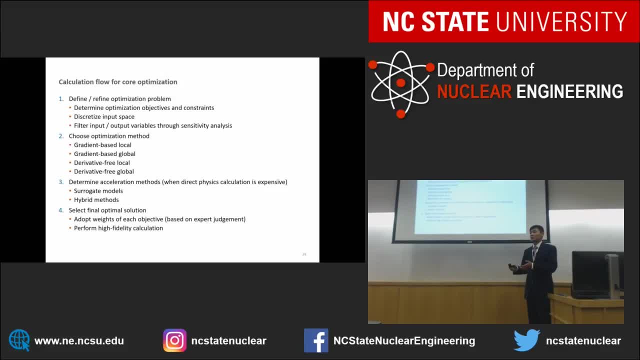 choose the final solution because this choose the final solution because this optimizers will give you a set of near optimizers will give you a set of near optimizers will give you a set of near optimal solution. it's not gonna tell you optimal solution. it's not gonna tell you. 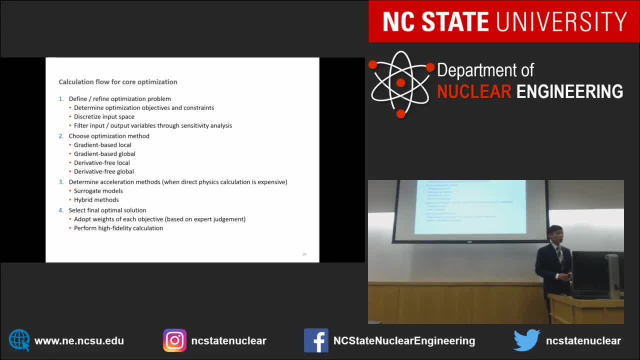 optimal solution. it's not gonna tell you which one is the best. the end of the day. which one is the best the end of the day, which one is the best? the end of the day, it is you who is going to teach or pick. it is you who is going to teach or pick. 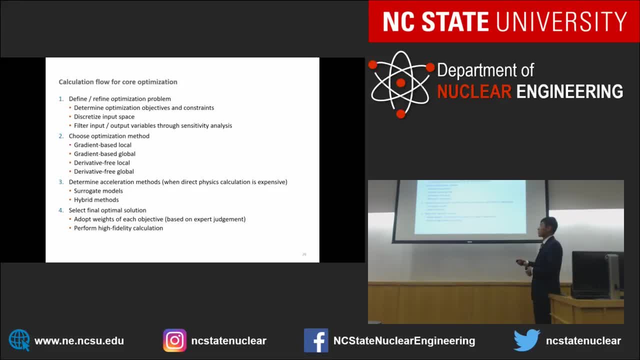 it is you who is going to teach, or pick the most favorable one and perform the the most favorable one, and perform the the most favorable one, and perform the high-fidelity calculation on that. so high-fidelity calculation on that. so high-fidelity calculation on that. so what is our problem? we wanted to design. 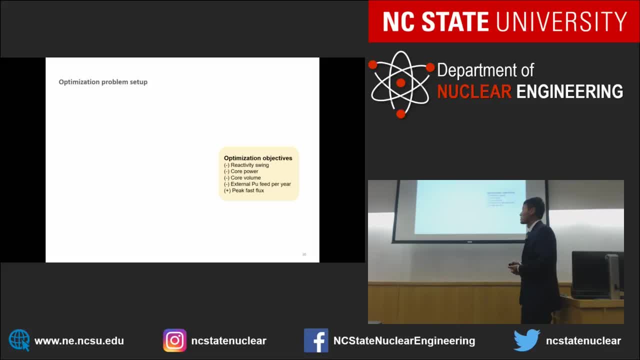 what is our problem? we wanted to design. what is our problem? we wanted to design a BTR that has low reactivity swing. okay, a BTR that has low reactivity swing- okay, a BTR that has low reactivity swing- okay, that's. we want to reduce the burden on. 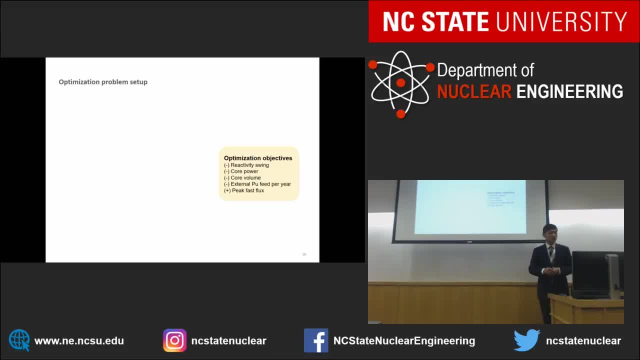 that's, we want to reduce the burden on that's. we want to reduce the burden on the control rods and we want to minimize the control rods. and we want to minimize the control rods and we want to minimize the core power- core volume for the cost. the core power- core volume for the cost. 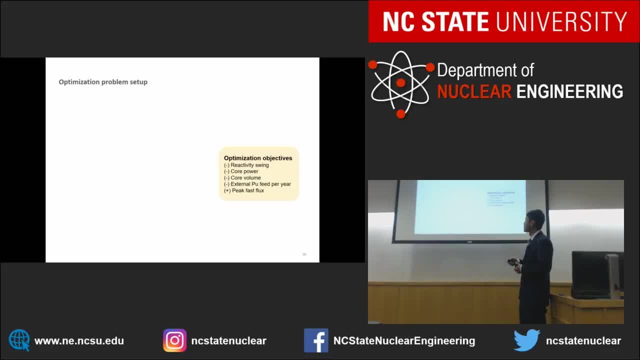 the core power, core volume, for the cost reason, and also we want to minimize the reason, and also we want to minimize the reason and also we want to minimize the external plutonium, because plutonium is external plutonium, because plutonium is external plutonium, because plutonium is also be feeding the reactor and by the 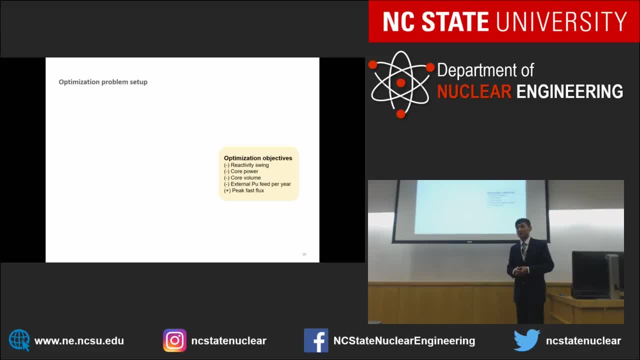 also be feeding the reactor and by the also be feeding the reactor and by the same time I want to maximize my peak. same time I want to maximize my peak. same time I want to maximize my peak- fast flux, because this is a test. fast flux, because this is a test. 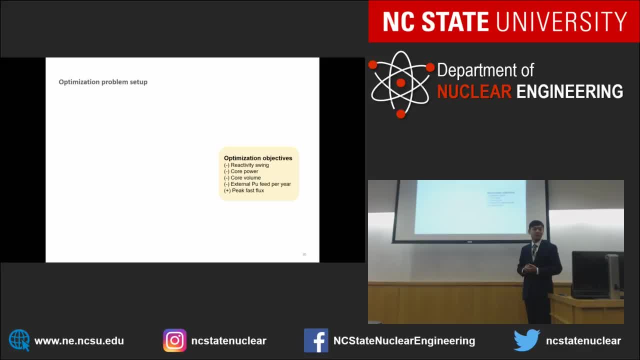 fast flux because this is a test director. I want to have high level of director. I want to have high level of director. I want to have high level of fast flux for the material testing. I can fast flux for the material testing. I can fast flux for the material testing. I can change a few things to achieve this goal. 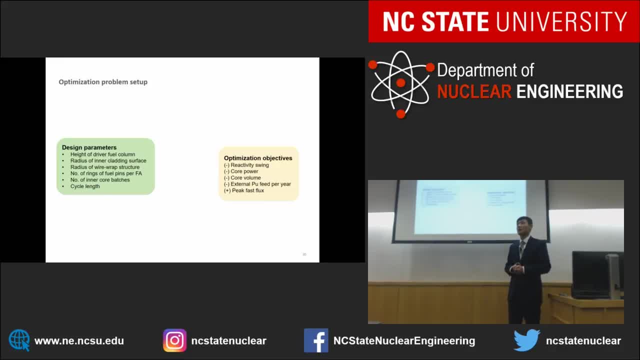 change a few things to achieve this goal. change a few things to achieve this goal. these are my design parameters. I can. these are my design parameters. I can. these are my design parameters. I can. change the dimension of the fuel rod. how change the dimension of the fuel rod? how? 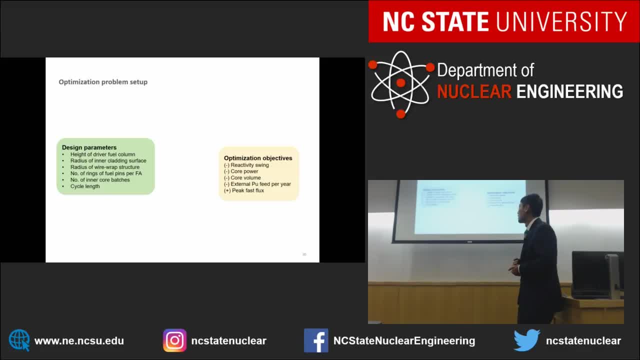 change the dimension of the fuel rod. how many rods are included in each fuel? many rods are included in each fuel. many rods are included in each fuel assembly, even the cycle length, etc. okay, assembly, even the cycle length, etc. okay, assembly, even the cycle length, etc. okay. ISO identify the input and output. 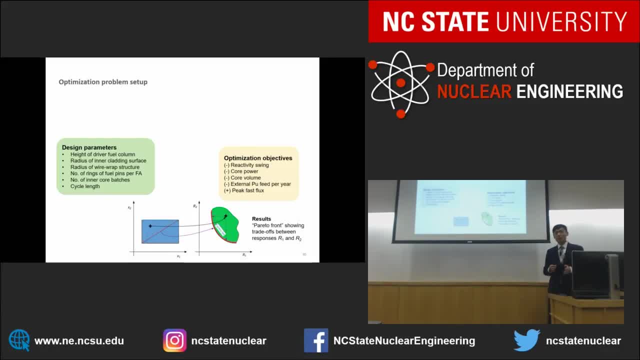 ISO identify the input and output. ISO identify the input and output. hopefully you know I can from this. hopefully you know I can from this. hopefully you know I can from this relation. I can get from the relation relation. I can get from the relation relation. I can get from the relation from input to output. I'll be able to. 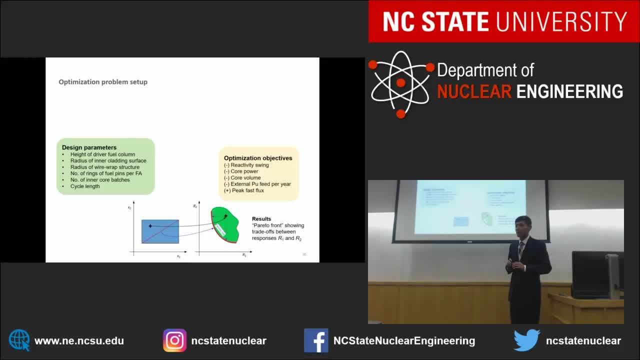 from input to output. I'll be able to. from input to output, I'll be able to identify my bias and my best design. but identify my bias and my best design. but identify my bias and my best design, but that's not enough, because if you look at, 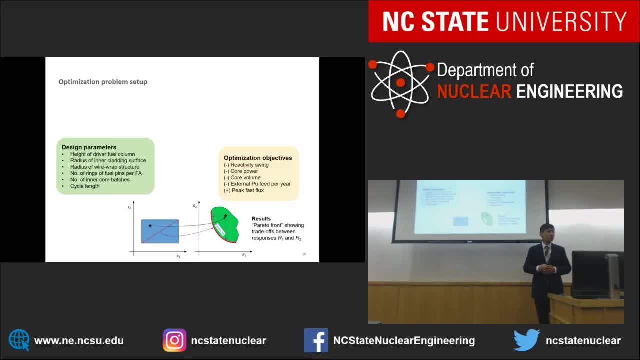 that's not enough, because, if you look at, that's not enough. because if you look at those optimization, our optimization, those optimization, our optimization, those optimization, our optimization objectives, some of them are actually objectives. some of them are actually objectives. some of them are actually contradicting which with each other. for 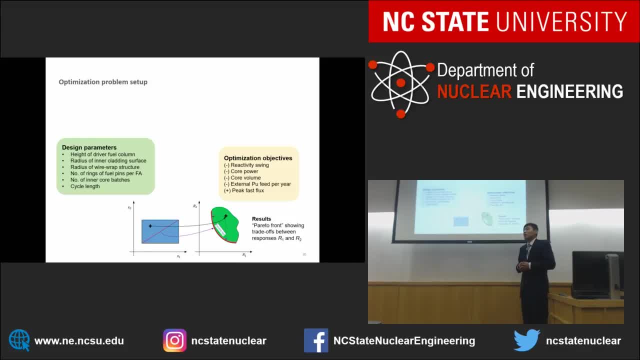 contradicting which with each other for contradicting which with each other. for example, if you want to lower the core example, if you want to lower the core example, if you want to lower the core power, does that mean the flux will be power? does that mean the flux will be? 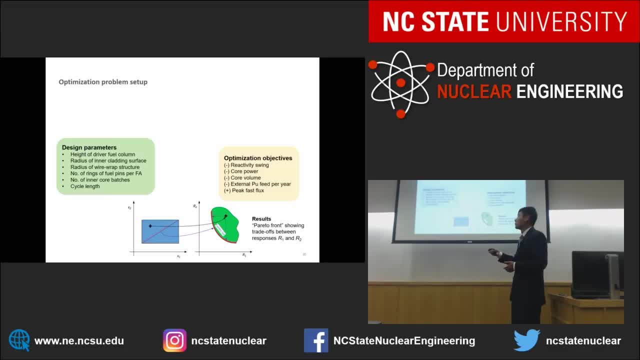 power. does that mean the flux will be lower? well, if the flux is lower, how do lower? well, if the flux is lower, how do lower? well, if the flux is lower, how do you achieve the maximization of your? you achieve the maximization of your. you achieve the maximization of your. peak, fast flux, right? you cannot achieve. 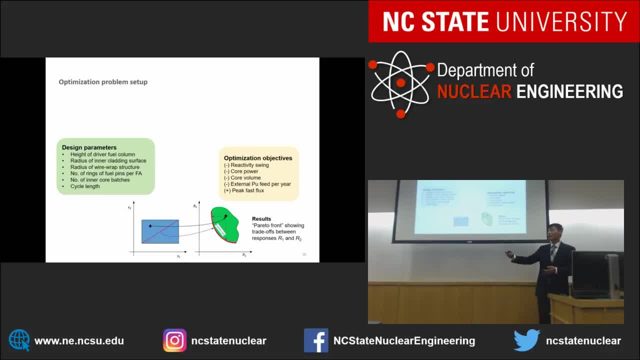 peak fast flux right. you cannot achieve peak fast flux right. you cannot achieve that one go without hurting another, so that one go without hurting another, so that one go without hurting another. so this is where you are if you have only. this is where you are if you have only. 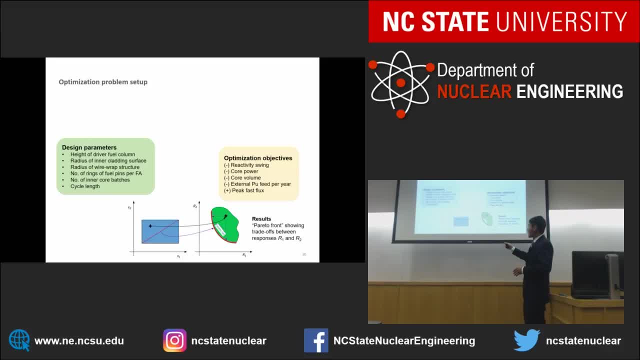 this is where you are. if you have only two objectives- you, you most likely will two objectives. you- you most likely will two objectives you- you most likely will end up the situation that you cannot end up, the situation that you cannot end up, the situation that you cannot improve in one without hurting the other. 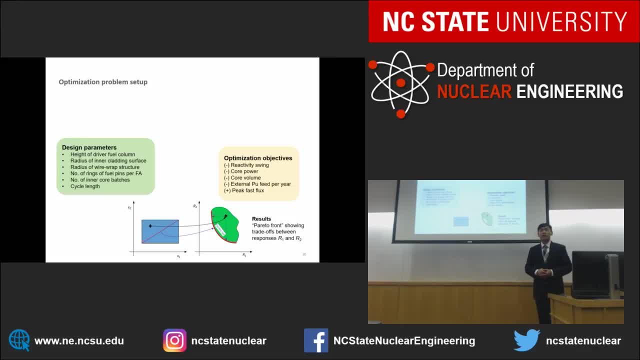 improve in one without hurting the other, improve in one without hurting the other, and on top of that we have also a list, and on top of that we have also a list, and on top of that we have also a list of constraints that we have to consider. 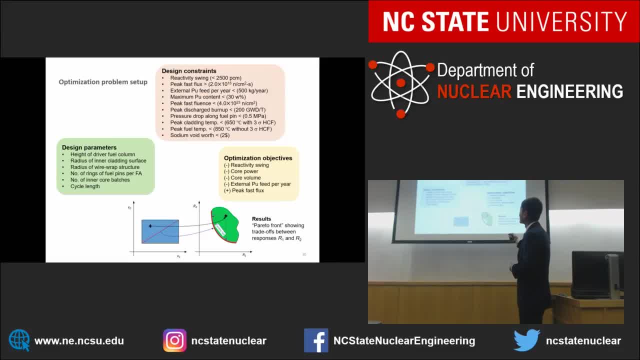 of constraints that we have to consider, of constraints that we have to consider, have them, have them, have them. cladding temperature should not exceed cladding temperature should not exceed cladding temperature. should not exceed certain level peak fuel temperature and certain level peak fuel temperature and certain level peak fuel temperature and sodium void force, which is single most. 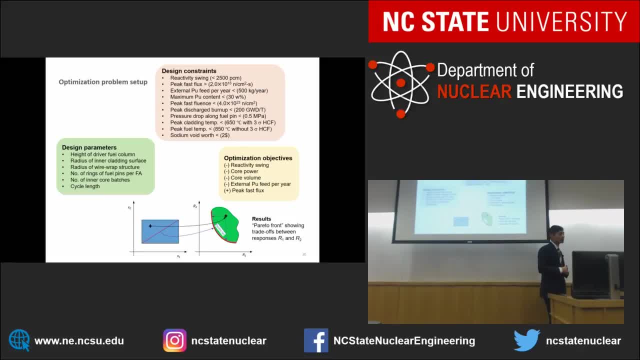 sodium void force, which is single, most sodium void force, which is single, most important. one feedback mechanism in important. one feedback mechanism in important. one feedback mechanism in sodium. could faster reactor, so these are sodium. could faster reactor, so these are sodium. could faster reactor. so these are the constraints, heart limit you should. 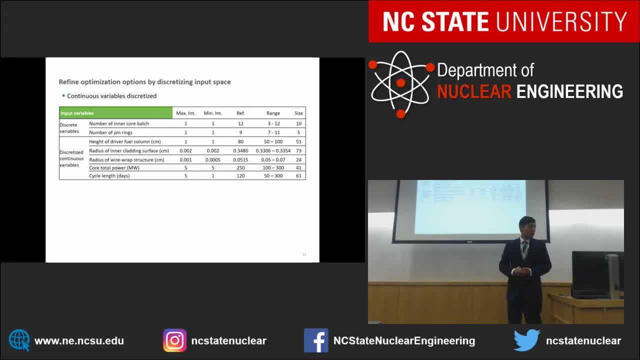 the constraints heart limit. you should. the constraints heart limit. you should never go beyond. and next we look at our never go beyond. and next we look at our never go beyond. and next we look at our input space, input space, input space, the dimension of the fuel assembly, the 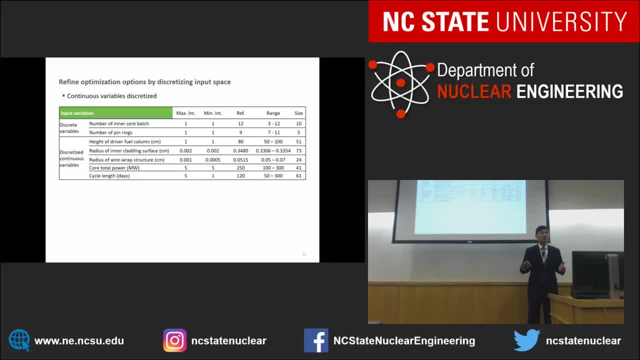 the dimension of the fuel assembly: the the dimension of the fuel assembly, the fuel rods can be changed, but some of fuel rods can be changed. but some of fuel rods can be changed, but some of them are really continuous, I mean number. them are really continuous, I mean number. 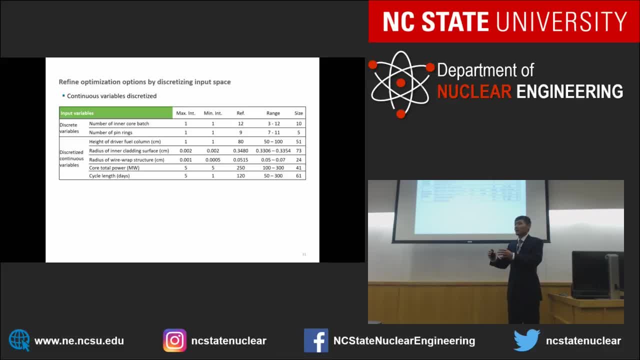 them are really continuous. I mean, number of fuel pins probably are integers, but of fuel pins probably are integers, but of fuel pins probably are integers but dimension or the radius, for example, dimension or the radius, for example, dimension or the radius, for example, radius of the fuel rod, they're continuous. 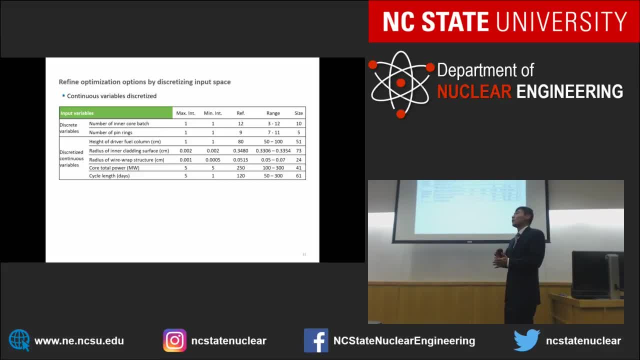 radius of the fuel rod: they're continuous. radius of the fuel rod: they're continuous. it means that we in a certain range are. it means that we in a certain range are. it means that we in a certain range are infinite ways for you to sample those, and 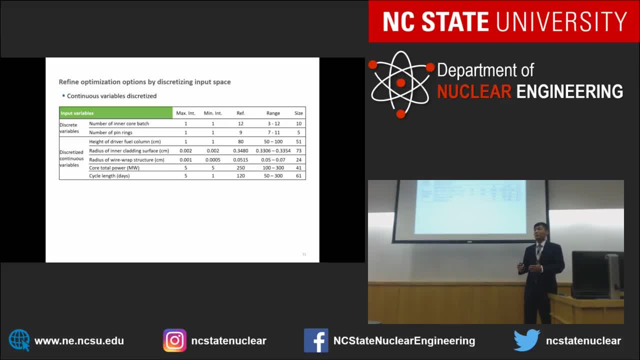 infinite ways for you to sample those and infinite ways for you to sample those and change the design which is not good. change the design which is not good. change the design which is not good. we want to limit the number of choices. we want to limit the number of choices. 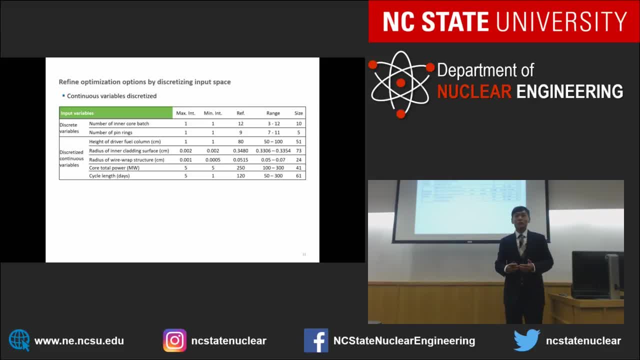 we want to limit the number of choices that we have, so we first discretize that we have. so we first discretize that we have. so we first discretize those input parameters. we define the those input parameters. we define the those input parameters, we define the maximum and minimum interval and give it. 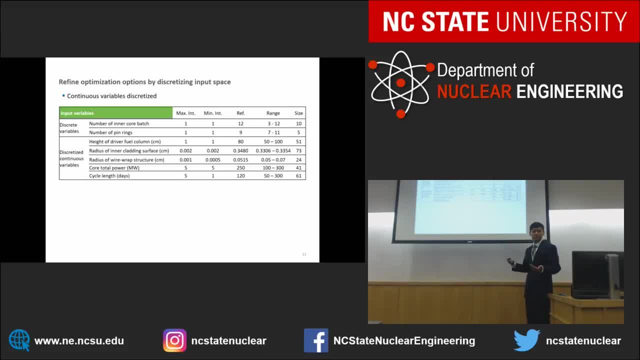 maximum and minimum interval, and give it maximum and minimum interval and give it a range, so we know how many choices we a range. so we know how many choices we a range, so we know how many choices we have. so by taking into consideration of have, so by taking into consideration of: 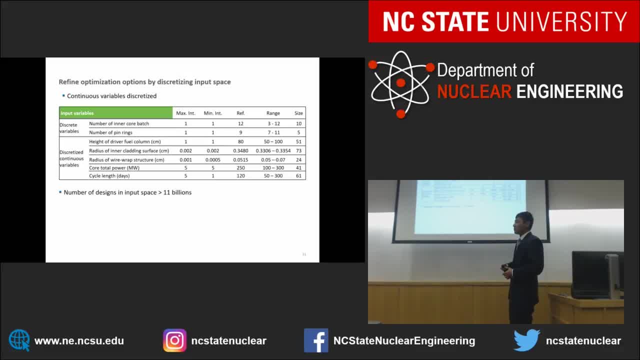 have. so, by taking into consideration of all this, we have more than 11 billion. all this, we have more than 11 billion. all this. we have more than 11 billion possible designs in the input space. I possible designs in the input space, I possible designs in the input space. I don't think you want exhaust all these. 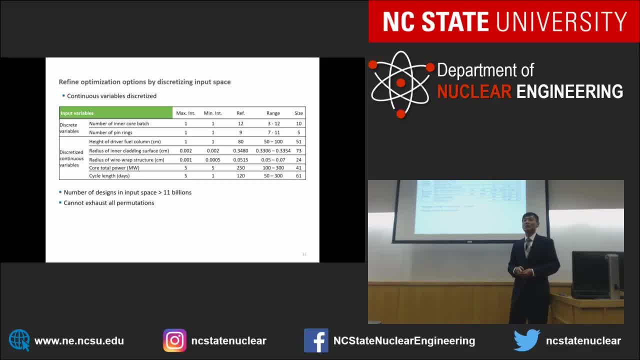 don't think you want exhaust all these, don't think you want exhaust all these permutations to find the best one. so we permutations to find the best one, so we permutations to find the best one. so we really need to have some optimization, really need to have some optimization. 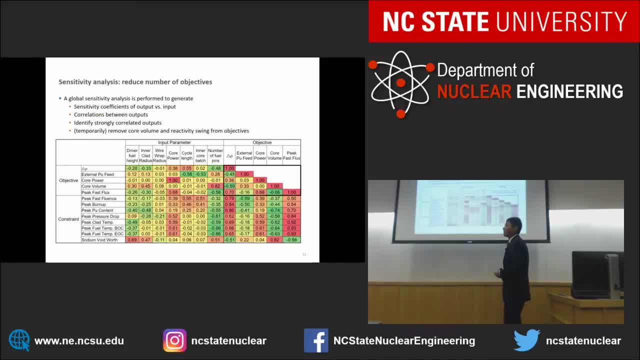 really need to have some optimization algorithm to help us. okay then, in order algorithm to help us. okay then, in order algorithm to help us. okay then, in order to make this problem even more solvable, to make this problem even more solvable, to make this problem even more solvable, we need to see, well, if it possible to. 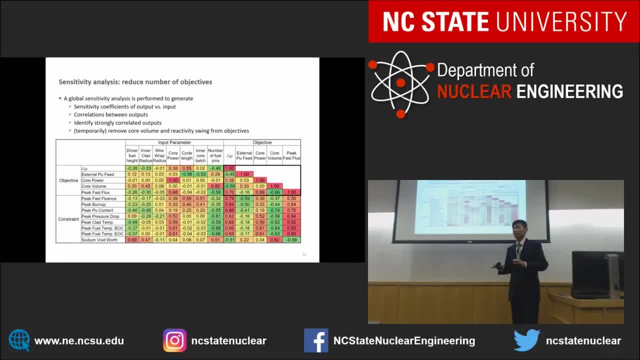 we need to see, well, if it possible to. we need to see, well, if it possible to remove some of the objectives right now. remove some of the objectives right now. remove some of the objectives right now. these are the objectives, so I want to. these are the objectives, so I want to. 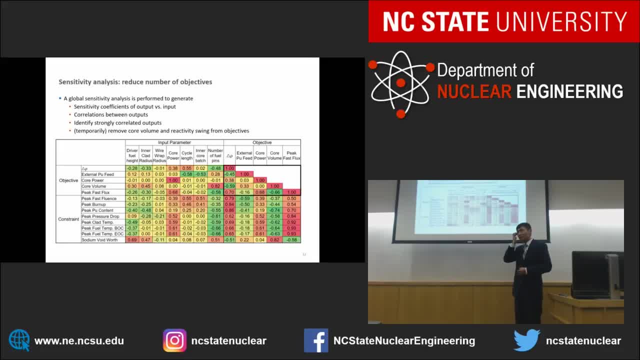 these are the objectives. so I want to see well how many of them are really, see well how many of them are really, see well how many of them are really correlated, if they're really strongly correlated- if they're really strongly correlated- if they're really strongly correlated, I can remove some of them. so 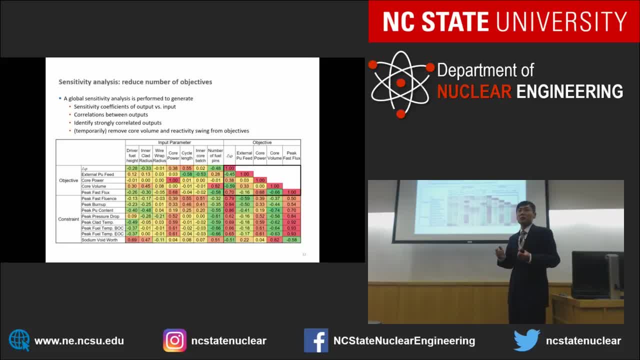 correlated, I can remove some of them. so, correlated, I can remove some of them. so I perform global sensitivity analysis. I. I perform global sensitivity analysis I. I perform global sensitivity analysis. I tweak the input parameters which are tweak the input parameters which are tweak the input parameters which are design parameters and find the 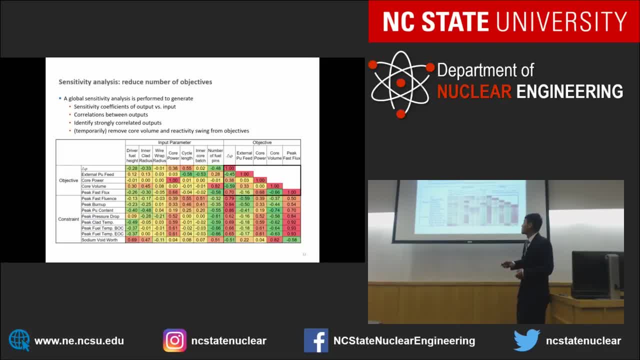 design parameters and find the design parameters and find the correlations of the output parameters. correlations of the output parameters. correlations of the output parameters. okay, this is what we found in the black. okay, this is what we found in the black. okay, this is what we found in the black box. I see that those two parameters- 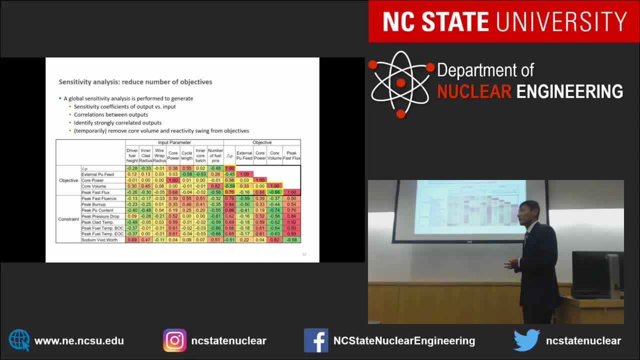 box. I see that those two parameters box. I see that those two parameters for activity swing and reactive correct. for activity swing and reactive correct. for activity swing and reactive correct. core volume are more heavily or strongly core volume are more heavily or strongly. core volume are more heavily or strongly correlated with others. so said okay. 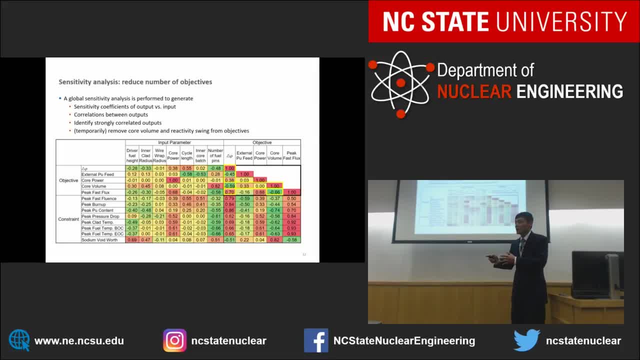 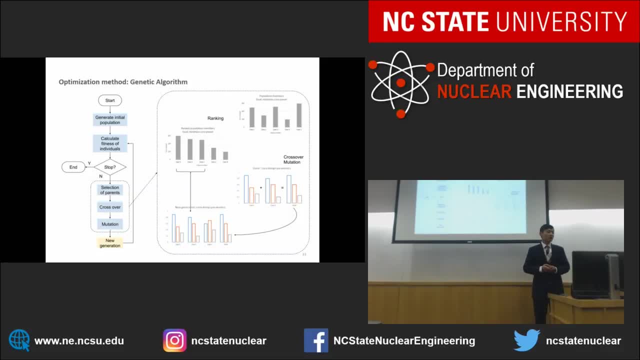 correlated with others, so said okay. correlated with others, so said okay, let's temporarily remove those two and let's temporarily remove those two. and let's temporarily remove those two and simplify our problem, just for at the simplify our problem just for at the. simplify our problem just for at the beginning, what we get. so then we pick. 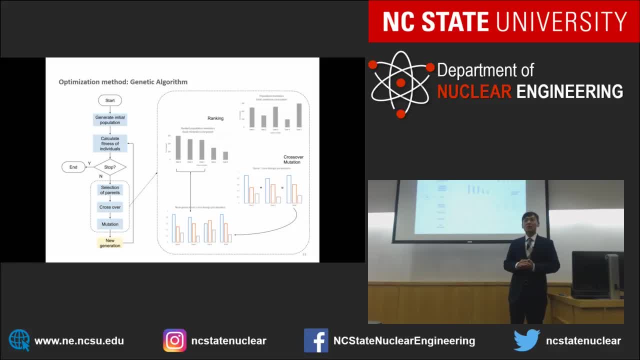 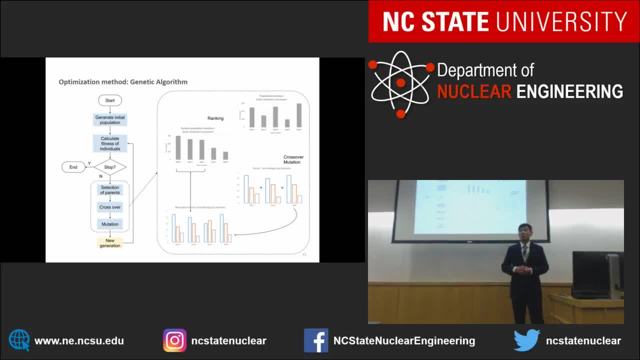 study is called genetic genetic algorithm. you probably ever heard about algorithm. you probably ever heard about algorithm. you probably ever heard about. it is based on the Darwin theory of. it is based on the Darwin theory of. it is based on the Darwin theory of natural selection. the fittest ones will. 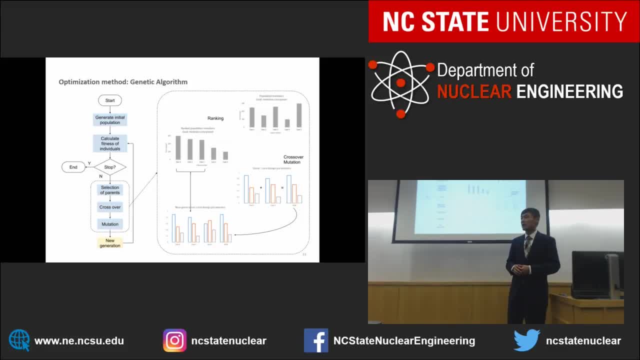 natural selection, the fittest ones will natural selection, the fittest ones will survive- a better chance to survive and survive- a better chance to survive and survive, a better chance to survive. and pass their genetic information to the, pass their genetic information to the, pass their genetic information to the next generation. so this is what we do. we 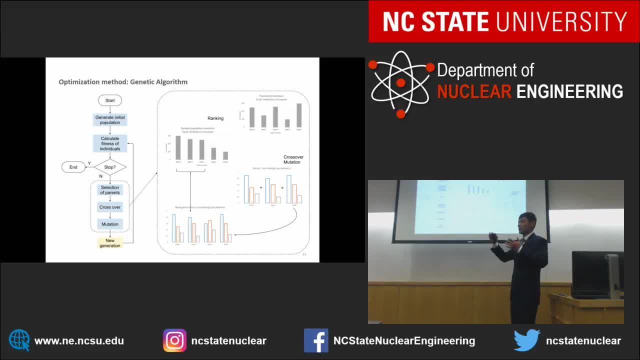 next generation. so this is what we do. we next generation. so this is what we do. we first a. generate the initial population, first a. generate the initial population, first a. generate the initial population. population meaning initial number of population, meaning initial number of population, meaning initial number of designs of the reactor. then we evaluate. 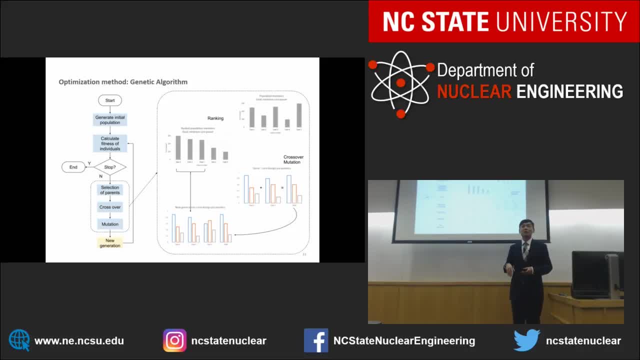 designs of the reactor, then we evaluate designs of the reactor, then we evaluate their performance or their fitness, this their performance or their fitness, this their performance or their fitness. this can be done using the code I just I can be done using the code I just I can be done using the code I just I showed you earlier. then we pick what we. 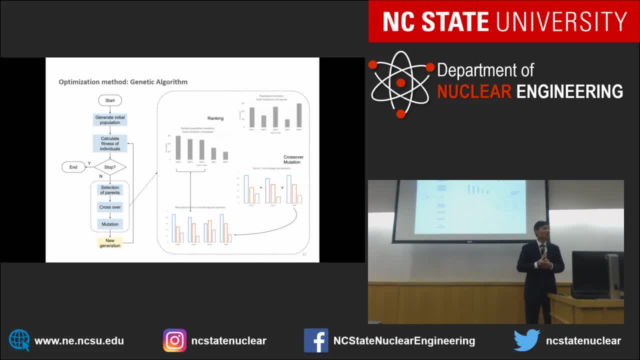 showed you earlier, then we pick what we showed you earlier, then we pick what we want to keep and we want to create from, want to keep and we want to create from, want to keep and we want to create from there. the way example to do this is show. 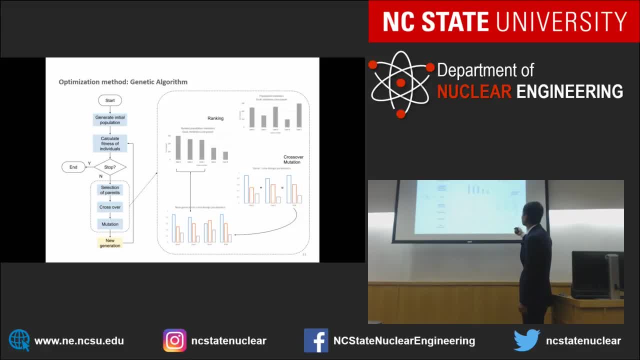 there. the way example to do this is show there. the way example to do this is show on the right first. we rank their on the right first. we rank their on the right first. we rank their performance. supposedly we have those performance. supposedly we have those performance. supposedly we have those members in one generation based on their 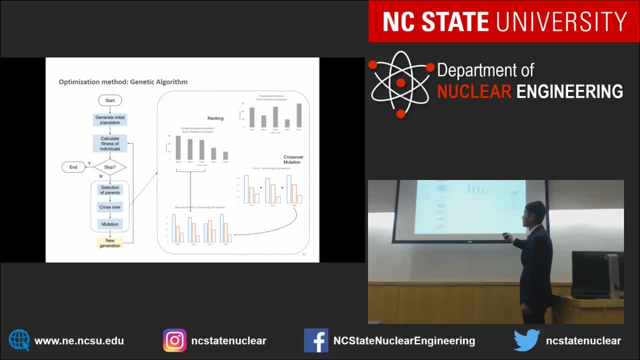 members in one generation, based on their members in one generation. based on their performance. I rank. so now I have case performance. I rank. so now I have case performance. I rank. so now I have case. you probably can read it: case five three. you probably can read it: case five three. 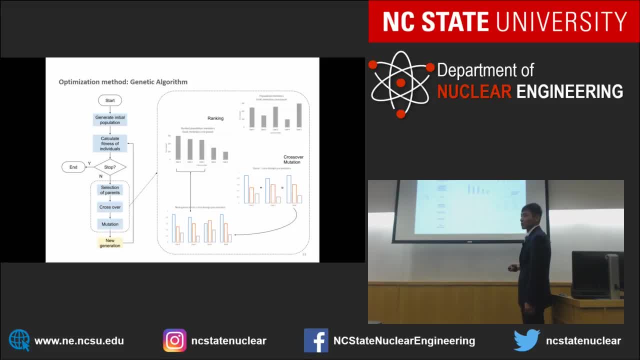 you probably can read it: case five, three and one the top three, one relative of, and one the top three, one relative of, and one the top three, one relative. of course we have much more than five. then course we have much more than five. then course we have much more than five. then we pick those, we directly send those to. 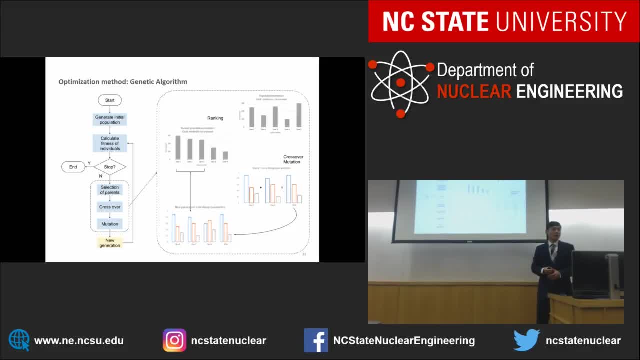 we pick those, we directly send those to. we pick those, we directly send those to the next generation. we say, okay, these, the next generation. we say okay, these, the next generation. we say, okay, these are the promising ones. and then I marry: are the promising ones, and then I marry. 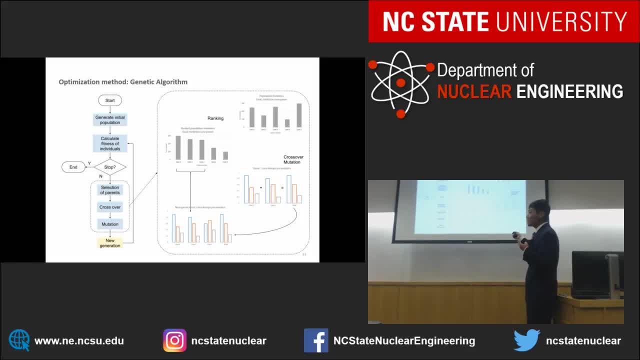 are the promising ones. and then I marry case five and case three by picking case five and case three, by picking case five and case three, by picking their attributes of the design. so these their attributes of the design, so these their attributes of the design. so these are the performance, these are the 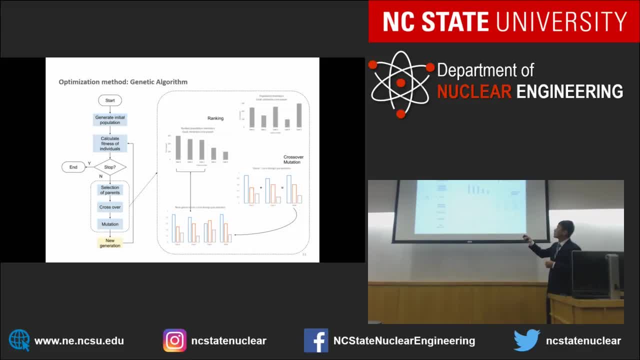 are the performance. these are the are the performance. these are the attributes or design parameters. I pick attributes or design parameters. I pick attributes or design parameters. I pick some from the first case, pick some from some from the first case, pick some from some from the first case, pick some from second case. this is called crossover. 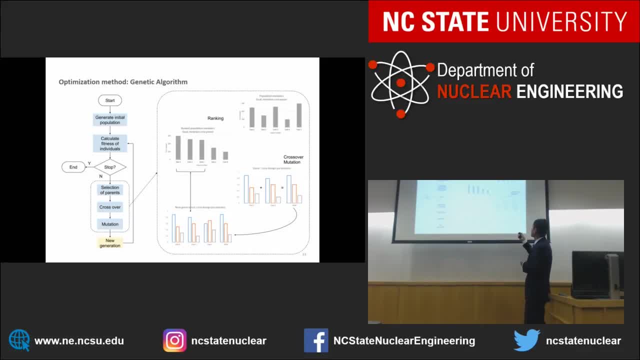 second case: this is called crossover. second case: this is called crossover. then I randomly change some of the. then I randomly change some of the. then I randomly change some of the attributes: this is the child right and I attributes this is the child right and I attributes this is the child right and I change some attributes of in the child. 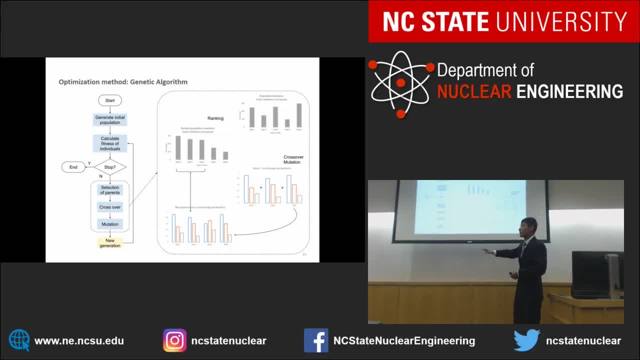 change some attributes of in the child, change some attributes of in the child, and I pass it to the next generation. so, and I pass it to the next generation so, and I pass it to the next generation so I have an another generation, these ones. I have an another generation, these ones. 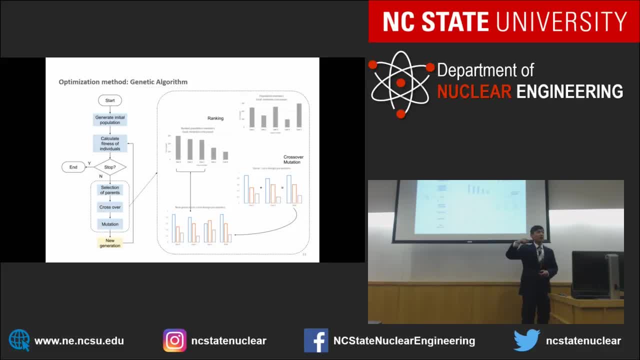 I have an another generation. these ones supposedly work better than the first, supposedly work better than the first, supposedly work better than the first one. then I continue to to evaluate to one, then I continue to to evaluate to one, then I continue to to evaluate, to create a new generation, until I cannot. 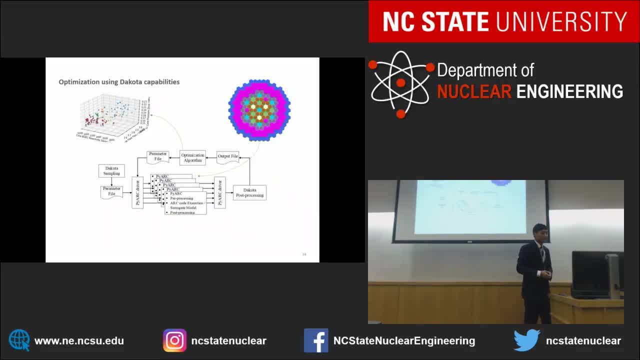 create a new generation. until I cannot create a new generation, until I cannot really improve anymore. so this is the really improve anymore. so this is the really improve anymore. so this is the mechanism that helps us with us, the core mechanism that helps us with us, the core. 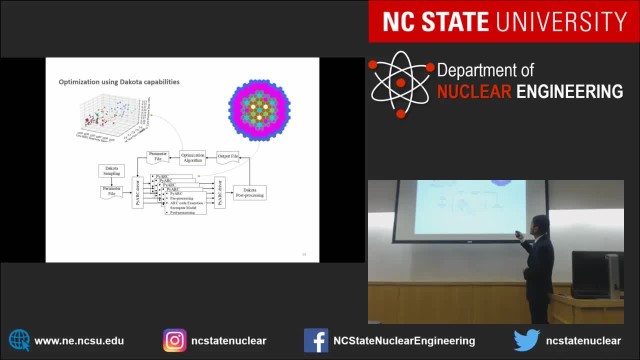 mechanism that helps us with us the core optimization, or sorry. the evaluation optimization, or sorry. the evaluation optimization or sorry. the evaluation will be done using arc argon. develop the will be done using arc argon. develop the will be done using arc argon. develop the code. the optimization algorithm will. 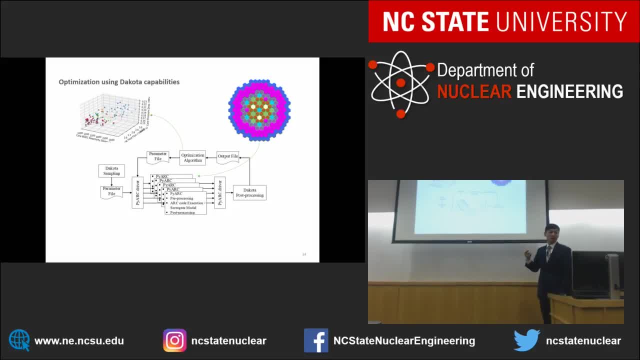 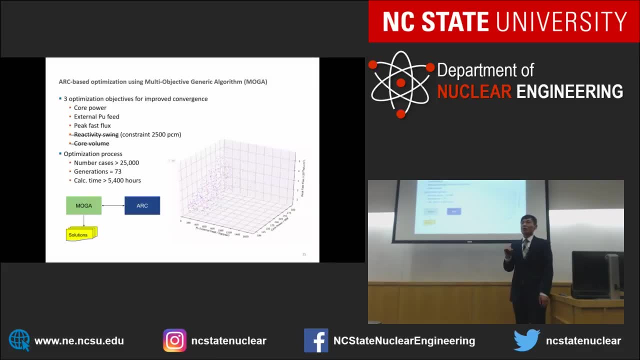 code. the optimization algorithm will code. the optimization algorithm will coming from Dakota. code which is designed coming from Dakota. code which is designed coming from Dakota. code which is designed or developed by Sandia National or developed by Sandia National or developed by Sandia National. so the first thing we did is that let's 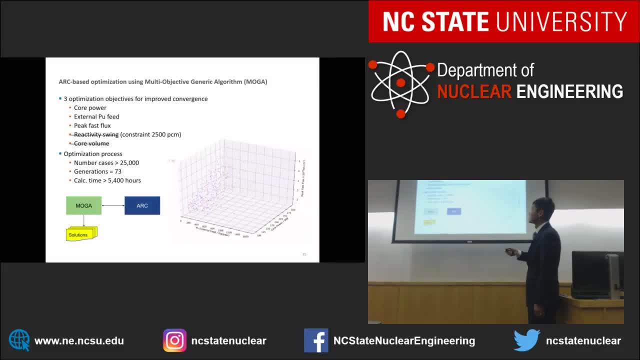 so the first thing we did is that let's. so the first thing we did is that let's stay with the three objectives. a core stay with the three objectives. a core stay with the three objectives. a core: power- external plutonium feed and peak power- external plutonium feed and peak. power, external plutonium feed and peak fast flux. we want to maximize or want to fast flux. we want to maximize or want to fast flux. we want to maximize or want to minimize the first two want to maximize, minimize the first two. want to maximize. minimize the first two. want to maximize the third one. we remove temporarily the. 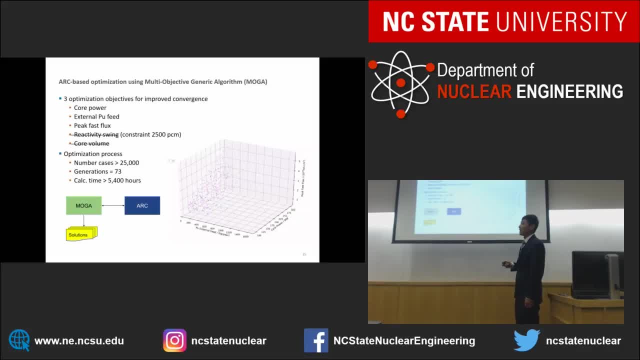 the third one: we remove temporarily the. the third one: we remove temporarily the reactivity swing. we just put a hard reactivity swing. we just put a hard reactivity swing. we just put a hard limit- 2500 PCM- and we remove the core limit- 2500 PCM- and we remove the core. 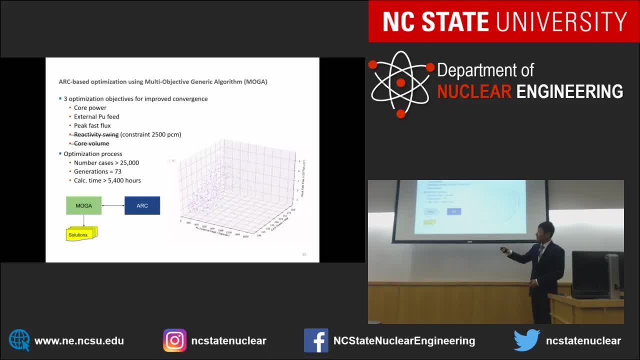 limit, 2500 PCM, and we remove the core volume and we do the multi object volume and we do the multi object volume and we do the multi object objective genetic algorithm- MOGA objective genetic algorithm. MOGA objective genetic algorithm, MOGA calculation. the evaluation again is done. 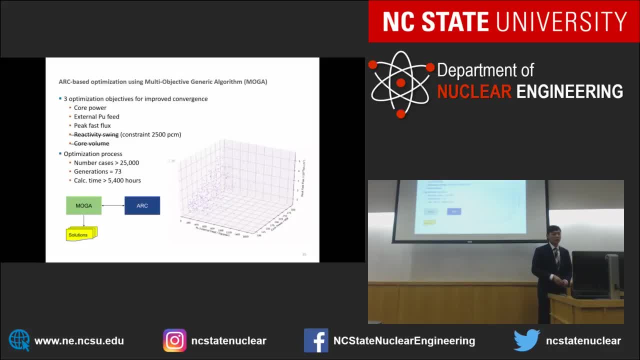 calculation: the evaluation again is done. calculation: the evaluation again is done by arc. in the end we hope we'll find a by arc in the end. we hope we'll find a by arc in the end. we hope we'll find a bunch of near optimal solutions. so this: 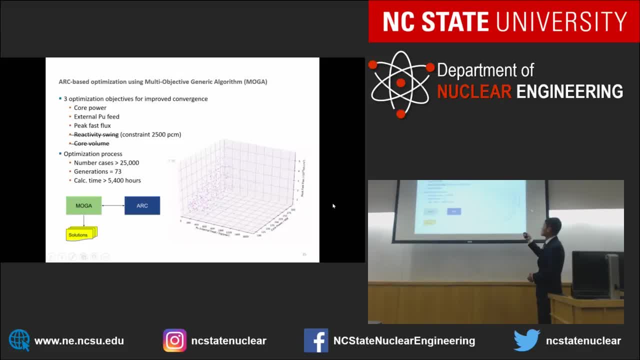 bunch of near optimal solutions. so this bunch of near optimal solutions. so this is how it looks like the three axis. here is how it looks like the three axis. here is how it looks like. the three axis here shows the three objectives: plutonium. shows the three objectives- plutonium. 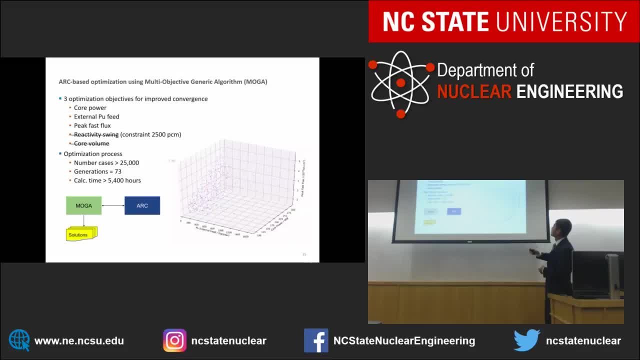 shows the three objectives: plutonium feed- cool power and fast flux. peak fast feed- cool power and fast flux. peak fast feed- cool power and fast flux- peak fast flux. I start my first generation okay, as flux. I start my first generation okay, as flux. I start my first generation okay, as you see more dots coming, then it means 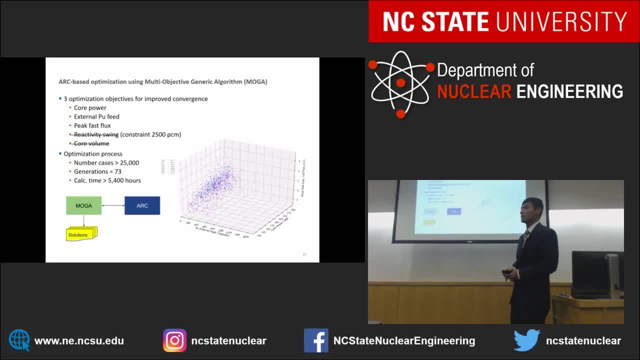 you see more dots coming, then it means you see more dots coming, then it means more generation is coming be created. more generation is coming be created. more generation is coming be created. join this design space and you can see. join this design space and you can see. join this design space and you can see different colors start to show and this: 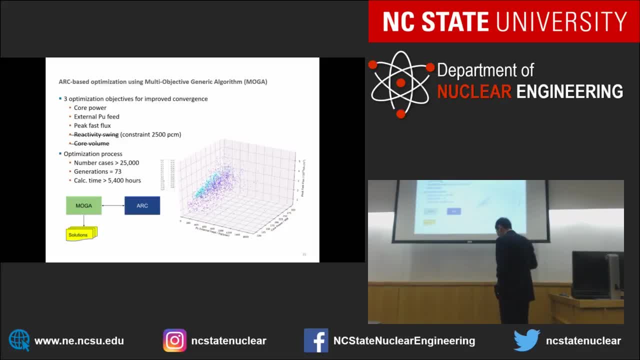 different colors start to show and this different colors start to show and this shows more generation is going on and shows more generation is going on and shows more generation is going on. and getting you see lava dots in this area. getting you see lava dots in this area. 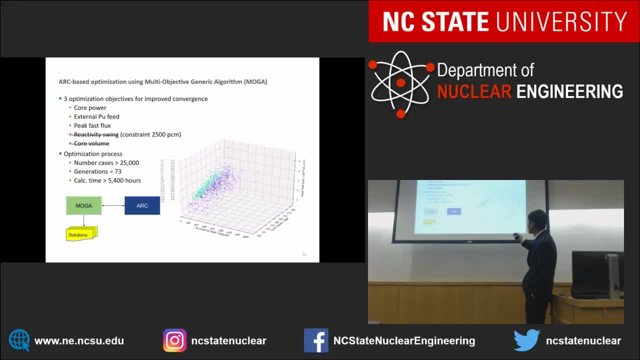 getting. you see lava dots in this area, but really this is the direction we're, but really this is the direction we're. but really this is the direction we're going to, because we're going to minimize, going to, because we're going to minimize, going to, because we're going to minimize the core or plutonium feed. we're going. 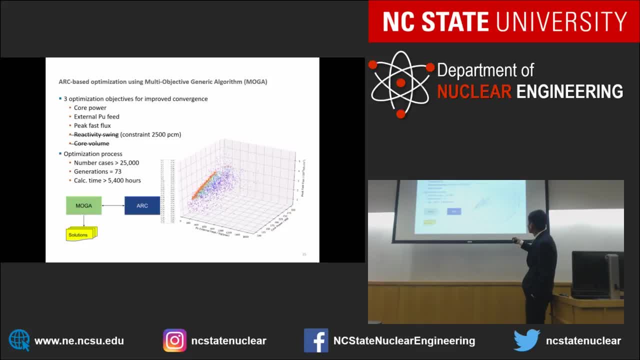 the core or plutonium feed. we're going the core or plutonium feed. we're going to minimize the core power. we're going to minimize the core power. we're going to minimize the core power. we're going to maximize the peak fast flux, so you should be able to see some front. it's. 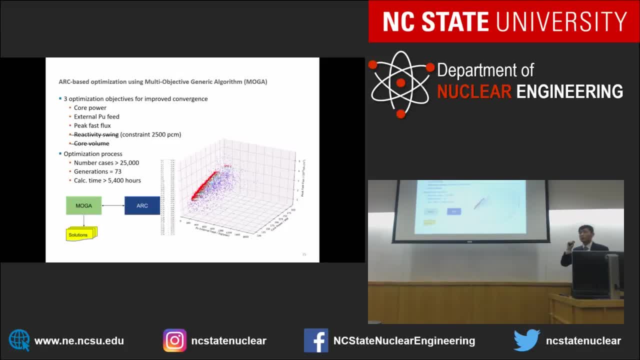 should be able to see some front. it's should be able to see some front. it's called Pareto front, where you can pick, called Pareto front, where you can pick, called Pareto front, where you can pick your best performing designs. okay so, your best performing designs, okay so. 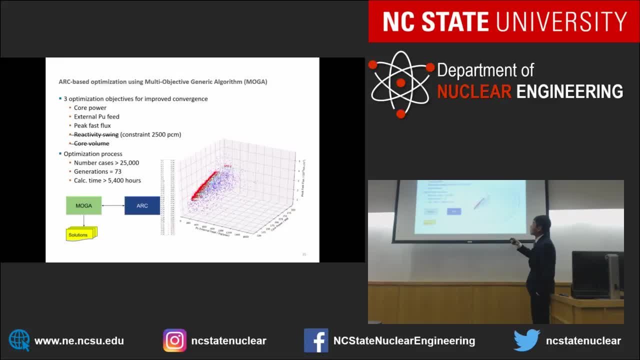 your best performing designs okay. so after 73 generations, we're able to get after 73 generations, we're able to get after 73 generations, we're able to get this Pareto front. okay at the beginning. this Pareto front okay at the beginning, this Pareto front- okay at the beginning. see all of dots in this area, but really, 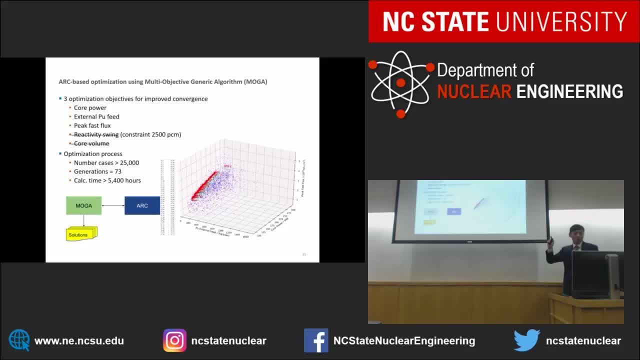 see all of dots in this area, but really see all of dots in this area, but really they're useless because they're not this. they're useless because they're not this. they're useless because they're not. this is not where the direction that we want is not where the direction that we want. 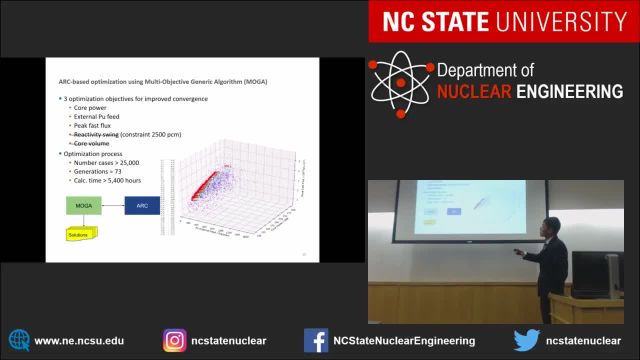 is not where the direction that we want. but more and more you see the dots, but more and more you see the dots, but more and more you see the dots coming in this line, okay, and in this coming in this line, okay, and in this coming in this line, okay. and in this whole process we evaluated more than 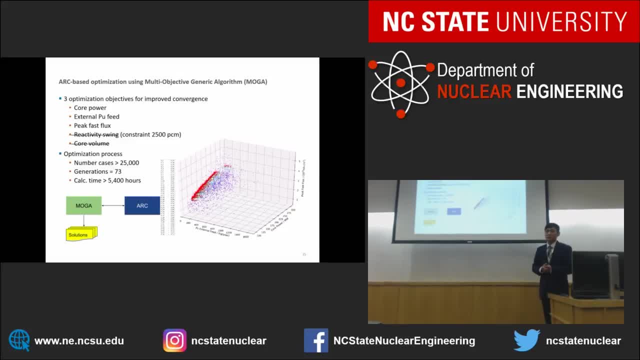 whole process. we evaluated more than whole process. we evaluated more than about 25,000 cases. okay, because each about 25,000 cases. okay, because each about 25,000 cases. okay, because each case takes about 13 minutes in total. we case takes about 13 minutes in total. we. 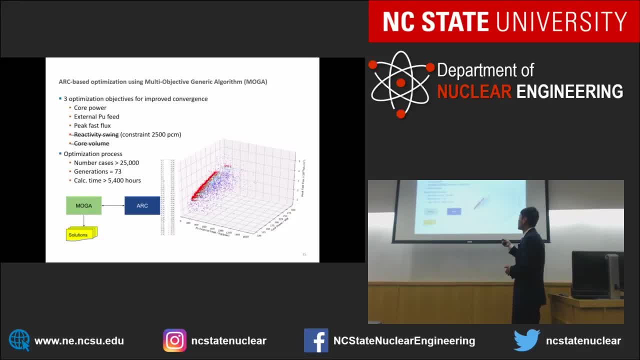 case takes about 13 minutes in total. we spend more than 5,000 hours to find the. spend more than 5,000 hours to find the. spend more than 5,000 hours to find the best solution. okay, so how? the? how do the? 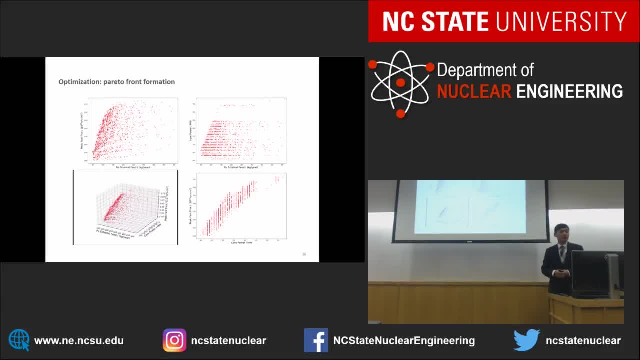 best solution. okay, so how the how do the best solution? okay, so how the how do the performance? look like: this is again the performance. look like this is again the performance. look like: this is again the Pareto front formation. I pick any two of Pareto front formation. I pick any two of: 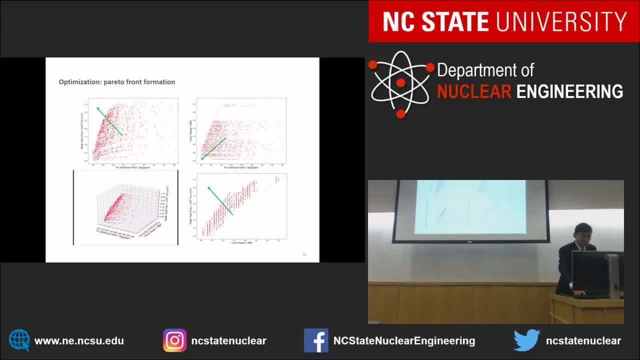 Pareto front formation. I pick any two of them and create a map. I want to reach them and create a map. I want to reach them and create a map. I want to reach into these location directions. okay for into these location directions. okay for into these location directions. okay, for example, minimizing the plutonium feed. 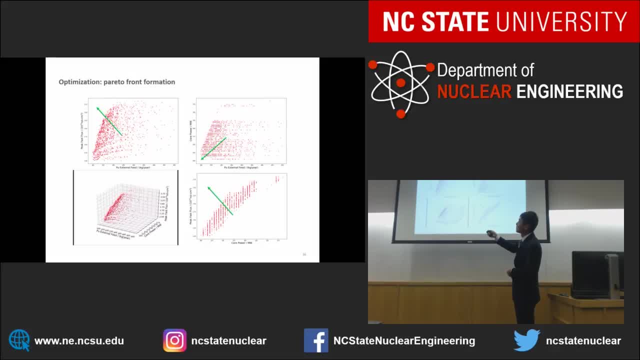 example, minimizing the plutonium feed. example: minimizing the plutonium feed while maximizing the peak fast flux. so, while maximizing the peak fast flux, so, while maximizing the peak fast flux. so this is the direction I'm going. I'm this is the direction I'm going. I'm. 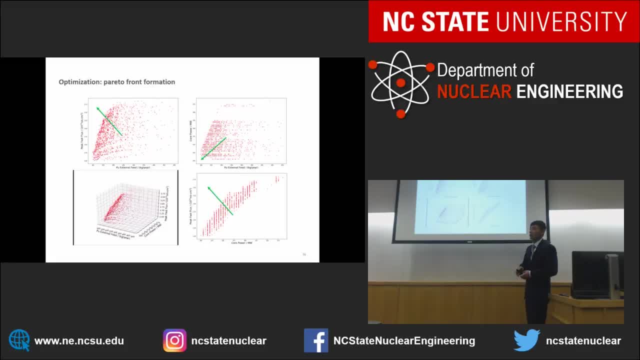 this is the direction I'm going. I'm going to pick some design in this, in this, going to pick some design in this, in this, going to pick some design in this, in this location, and the same for the others location, and the same for the others location and the same for the others. this is just a 3d visualization of the. 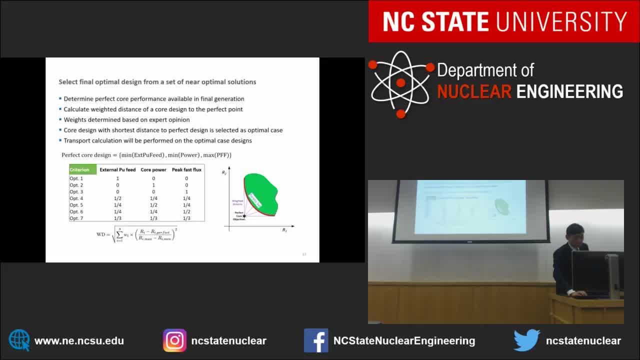 this is just a 3d visualization of the. this is just a 3d visualization of the Pareto front. so, among all this near Pareto front, so among all this near Pareto front, so among all this near optimal designs, how do I pick the best? 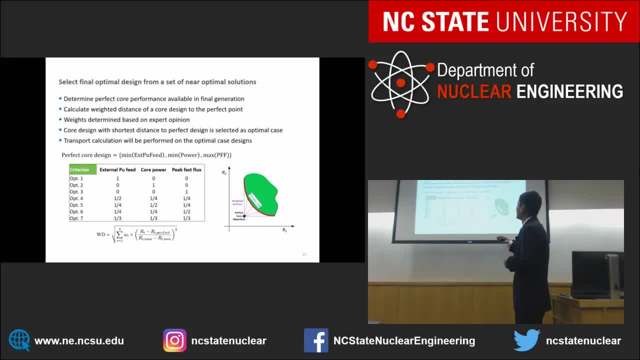 optimal designs. how do I pick the best optimal designs? how do I pick the best ones, or the one? I need the different ones, or the one I need the different ones, or the one I need the different ways because you're going to pick along ways, because you're going to pick along. 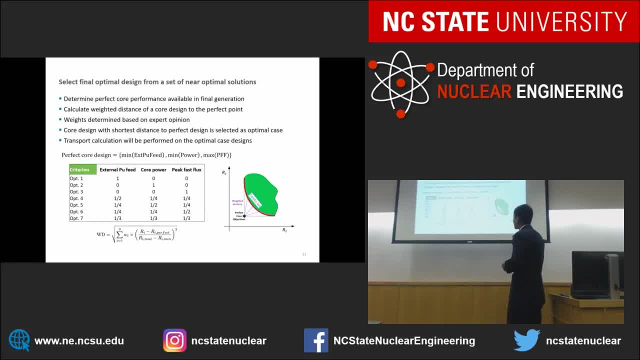 ways, because you're going to pick along this red curve Pareto front. it really this red curve Pareto front. it really this red curve Pareto front? it really depends if you have only two, depends if you have only two, depends if you have only two parameters or objectives and you think 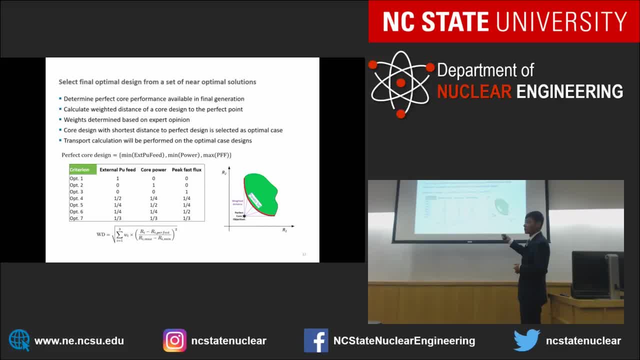 parameters or objectives, and you think parameters or objectives, and you think r1 is more important than r2. you, r1 is more important than r2. you, r1 is more important than r2. you, probably, you probably want to minimize, probably, you probably want to minimize. 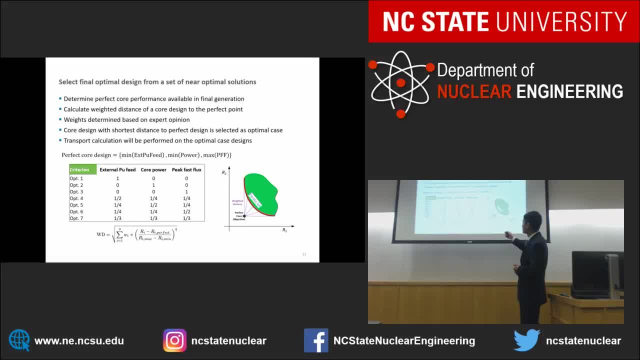 probably. you probably want to minimize r1 more than r2, so you should go this r1 more than r2. so you should go this r1 more than r2, so you should go this. region if r2 minimizing r2 is more. region if r2 minimizing r2 is more. 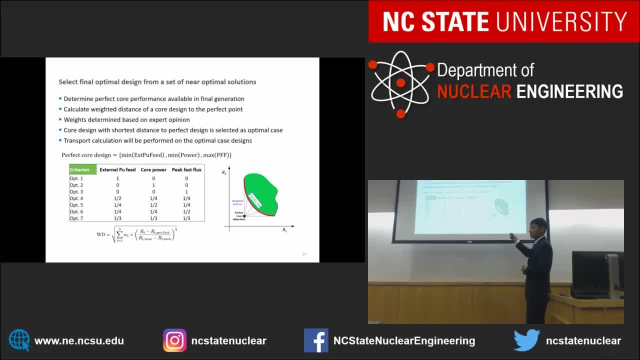 region. if r2- minimizing r2- is more important than minimizing r1, you important than minimizing r1, you important than minimizing r1, you probably should go to this region. so it probably should go to this region. so it probably should go to this region. so it means that you, when you, you can assign. 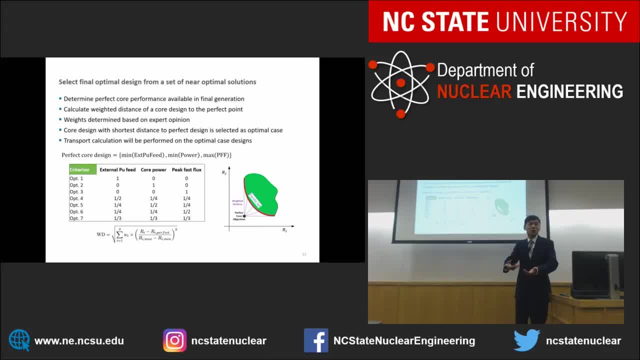 means that you, when you, you can assign, means that you, when you, you can assign different weight to different objectives. different weight to different objectives, different weight to different objectives. you can assign all your weights to one. you can assign all your weights to one. you can assign all your weights to one of the objects or you can evenly. 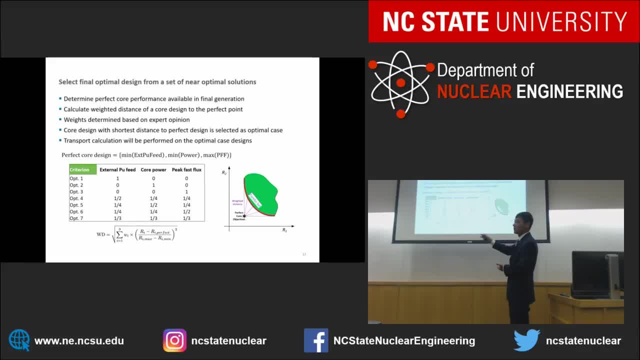 of the objects, or you can evenly of the objects, or you can evenly distribute the weights, or you can do distribute the weights, or you can do distribute the weights, or you can do something in between 50 in 1 and 25, and something in between 50 in 1 and 25, and 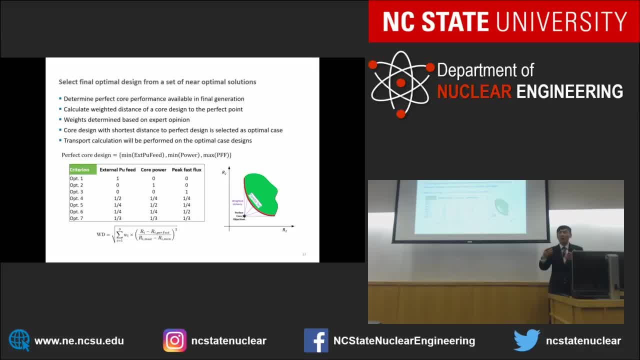 something in between 50 in 1 and 25 and 25 in the other two. so you have seven, 25 in the other two. so you have seven, 25 in the other two. so you have seven options. here I mean you have infinite options. here I mean you have infinite. 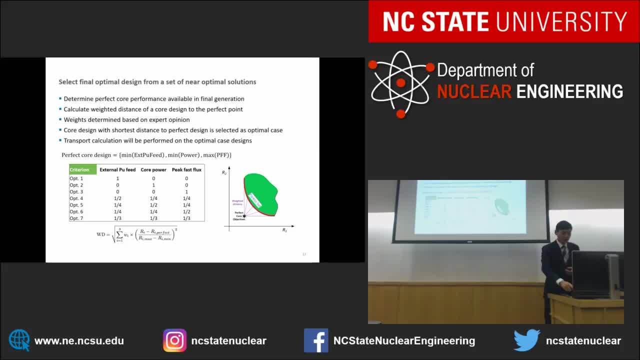 options here. I mean, you have infinite options. we just tried this seven to see options. we just tried this seven to see options. we just tried this seven to see how it have impact on our choice. so how it have impact on our choice, so how it have impact on our choice. so these are the performance of these seven. 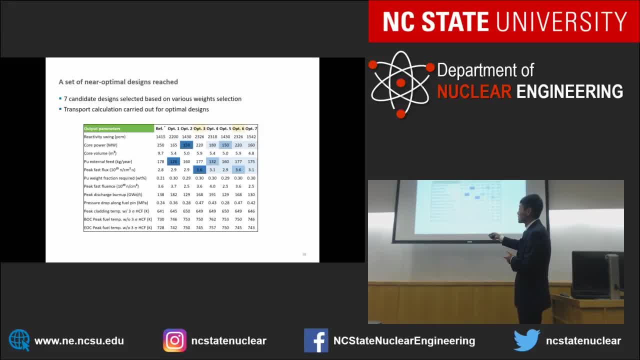 these are the performance of these seven. these are the performance of these seven options in addition to the reference options, in addition to the reference options, in addition to the reference case. or the reference is the argon case, or the reference is the argon case, or the reference is the argon design from many years ago. we want to 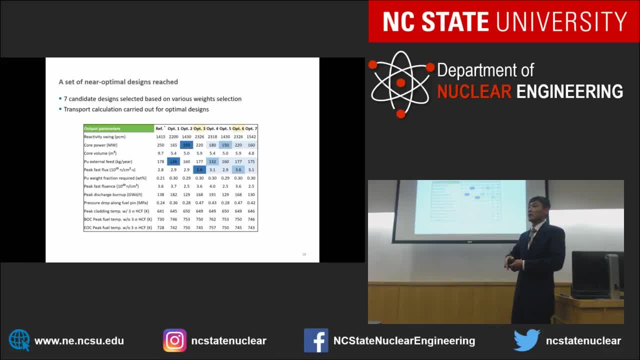 design from many years ago. we want to design from many years ago. we want to see if our new design can outperform, see if our new design can outperform, see if our new design can outperform their reference design. if I compare all their reference design, if I compare all. 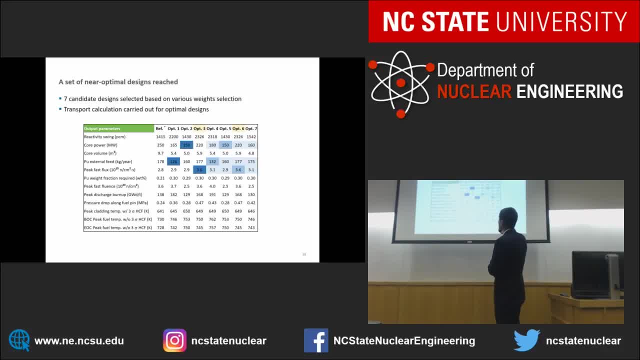 their reference design. if I compare all this numbers in this region- okay, I see this numbers in this region. okay, I see this numbers in this region- okay, I see, yeah, all this one we're able to minimize. yeah, all this one we're able to minimize. yeah, all this one we're able to minimize. or- let's leave that for a moment- reduce. 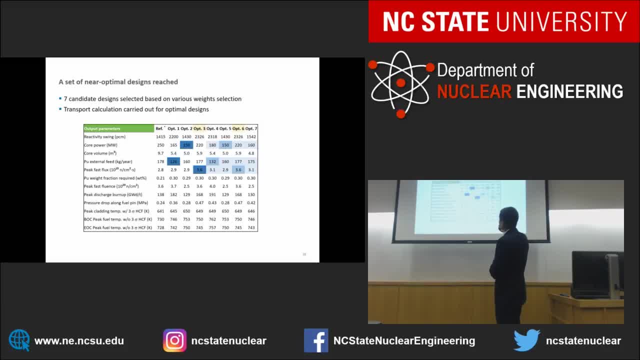 or let's leave that for a moment. reduce or let's leave that for a moment. reduce the core power. reduce the core volume, the core power. reduce the core volume, the core power. reduce the core volume. minimize the plutonium feed and minimize the plutonium feed. and. 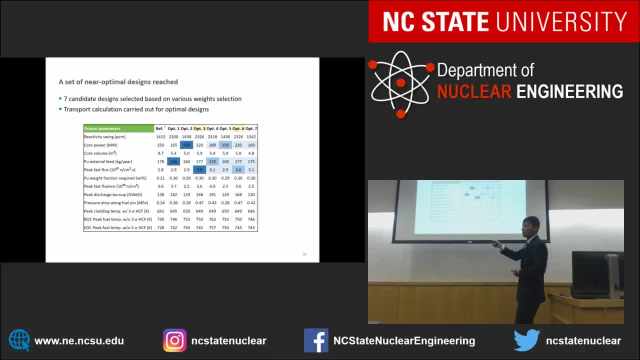 minimize the plutonium feed and increasing or promoting the fast flux. we increasing or promoting the fast flux. we increasing or promoting the fast flux. we achieved our goal and the one for the achieved our goal and the one for the achieved our goal and the one for the rectific swing, even though some of them. 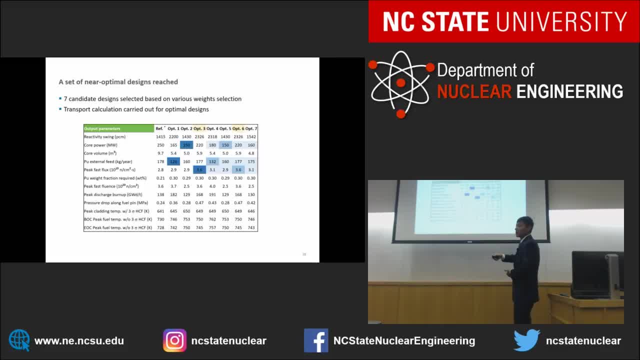 rectific swing. even though some of them rectific swing, even though some of them are not as good as this one, we're still are not as good as this one. we're still are not as good as this one. we're still under the limit: 2,500 PCM and number. 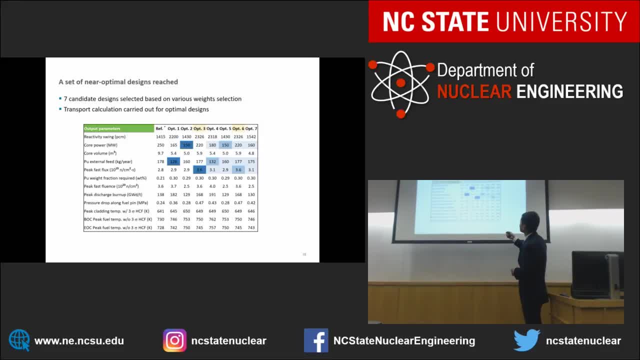 under the limit 2,500 PCM and number under the limit 2,500 PCM. and number three and number six: they are exact: the three and number six. they are exact: the three and number six. they are exact, the same design, even though different. same design even though different. 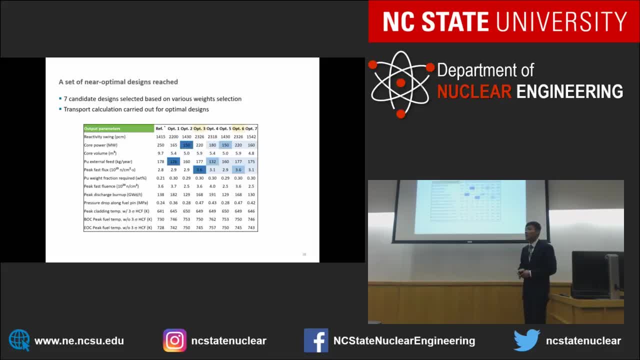 same design, even though different weights have been applied to the three. weights have been applied to the three. weights have been applied to the three. it probably means peak fast flux. is it probably means peak fast flux? is it probably means peak fast flux is really difficult to to maximize, so 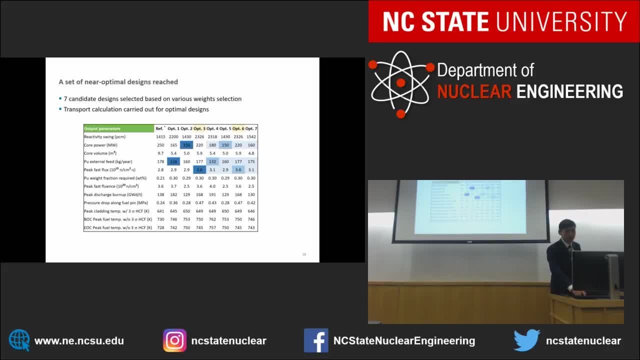 really difficult to to maximize, so really difficult to to maximize. so that's why, even when you apply different, that's why, even when you apply different, that's why, even when you apply different weights, you still end up with the same weights. you still end up with the same. 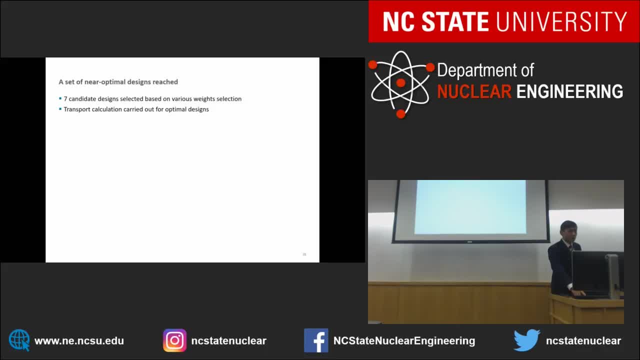 weights, you still end up with the same design. so this is another way to look at design. so this is another way to look at design. so this is another way to look at the performance. I plot the optimal value, the performance. I plot the optimal value, the performance. I plot the optimal value versus the reference value. if I'm going 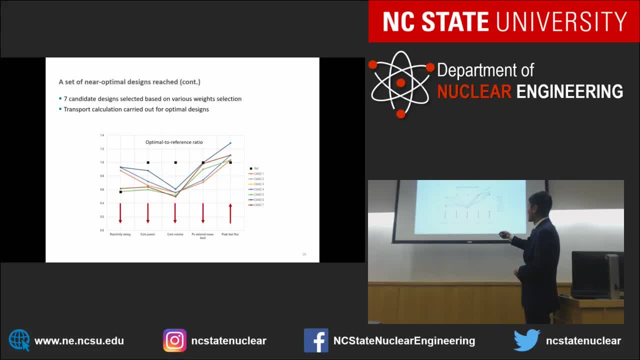 versus the reference value. if I'm going versus the reference value, if I'm going to minimize those, I want to see my the to minimize those. I want to see my the to minimize those. I want to see my the color dots below the black square. which color dots below the black square? which? 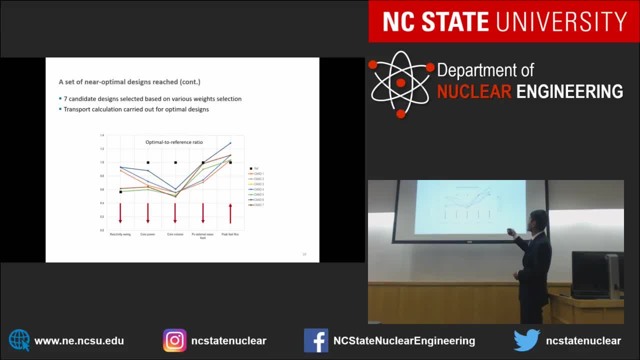 color dots below the black square, which is reference. if I'm going to maximize is reference. if I'm going to maximize is reference. if I'm going to maximize them, I want to see them above the black them. I want to see them above the black them, I want to see them above the black square. and they are, except for this one. 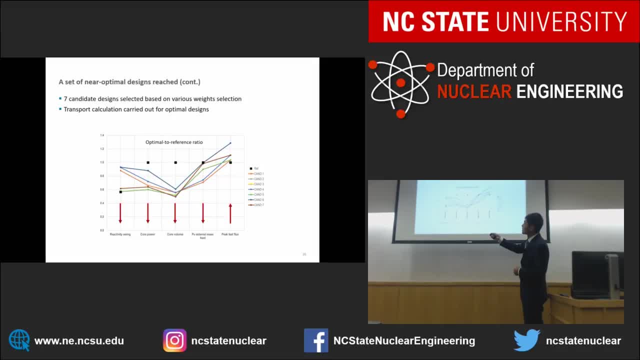 square, and they are except for this one square, and they are except for this one, but again one in this reactivity swing, but again one in this reactivity swing, but again one in this reactivity swing means it's is the bound, upper bound: 2500. 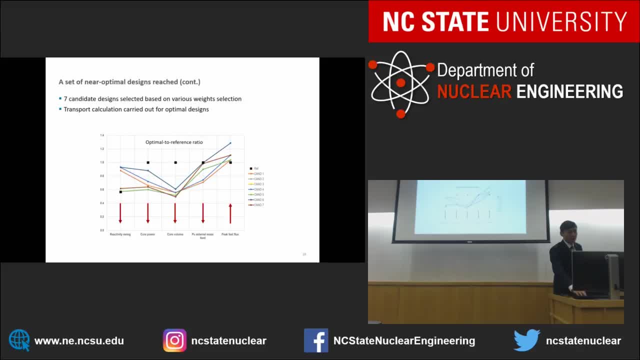 means it's: is the bound upper bound: 2500 means it's: is the bound upper bound: 2500 PCM. we're still below it, so we're okay, PCM. we're still below it, so we're okay, PCM. we're still below it, so we're okay. and again, the issue with this is that 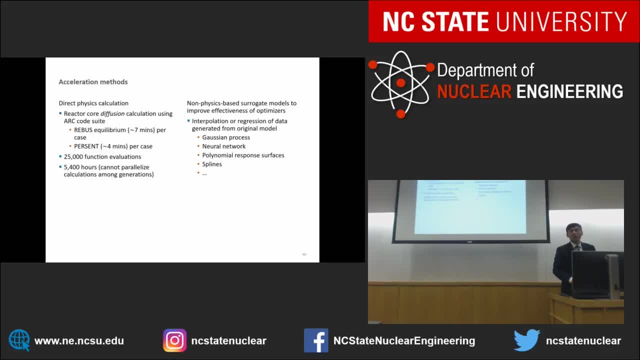 and again. the issue with this is that, and again, the issue with this is that it's really slow, more than 5,000 hours. it's really slow, more than 5,000 hours. it's really slow, more than 5,000 hours. still now we're thinking if we can. 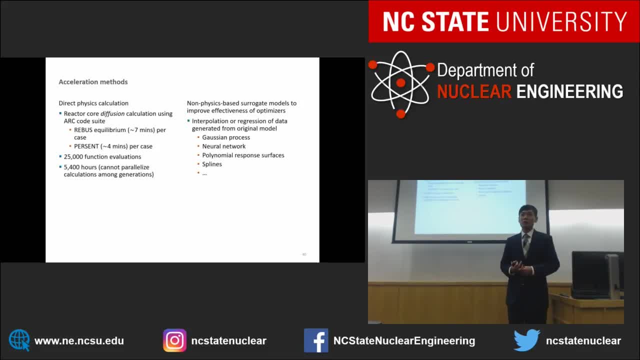 still now we're thinking, if we can. still now we're thinking if we can, replace the arc which is physics based, replace the arc which is physics based. replace the arc which is physics based calculation with some non physics based calculation with some non physics based calculation with some non physics based. a circuit model: I have different. 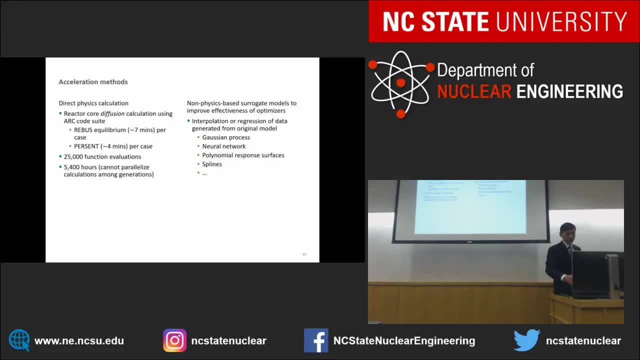 a circuit model. I have different a circuit model, I have different choices here. and if also we want to choices here and if also we want to choices here and if also we want to think if we can even try some hybrid, think if we can even try some hybrid, 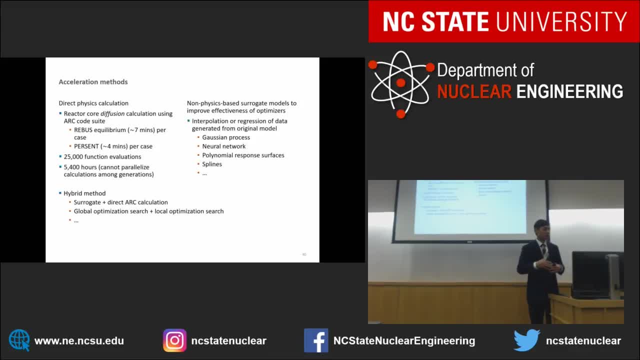 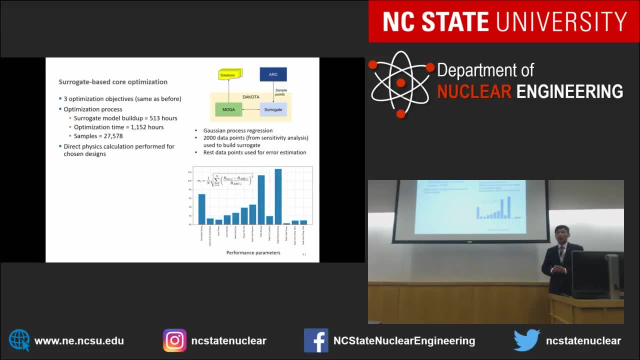 think if we can even try some hybrid breed method, combine the circuit with breed method, combine the circuit with breed method, combine the circuit with the direct physics based calculation. so the direct physics based calculation, so the direct physics based calculation. so that's what we tried. next I pick: we 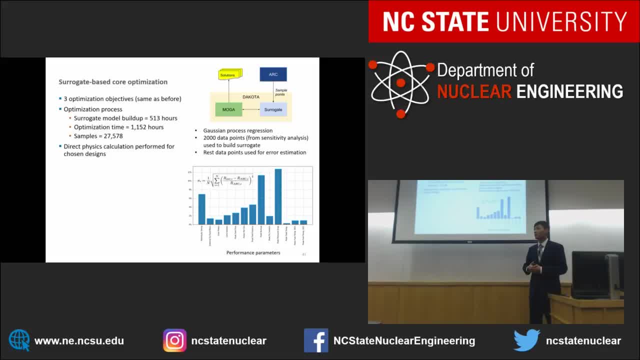 that's what we tried next, I pick we. that's what we tried next, I pick we. pick the Gaussian process regression as pick the Gaussian process regression as pick the Gaussian process regression as the circuit model. I used data sets- the circuit model. I used data sets- the circuit model. I used data sets generated from the arc calculation to 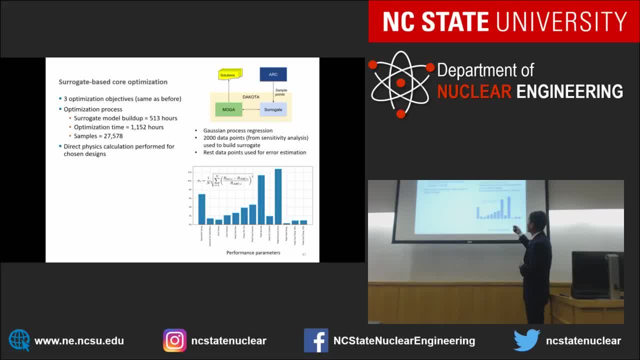 generated from the arc calculation to generated from the arc calculation to train my surrogate, and then I compare train my surrogate and then I compare train my surrogate and then I compare the performance of circuit versus arc, the performance of circuit versus arc, the performance of circuit versus arc. this is a relative error of the core. 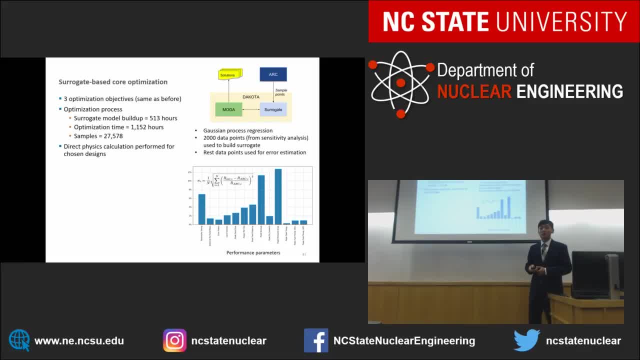 this is a relative error of the core. this is a relative error of the core performance. many of them are below 5% performance. many of them are below 5% performance. many of them are below 5%. only two of them are beyond 10%. okay so, 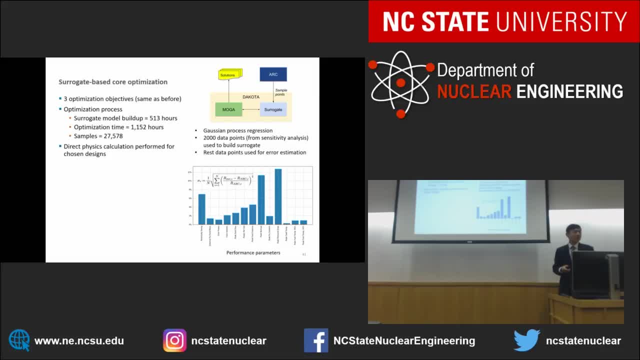 only two of them are beyond 10%. okay, so only two of them are beyond 10%. okay, so I consider that acceptable. then this: I consider that acceptable. then this: I consider that acceptable. then this process takes about 500 hours training process takes about 500 hours training. 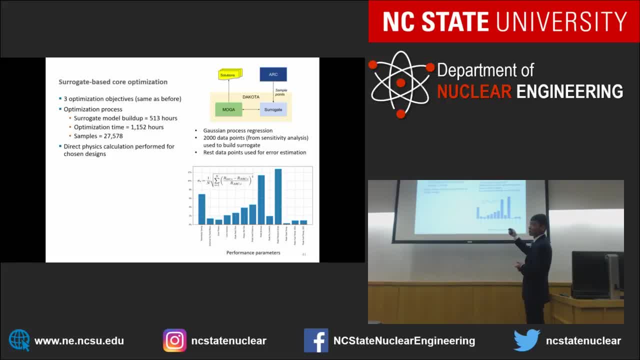 process takes about 500 hours: training the circuit, then I use the circuit to do the circuit, then I use the circuit to do the circuit, then I use the circuit to do the optimization takes about 1100 hours. the optimization takes about 1100 hours. the optimization takes about 1100 hours. in total, we're talking 1600 hours- much. 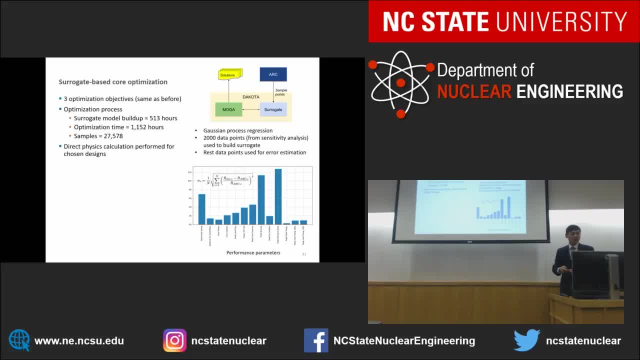 in total, we're talking 1600 hours, much in total. we're talking 1600 hours, much better than 500. you know 5,000 hours better than 500. you know 5,000 hours better than 500. you know 5,000 hours. then I'm checking the performance. they. 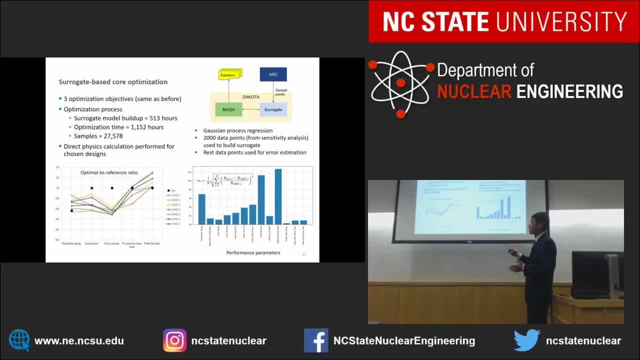 then I'm checking the performance. they then I'm checking the performance. they look just fine without too much detailed. look just fine without too much detailed. look just fine without too much detailed. comparison, except so what should be comparison? except so what should be comparison? except so what should be below. they're below which should be above. 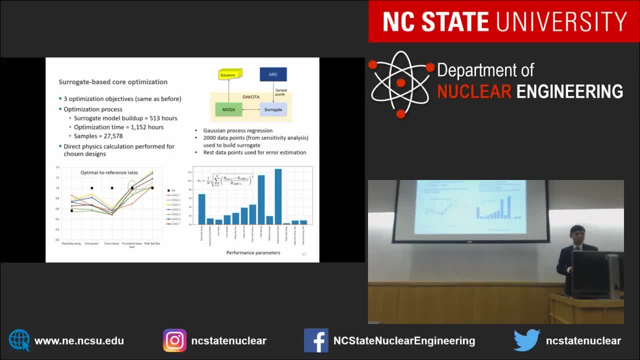 below they're below, which should be above. below they're below, which should be above or above, and except for a couple of or above, and except for a couple of or above, and except for a couple of cases, here they should be below, but cases, here they should be below. but. 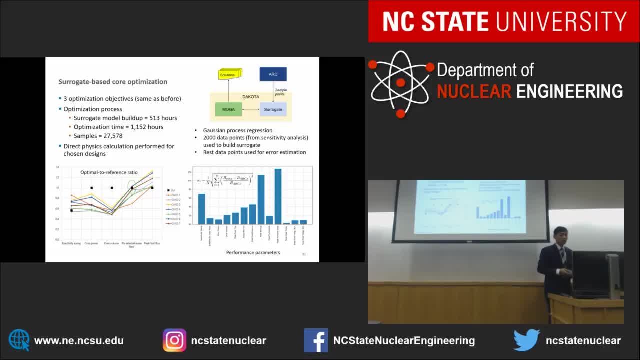 cases here. they should be below, but they're above. this is plutonium feed. they're above. this is plutonium feed. they're above. this is plutonium feed. they're higher than reference. so it they're higher than reference. so it they're higher than reference. so it means that your reference or your circuit, 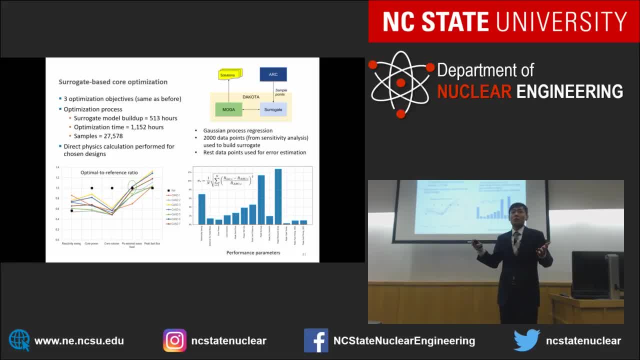 means that your reference or your circuit, means that your reference or your circuit model are not so accurate, which is model- are not so accurate, which is model are not so accurate, which is understandable, but we're right with understandable. but we're right with understandable, but we're right with they're buying us. it's the time, okay, we. 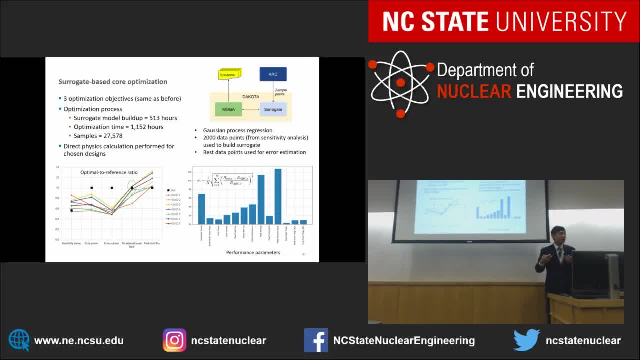 they're buying us. it's the time, okay. we they're buying us. it's the time, okay. we understand there. they won't be. act as understand there. they won't be. act as understand. there. they won't be. act as accurate as the direct physics. accurate as the direct physics. 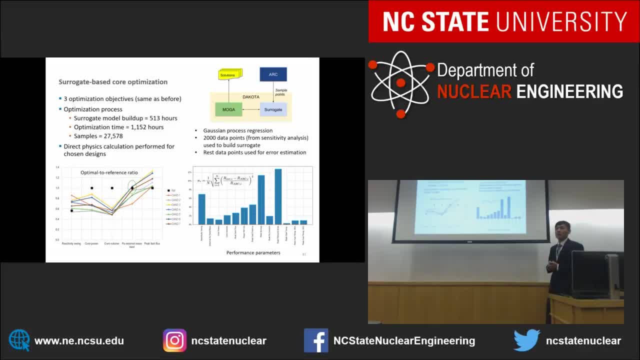 accurate as the direct physics calculation. next thing I want to say: see calculation. next thing I want to say: see calculation. next thing I want to say: see is it can we further improve? is it can we further improve? is it can we further improve effectiveness or reduce the? 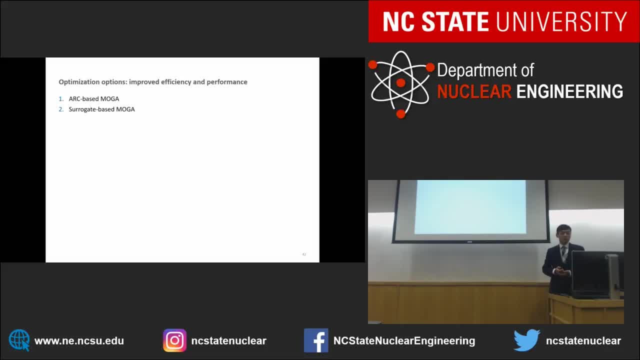 effectiveness, or reduce the effectiveness or reduce the computational time. so we tried this. so computational time, so we tried this. so computational time, so we tried this. so this is the first choice. second choice: this is the first choice. second choice: this is the first choice. second choice: all right. next thing I tried is: let's. 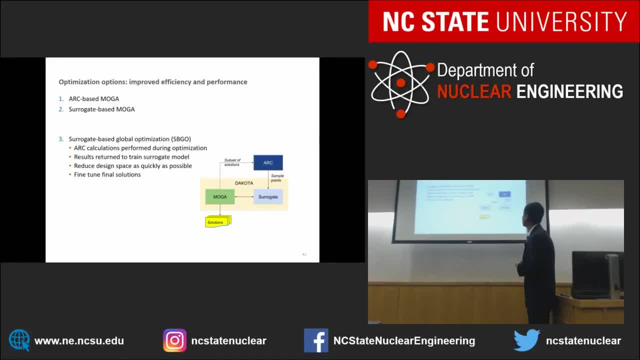 all right. next thing I tried is: let's all right. next thing I tried is let's combine the surrogate with the arc, combine the surrogate with the arc, combine the surrogate with the arc. calculation: so what we did is that we use calculation. so what we did is that we use 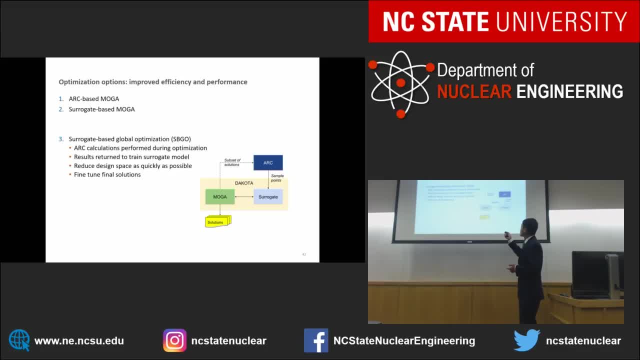 calculation. so what we did is that we use arc to generate a smaller sample of arc. to generate a smaller sample of arc. to generate a smaller sample of points to train the surrogate. smaller points to train the surrogate. smaller points to train the surrogate. smaller sample means the surrogate won't be as 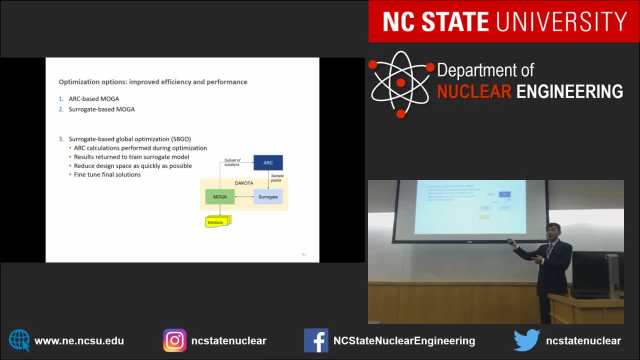 sample means the surrogate won't be as sample means the surrogate won't be as accurate as before, but that's okay. as accurate as before, but that's okay. as accurate as before. but that's okay. as long as it's in the ballpark it will. long as it's in the ballpark it will. 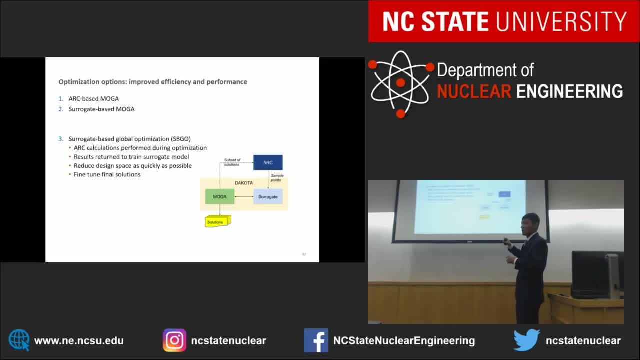 long as it's in the ballpark, it will help us. and then we'll use this circuit help us, and then we'll use this circuit help us, and then we'll use this circuit to opt to do the optimization, even to opt to do the optimization. even to opt to do the optimization, even though it's not as accurate, it helps to. 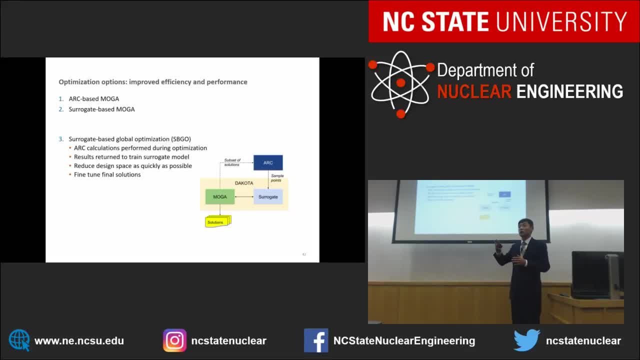 though it's not as accurate, it helps to- though it's not as accurate, it helps to reduce the design space as quickly as reduce the design space as quickly as reduce the design space as quickly as possible because I remember the 3d plot. possible because I remember the 3d plot. 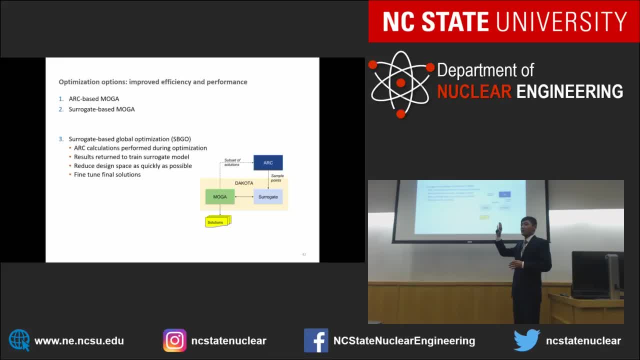 possible because I remember the 3d plot with the dots. a lot of the dots in the with the dots, a lot of the dots in the with the dots, a lot of the dots in the first few generations are really far. first few generations are really far. 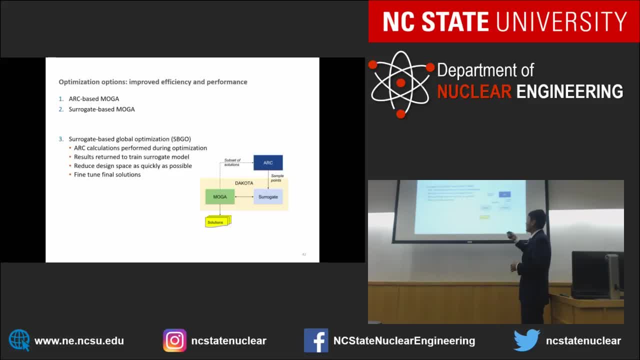 first few generations are really far away from Pareto front. I know that and I away from Pareto front, I know that and I away from Pareto front. I know that and I think we can use the surrogate model to think we can use the surrogate model to. 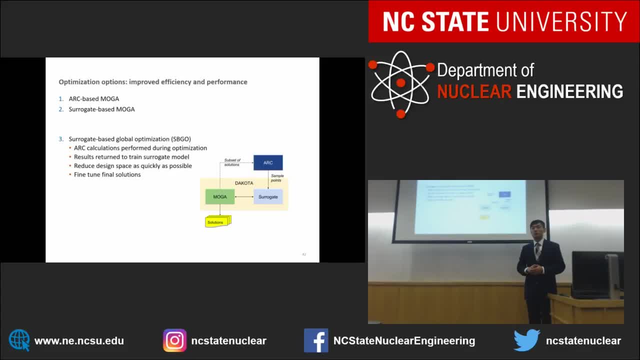 think we can use the surrogate model to just quickly get away from those dots. we just quickly get away from those dots. we just quickly get away from those dots. we move quickly to the Pareto front and move quickly to the Pareto front and move quickly to the Pareto front and then in the next, after few relations, I 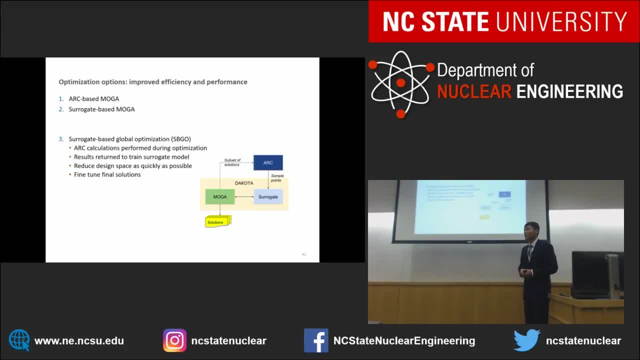 then in the next, after few relations, I then in the next, after few relations, I use arc to generate another set of use arc to generate another set of use arc to generate another set of sample. I use that to improve my circuit sample. I use that to improve my circuit. 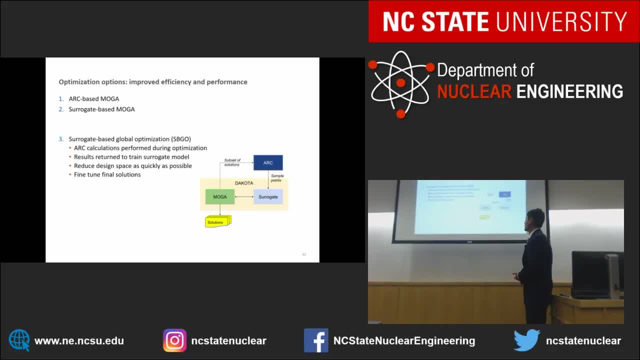 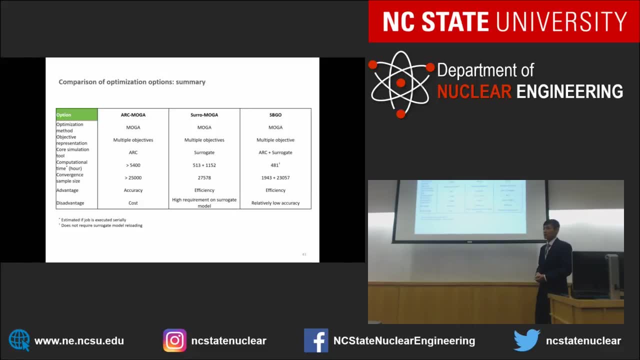 sample. I use that to improve my circuit model, so that to prove the, the, the model, so that to prove the, the, the model, so that to prove the, the, the computational efficiency. so I compare computational efficiency, so I compare computational efficiency, so I compare these three options here. apparently the 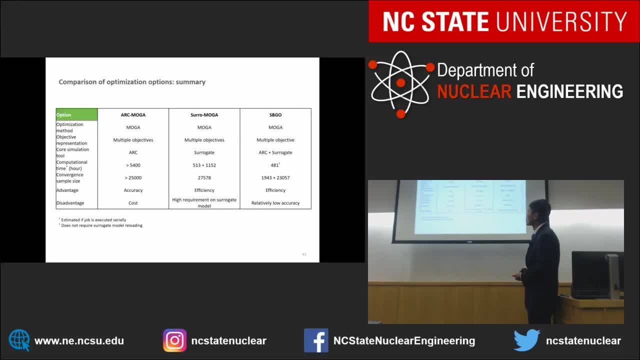 these three options here, apparently, the these three options. here, apparently, the arc based optimization is more time. arc based optimization is more time. arc based optimization is more time consuming most content consuming, but consuming most content consuming but consuming most content consuming. but there it is most accuracy. the second one: 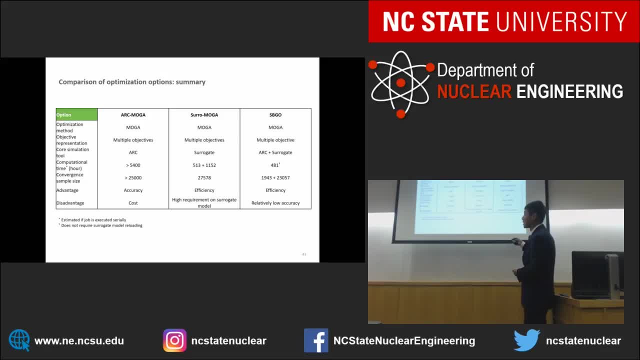 there it is most accuracy. the second one: there it is most accuracy. the second one is in the middle, but then really, if you is in the middle, but then really, if you is in the middle, but then really, if you look at this, the third option with a: 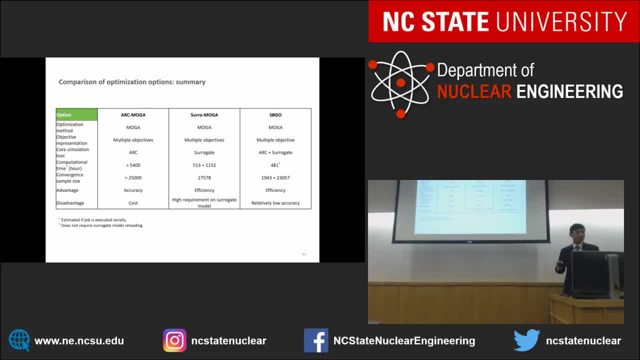 look at this, the third option, with a. look at this, the third option, with a surrogate plus the arc calculation. the surrogate plus the arc calculation, the surrogate plus the arc calculation: the computational time is really really computational time is really really computational time is really really short, and what part of the reason is? 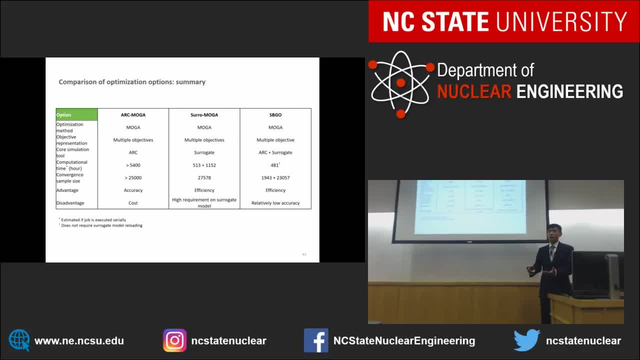 short and what part of the reason is short and what part of the reason is? because now everything is under the hood. because now everything is under the hood, because now everything is under the hood of Dakota. so you, there's data writing of Dakota. so you, there's data writing. 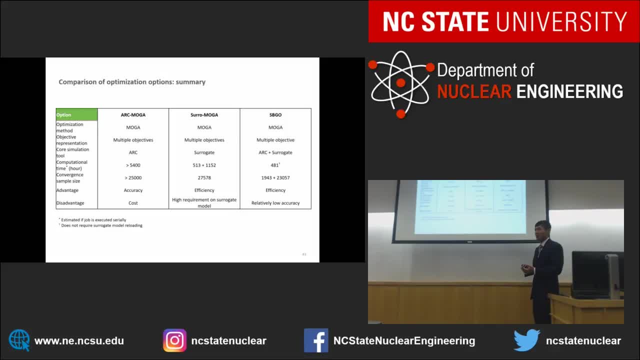 of Dakota. so you, there's data writing and the reading is less time it takes, and the reading is less time it takes, and the reading is less time it takes less time, but still this sees a lot of less time, but still this sees a lot of less time, but still this sees a lot of improvement on the, on the, on the. 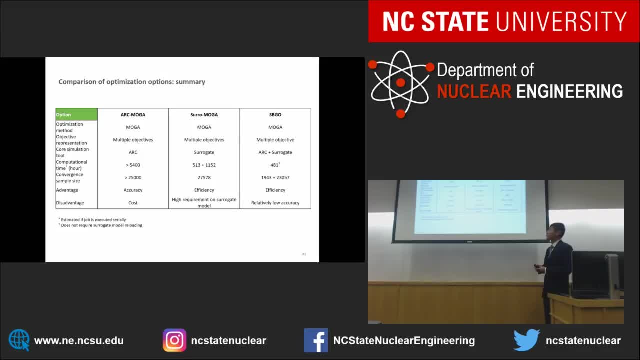 improvement on the, on the, on the improvement on the, on the, on the efficiency. but the cost is of course it efficiency. but the cost is of course it efficiency. but the cost is of course it has. it has a relatively low accuracy, so has it has a relatively low accuracy, so 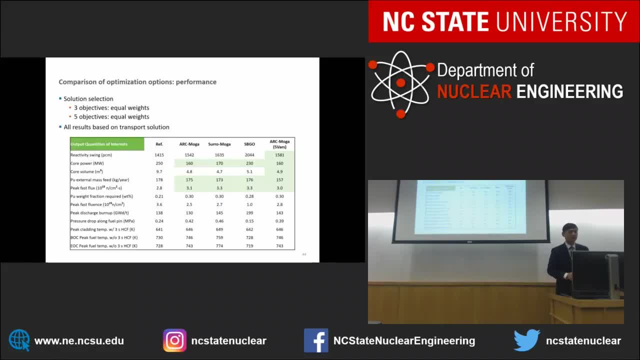 has. it has a relatively low accuracy. so you have to really make a judgment, when you have to really make a judgment, when you have to really make a judgment, when you come to practicality, and this is the you come to practicality and this is the you come to practicality, and this is the comparison of the performance of the. 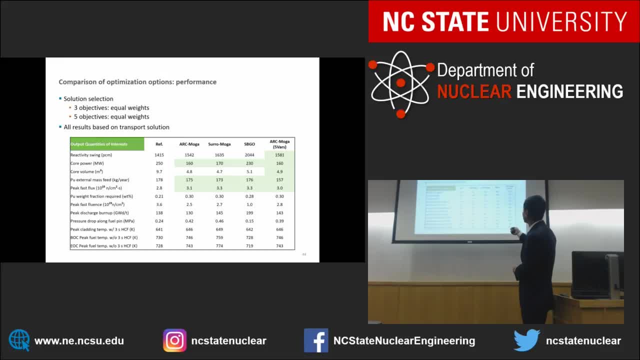 comparison of the performance, of the comparison of the performance of the reference listed here: first option. reference listed here: first option. reference listed here: first option, second, third, and if you look at those second, third, and if you look at those second, third, and if you look at those, the third option definitely doesn't. 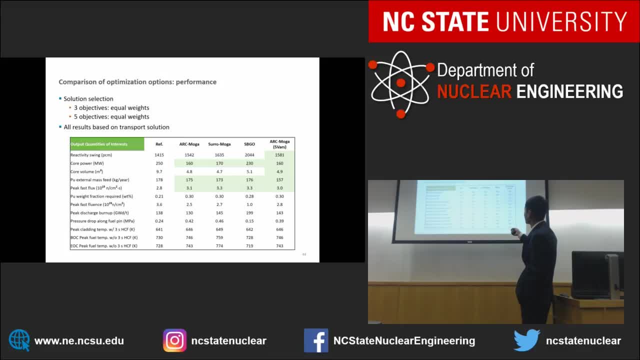 the third option definitely doesn't. the third option definitely doesn't outperform the first two. for example, the outperform the first two. for example, the outperform the first two. for example, the core power is much higher and petonia, core power is much higher and petonia. 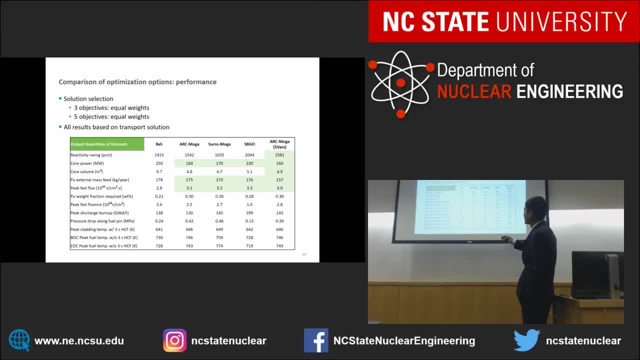 core power is much higher and petonia feed is much higher. slightly improve on feed is much higher. slightly improve on feed is much higher. slightly improve on the peak fast flux, which is understandable, the peak fast flux, which is understandable, the peak fast flux, which is understandable. but if you compare this with a reference, 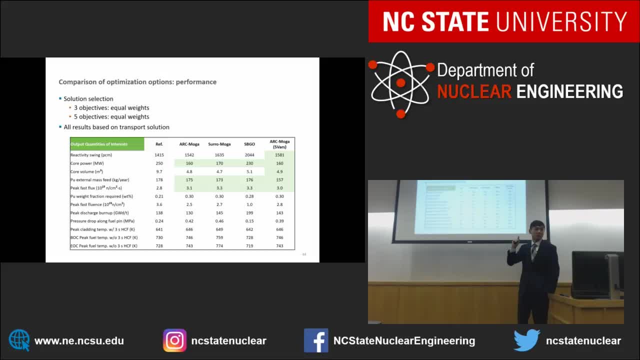 but if you compare this with a reference, but if you compare this with a reference, still much, much better. you all metrics still much, much better. you all metrics still much, much better. you all metrics. okay, the next thing I want us, I want to. okay, the next thing I want us, I want to. 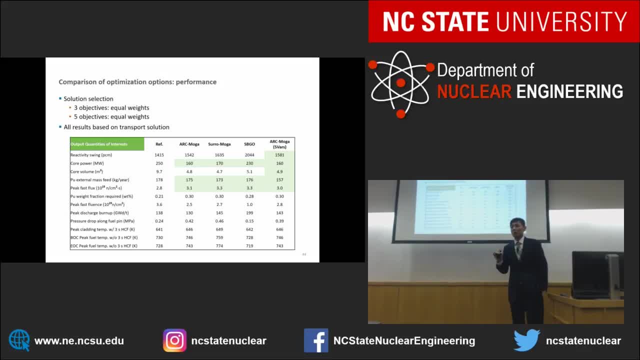 okay, the next thing I want us, I want to check is at the beginning. we remove two. check is at the beginning. we remove two, check is at the beginning. we remove two parameters design objectives, which are parameters, design objectives, which are parameters, design objectives, which are reactivity, swing and core volume. now, 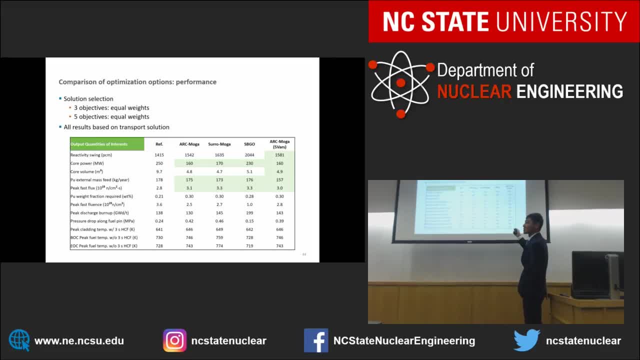 reactivity swing and core volume now. reactivity swing and core volume: now. let's put it back. we run arc based the. let's put it back. we run arc based the. let's put it back. we run arc based the most expensive optimization. let's see how. 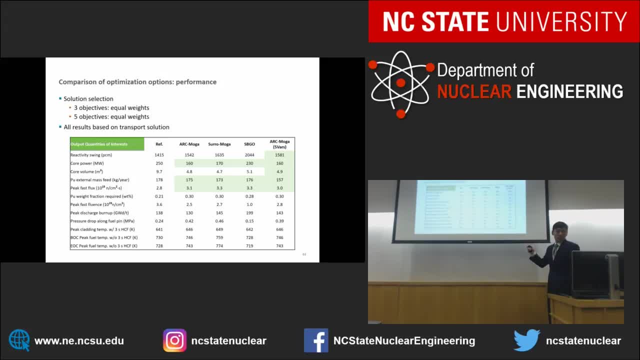 most expensive optimization. let's see how most expensive optimization. let's see how how it works. these are the results in how it works. these are the results in how it works. these are the results. in fact is to compare this column and the fact is to compare this column and the 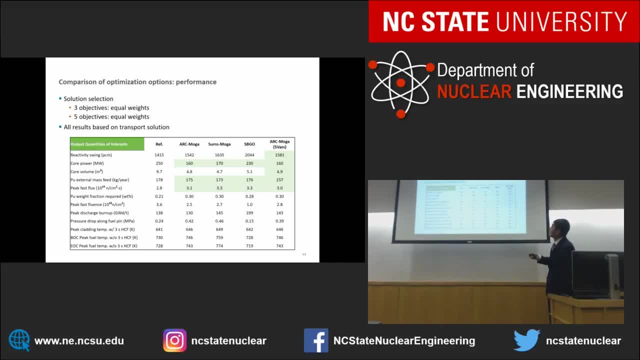 fact is to compare this column and the three object of our column. well, this one three object of our column, well, this one three object of our column, well, this one doesn't really look better than than doesn't really look better than than. doesn't really look better than than the first one. okay, 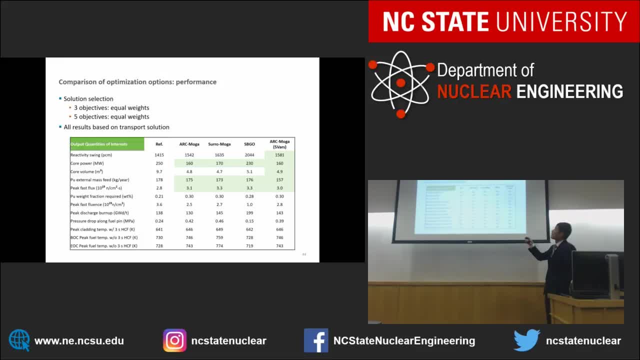 the first one. okay, the first one. okay, direct is sweet erectivity swings. higher direct is sweet erectivity swings. higher direct is sweet erectity swings. higher at the core volume, okay so, which at the core volume. okay so, which at the core volume. okay so, which probably is the indication that we made. 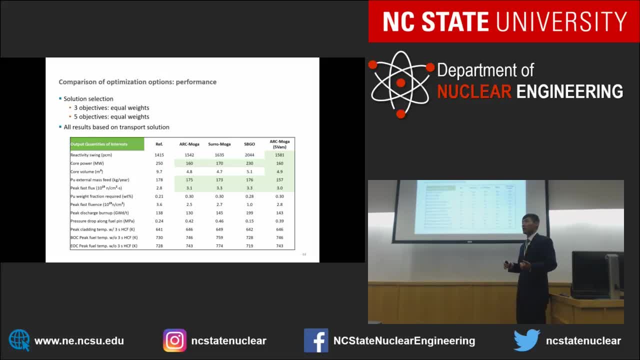 probably is the indication that we made. probably is the indication that we made a good choice at the beginning of a good choice at the beginning of a good choice at the beginning of removing those two, because those two are removing those two, because those two are removing those two, because those two are really strongly correlated with other. 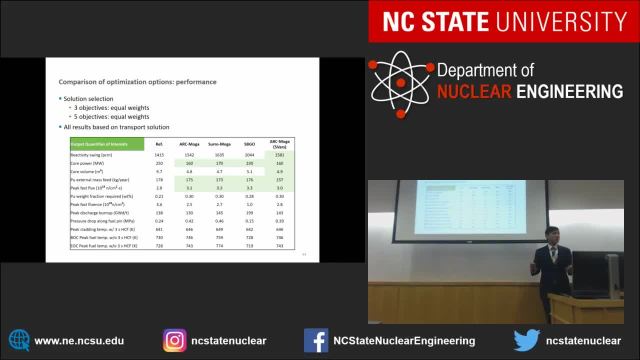 really strongly correlated with other, really strongly correlated with other three. you don't really need to consider three. you don't really need to consider three. you don't really need to consider them in the optimization. so that's how them in the optimization, so that's how them in the optimization, so that's how the sensitivity analysis can be really. 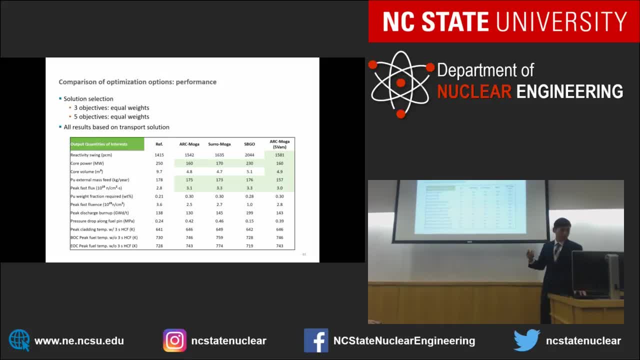 the sensitivity analysis can be really the sensitivity analysis can be really useful to simplify the optimization useful, to simplify the optimization useful, to simplify the optimization problem. and this is just summarize problem and this is just summarize problem and this is just summarize. summarize the performance comparison, the summarize the performance comparison, the. 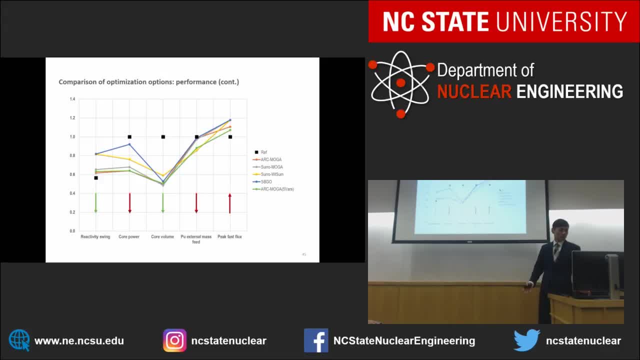 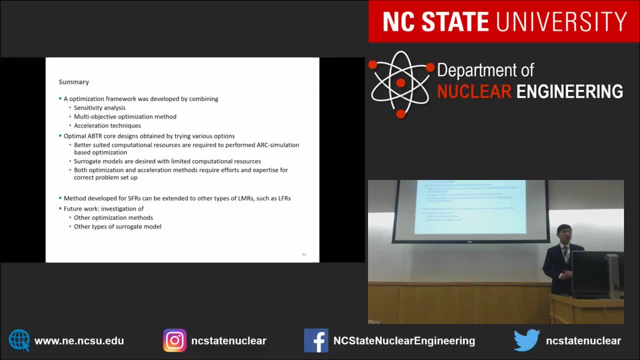 summarize the performance comparison: the same plot, okay, but they all satisfy the same plot. okay, but they all satisfy the same plot. okay, but they all satisfy the design objectives. so the second half the design objectives, so the second half the design objectives, so the second half the talk really shows you a framework for 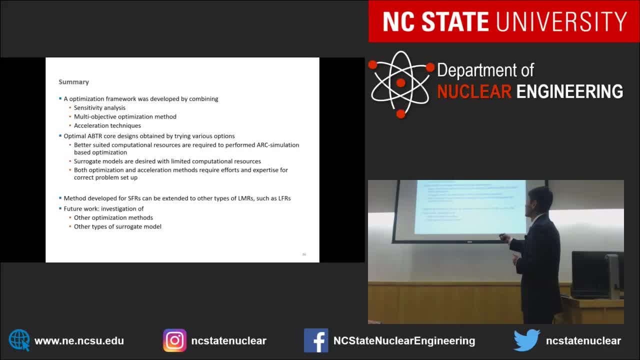 talk really shows you a framework for talk, really shows you a framework for optimization for the fast reactors. we optimization for the fast reactors, we optimization for the fast reactors. we combine sensitivity analysis with. combine sensitivity analysis with. combine sensitivity analysis with multi-active objective optimization. multi-active objective optimization. 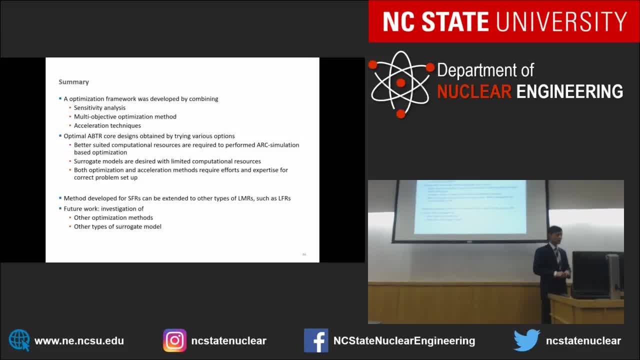 multi-active objective optimization method, with some acceleration method, with some acceleration method, with some acceleration technique, technique, technique based on the circuit models. it does based on the circuit models. it does based on the circuit models. it does require a lot of effort to understand, require a lot of effort to understand. 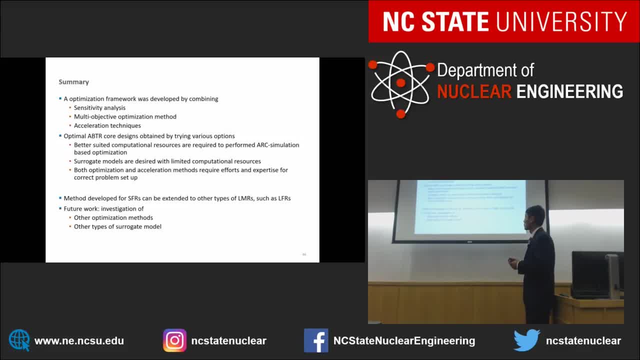 require a lot of effort to understand how different codes and circuit model, how different codes and circuit model, how different codes and circuit model works. it requires a lot of expertise. if works, it requires a lot of expertise. if works, it requires a lot of expertise. if you have the luxury of the. 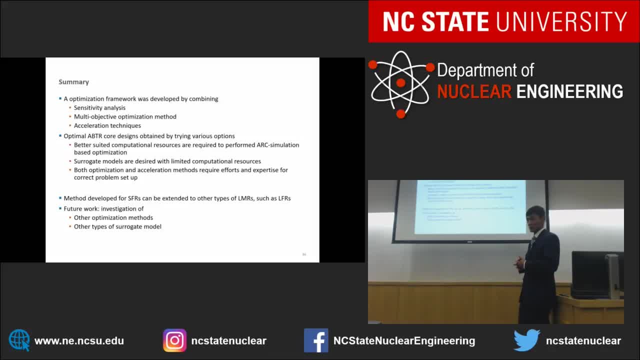 you have the luxury of the. you have the luxury of the computational resource. then go with the computational resource. then go with the computational resource. then go with the physics-based calculation if you want to physics-based calculation, if you want to physics-based calculation, if you want to save time, circuit model is probably your. 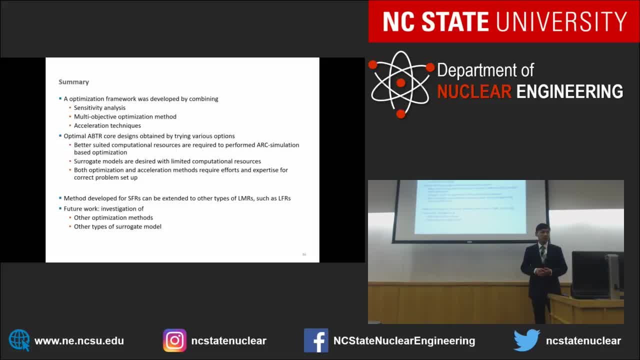 save time circuit model is probably your save time circuit model is probably your choice. we plan to extend this method choice. we plan to extend this method choice. we plan to extend this method for other retro types and we want to for other retro types and we want to. 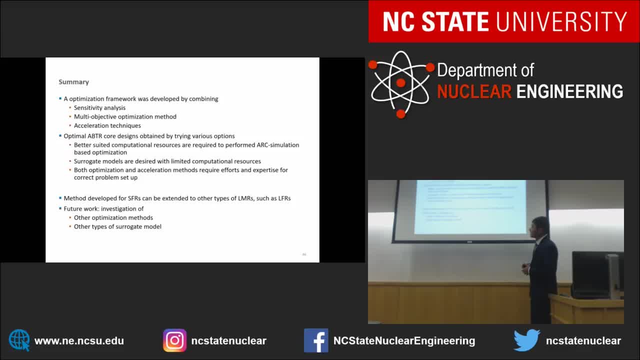 for other retro types and we want to continue looking to other optimization, continue looking to other optimization, continue looking to other optimization methods and other types of circuit methods and other types of circuit methods and other types of circuit models. with that I conclude my models. with that I conclude my. 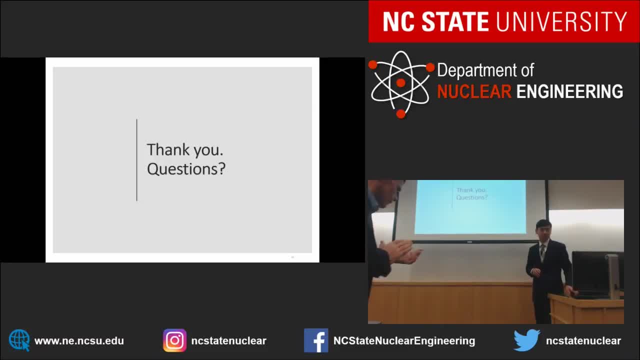 models. with that I conclude my presentation. I'll take questions. if you presentation, I'll take questions. if you presentation, I'll take questions. if you have, thank you have, thank you have, thank you. did you ever estimate how much extra? did you ever estimate how much extra? did you ever estimate how much extra time it would take to do the refueling? 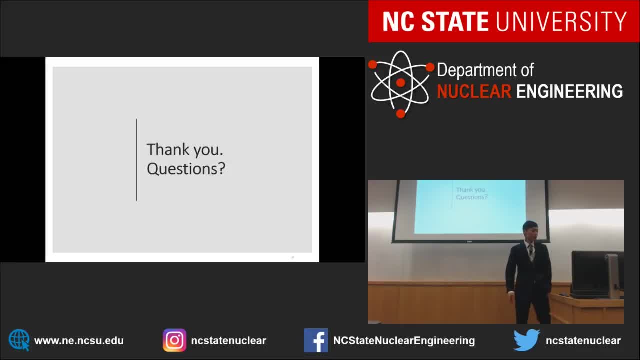 time it would take to do the refueling. Yeah, I didn't do a direct comparison, but I realized it could be a problem because you will have much more fuel assemblies. It requires a lot more shuffling, time and space. So actually we did. let me see. 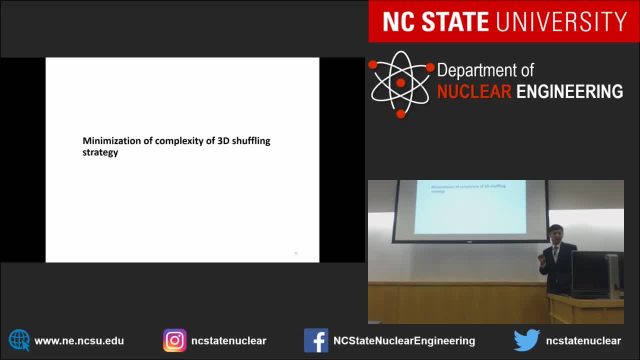 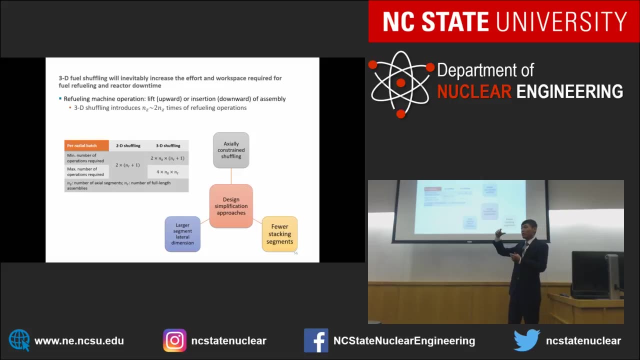 Some study to maximize the complexity of the 3d shuffling. few things we tried is We've. we tried axially constrained shuffling, Which means you take one assembly with four segments away, Then you put them all at the same radio location instead of putting them in different radio location. 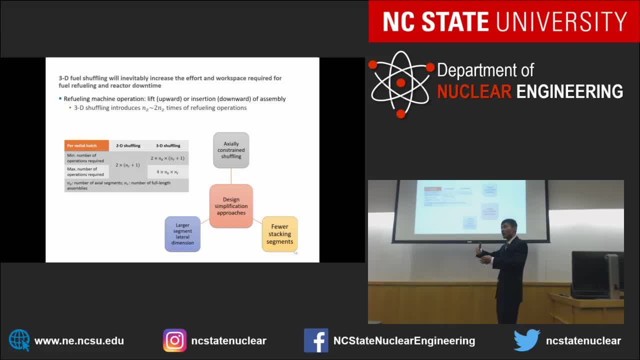 But in different active order. that could simplify your shuffling skin. then we can with Consider fewer stacking segments. We reduce from four to three to even two right, And then we consider a larger segment, lateral dimension, so you can have a fewer fuel assemblies with the same core volume. 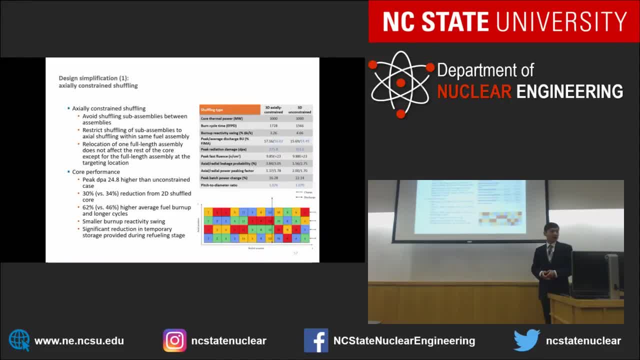 So I can show you something very quickly: when you act axially, constrained the shuffling, Okay. so all the assembly, you see all these numbers are aligned because they are in the same location, But different axial or elevation. by doing this I'm not losing too much. This is my constrained shuffling and this is my 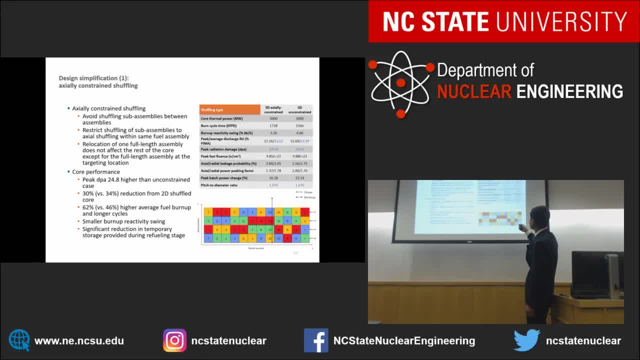 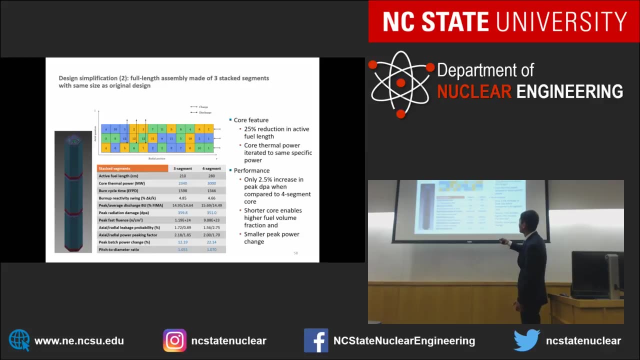 free Shuffling 3d. you see only 25 Dpa increase, which is not how a lot, but it saves you a lot of time and space in term of the shuffling and I can even reduce to three segments and You know I see less than 10. 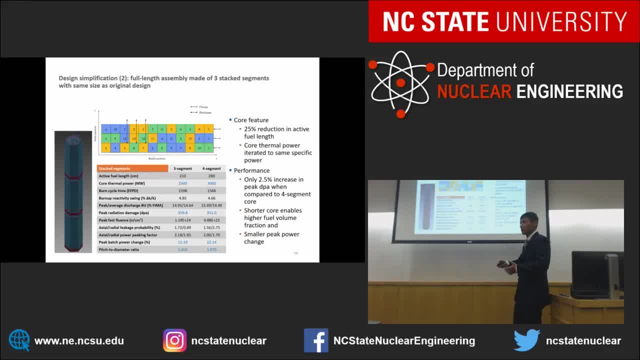 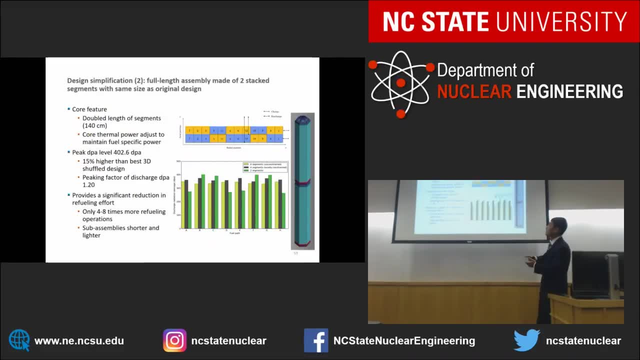 So you reduce 25% of a few assemblies but you lose only like a 10 DPA DPA in terms of radiation damage and even with two- with two is not Really performing really well, but we also try that. Yes, we install control rods for these 3d assemblies. 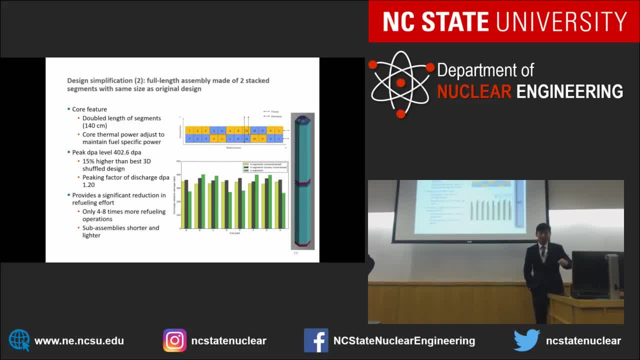 because when we are having different power factors we may need to control the control rods at different positions. we change the positions of these control rods, we burn up for these three independent assemblies or the different 3d, and the control rod history can be controlled before the cycle. 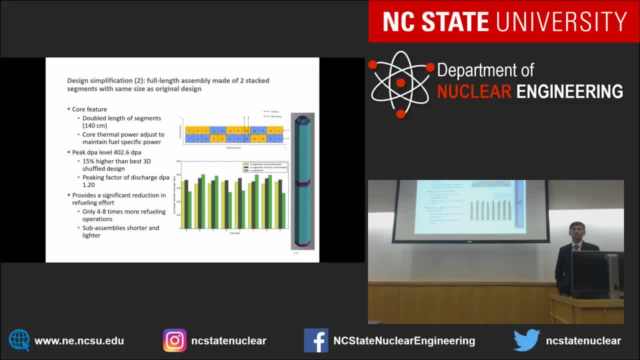 So after one cycle, how do you make sure these burn up in different segments or be ready for the next cycle? Right, right, Okay. First of all, the calculation down here is called equilibrium cycle. It means that you have run in many, many cycles and the core 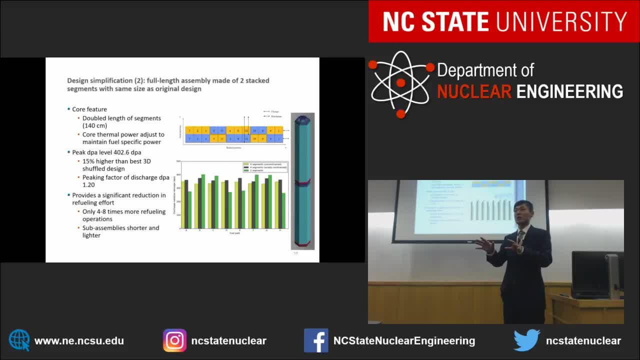 Performance does not change over cycle, right. So we know exactly where the radial and axial picking will happen, just as normal 2d shuffle case. right so? but in the transition, yes, that's a challenge, because from Non 3d shuffle to 3d shuffle the transition is is kind of difficult. 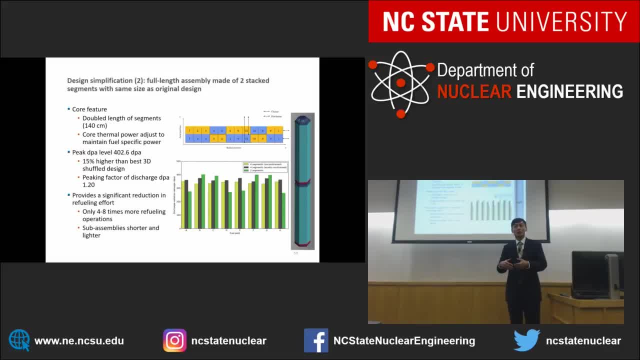 But once you establish the equilibrium cycle, equilibrium core, the control is. it's just the same. Thank you, very much, Thank you.